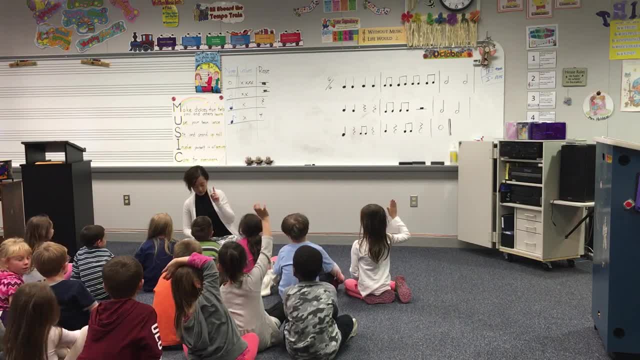 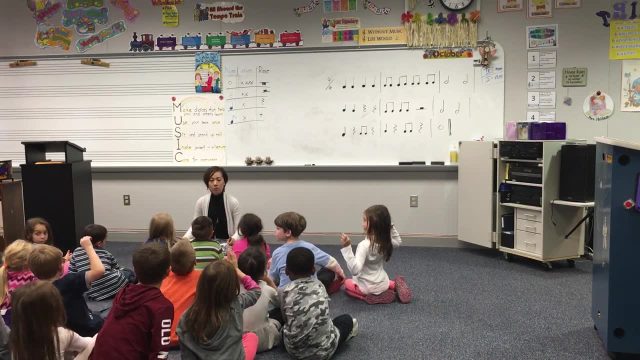 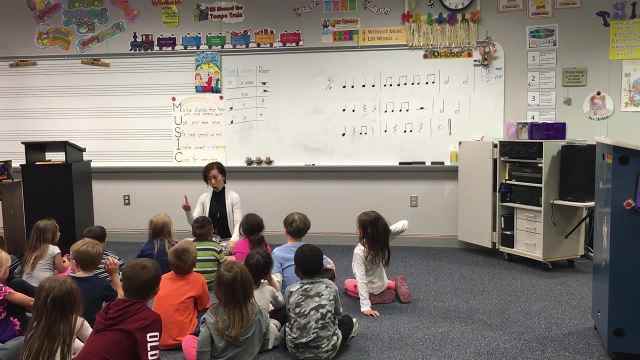 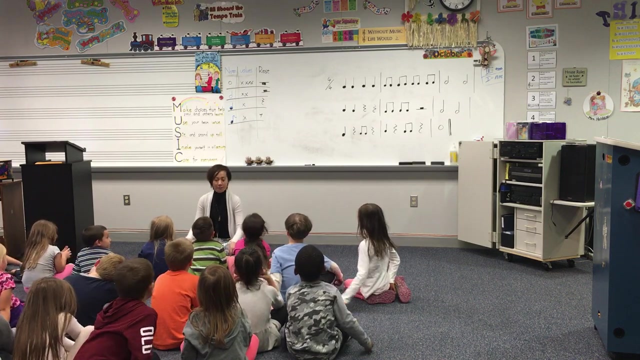 Lemon, Now listen. I love you Now hold Our bathroom. rule is you go to the bathroom before you come. Thank you Hold. Oh, wow, Hands down. Now listen. When I call your name, what do I want to say? 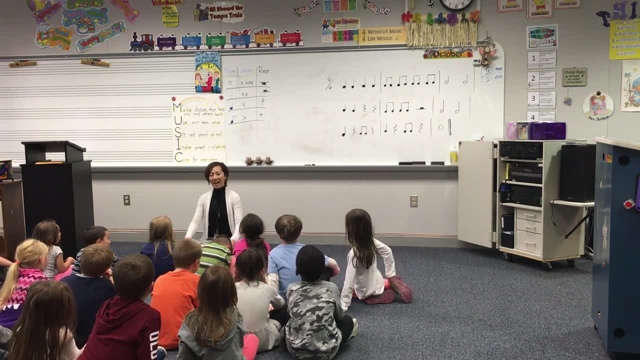 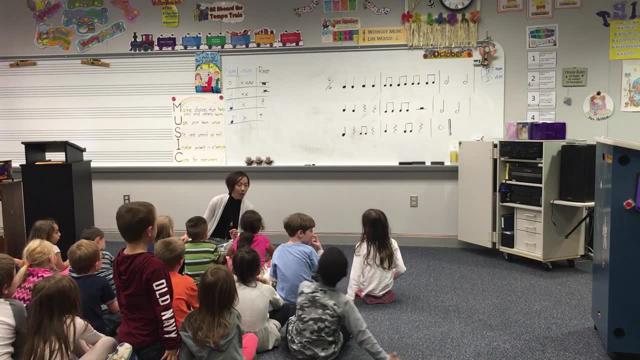 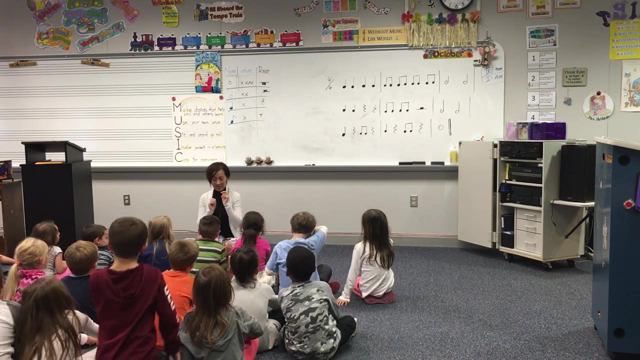 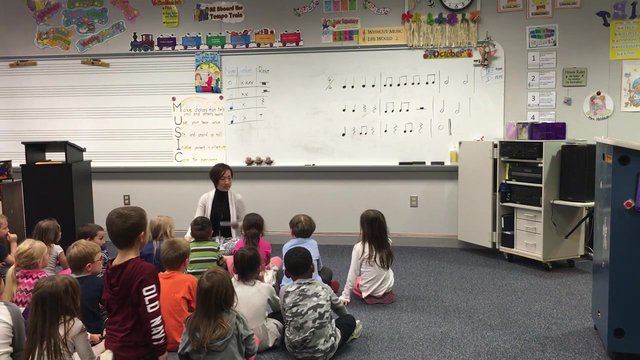 Fantastic, Fantastic, dream Banana Or what is your favorite word, Water, Watermelon. And then she will say: Watermelon. Okay, great, Let's try that. Let's start Shh Cassidy: Watermelon, Watermelon. 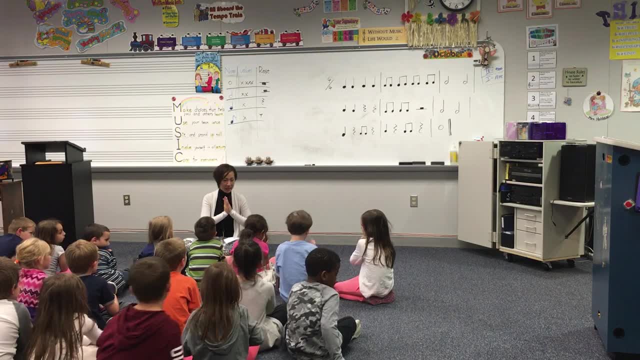 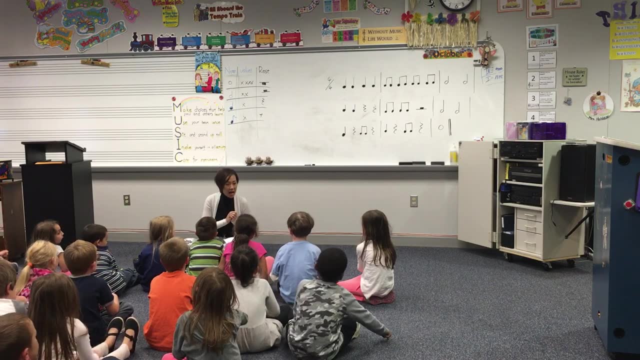 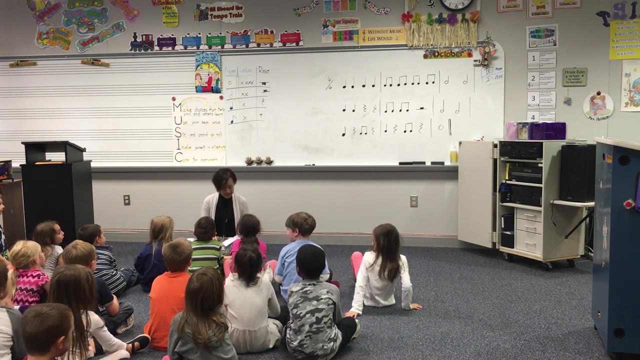 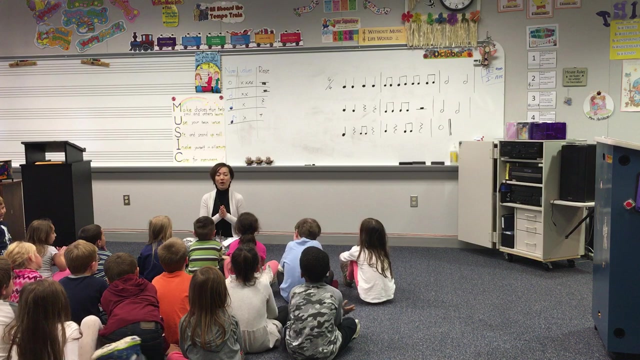 One, two ready go My phone, Apple, Apple. One, two ready go, Apple, Apple, Apple. Let's try it. Lemon: One, two pretty. Oh, that's that, Let's do that. 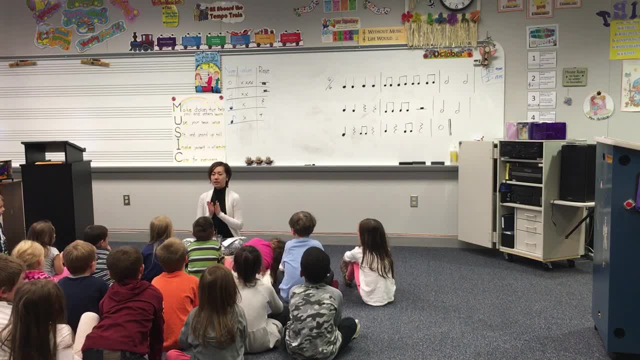 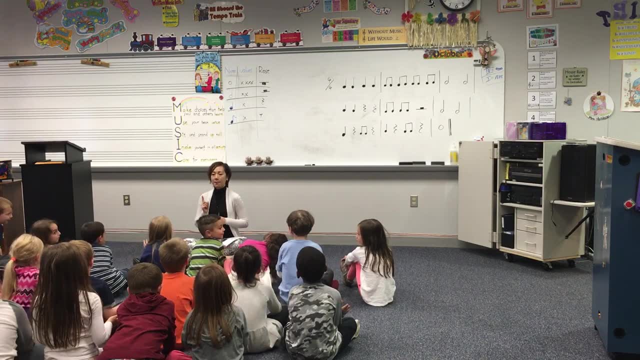 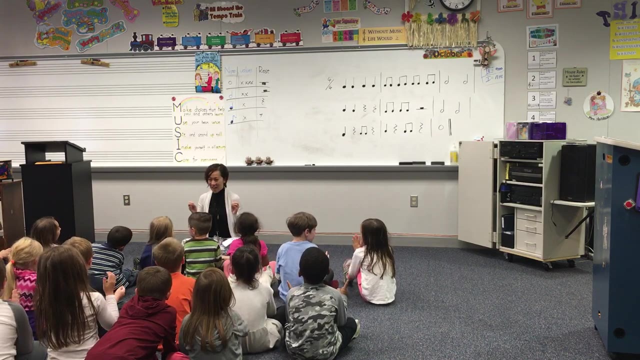 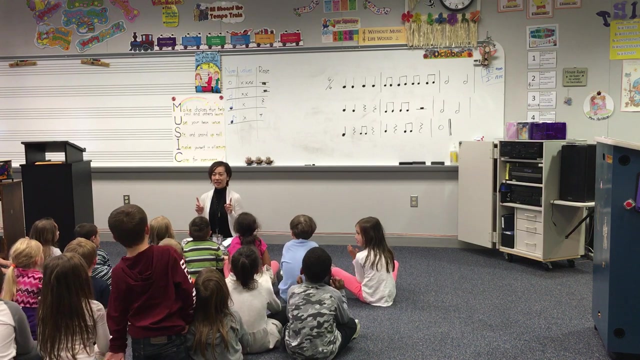 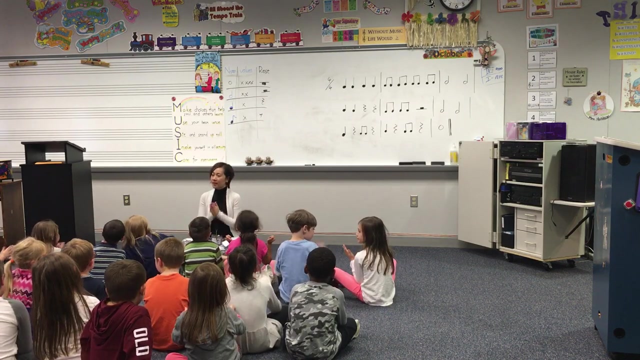 Let's all try it, Apple. And then clap your hands: One, two, ready, go Apple, Apple, Apple, Apple, Apple, Apple. How about banana? One, two and three, four, Banana Banana. 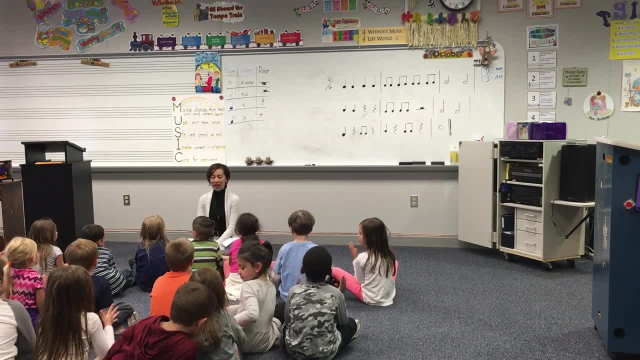 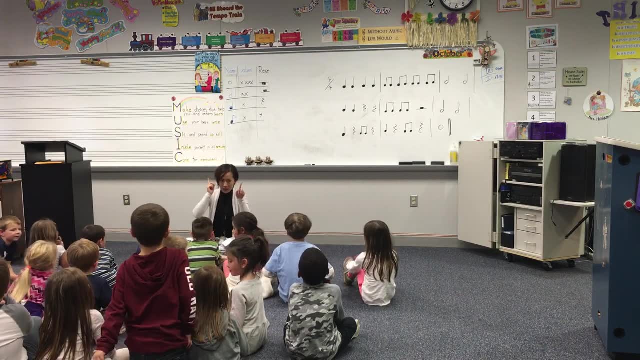 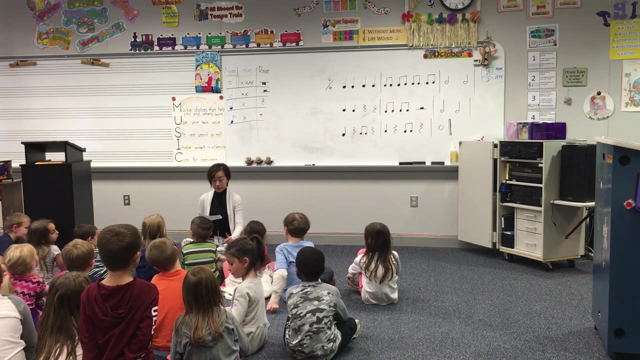 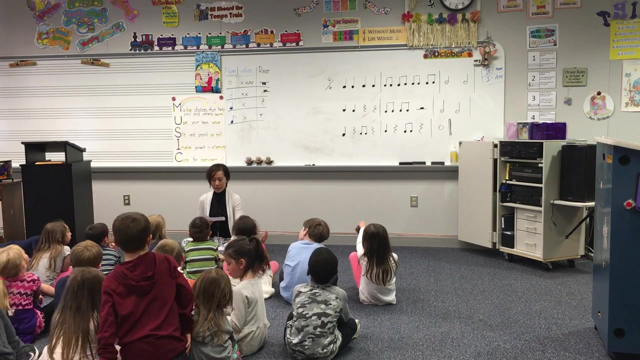 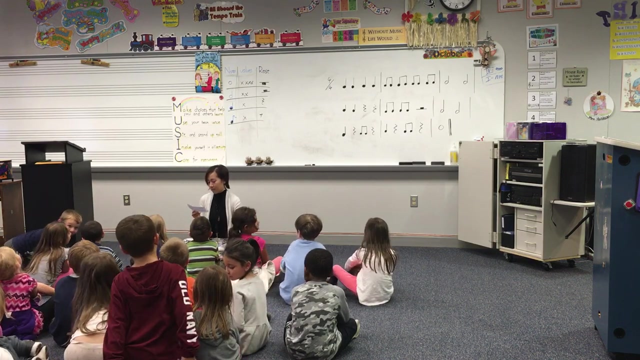 Banana. Let's choose apple or banana. Okay, think about your choice. Think about your choice. No, whale Apple. Clap, clap, clap, Clap. three times Ready. Good, Two, three Good, Like this one. 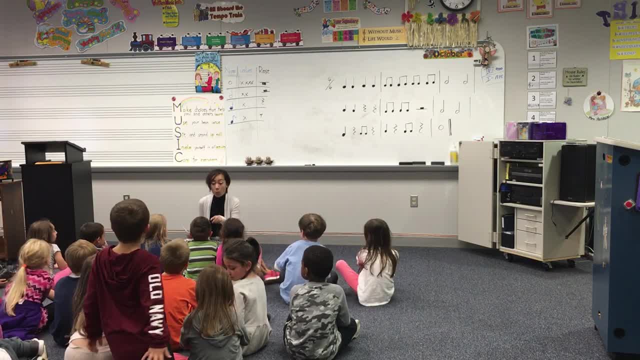 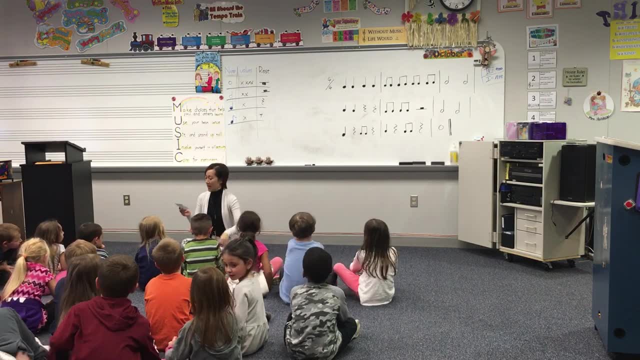 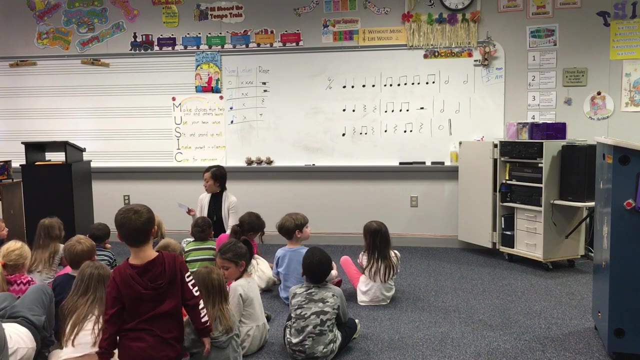 Anthony, Apple, Apple, Clap, clap clap. Remember Clap clap clap, Let's see. Apple Good, Joseph Good, Clap three times. Banana, Banana, Banana Good, Gregory Banana. 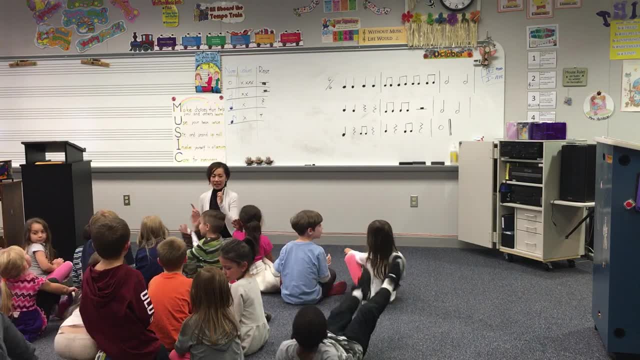 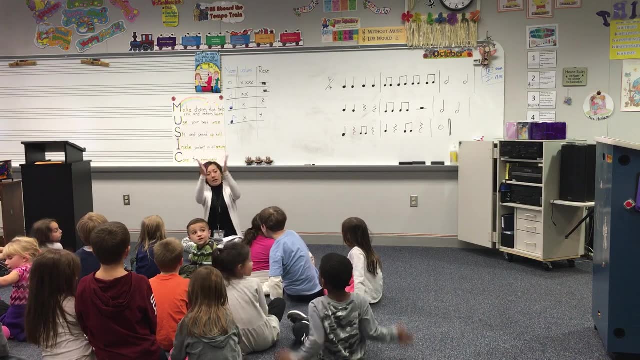 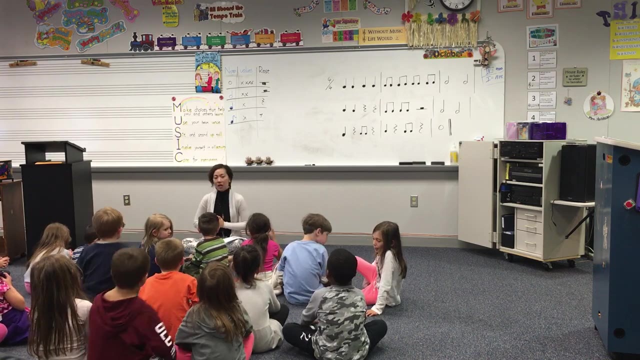 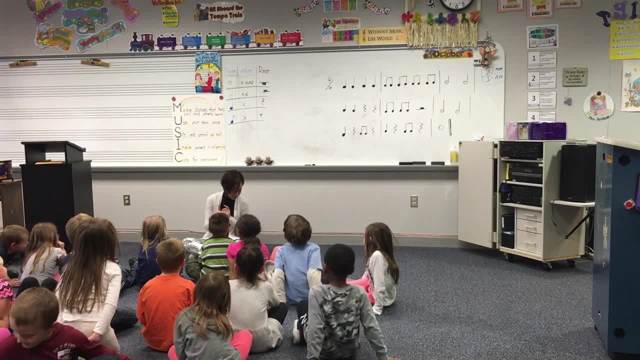 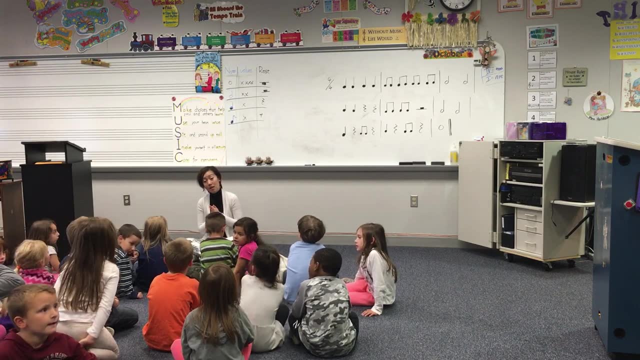 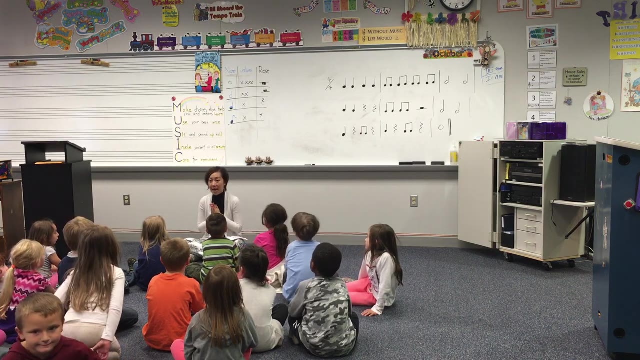 Analog Three: Three eleven Red Red Red. What's my name? breaths Work Good, Oh, ready, Oh. Red, Red, Red Red. I like red Red, vision Red Red. 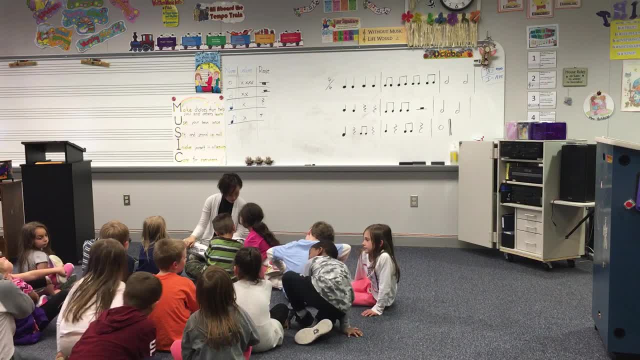 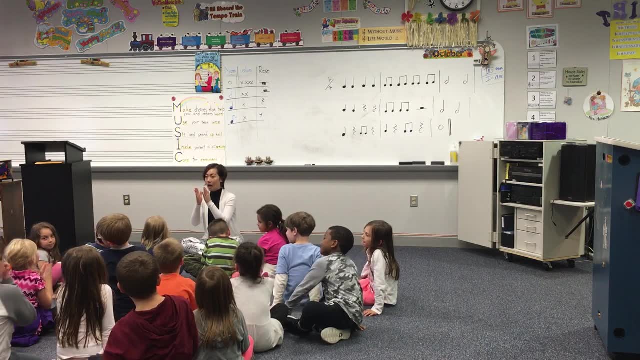 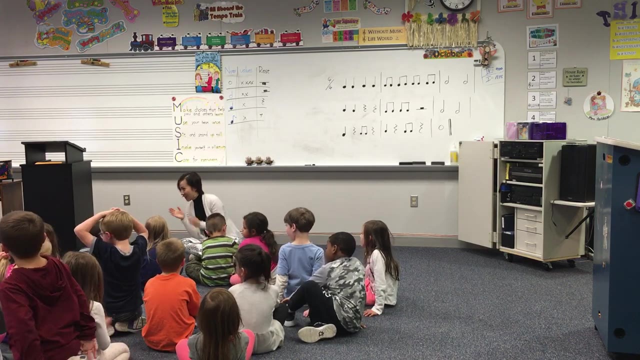 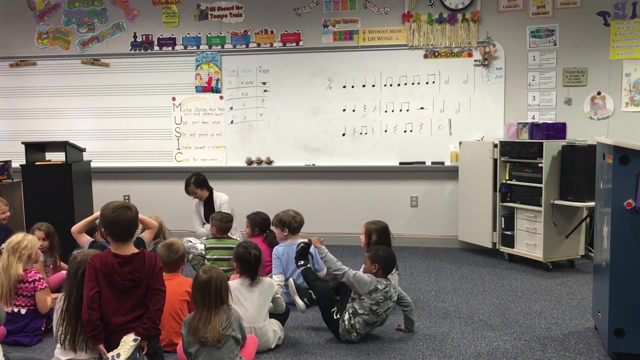 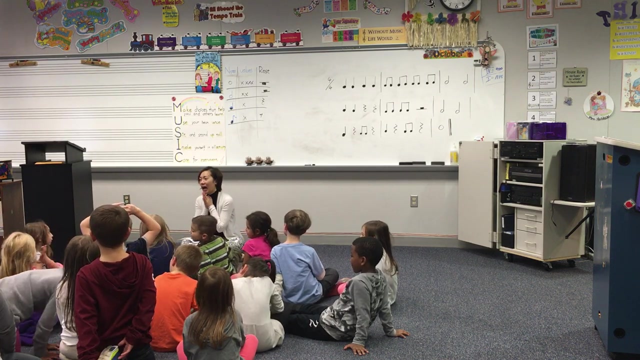 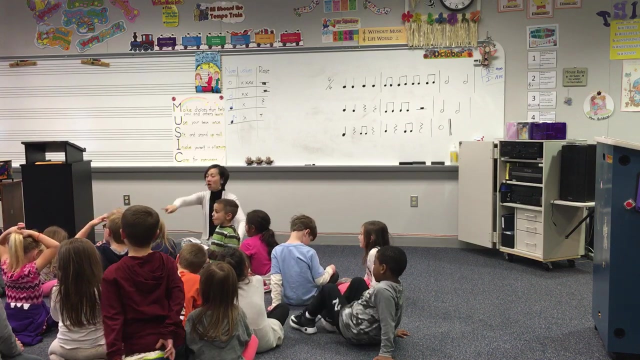 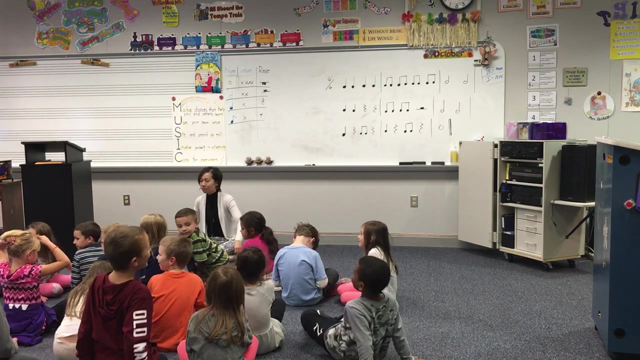 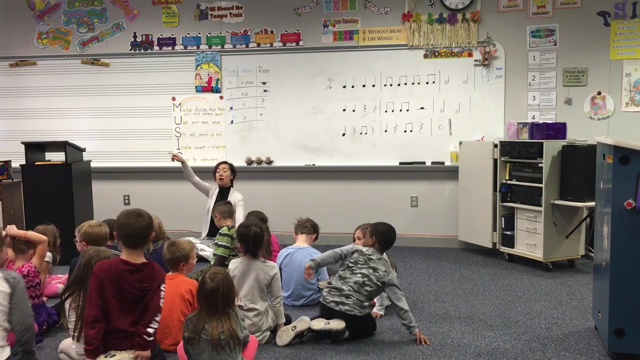 Good job, Really good job. Good job, Good job. I like that one. Yeah, I will say this: Logan Water Mountain- Good you too. Switch spot, Trevor. Switch your spot with Logan. Thank you The third row. are you ready? 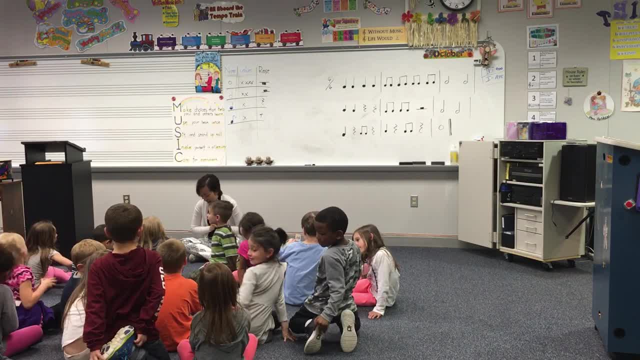 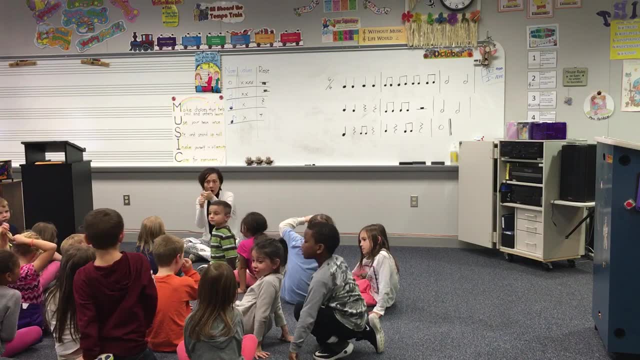 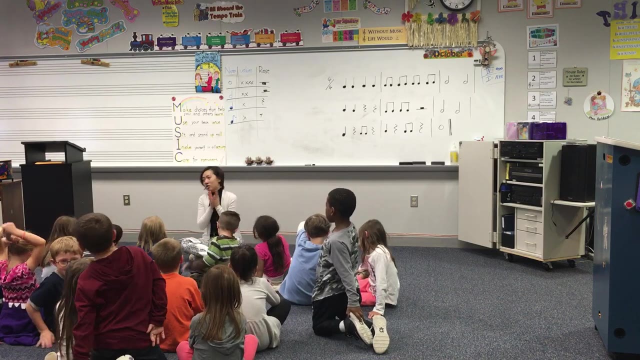 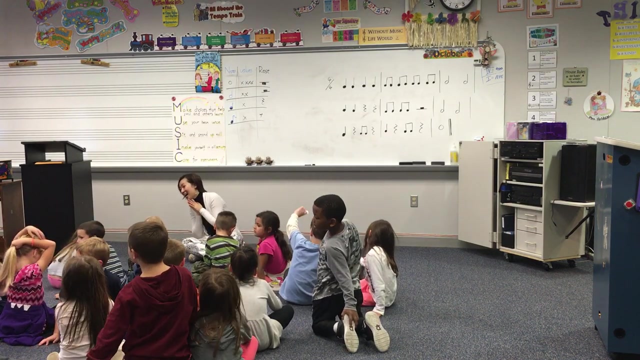 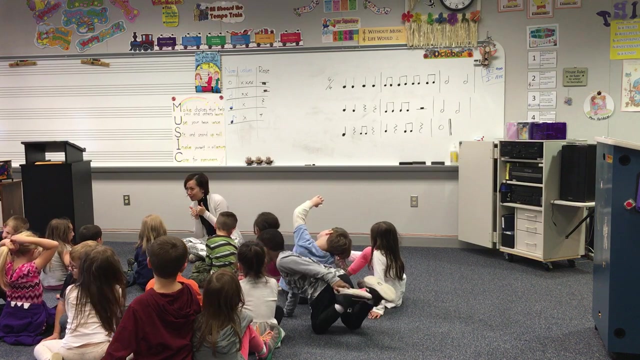 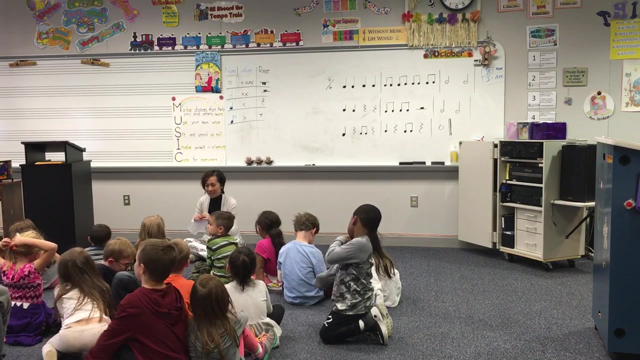 Blackberry- Good, I like that one, Okay. Fruit Strawberry- Nice, I like that one, Yeah. Strawberries- Good. Eli- Great, Oh good. I love all the three challenges. Let's work. One, two, step, one. 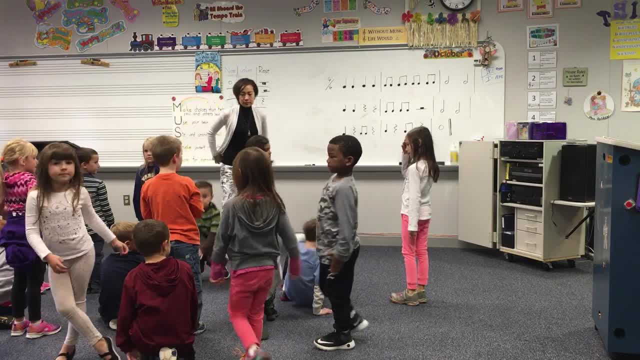 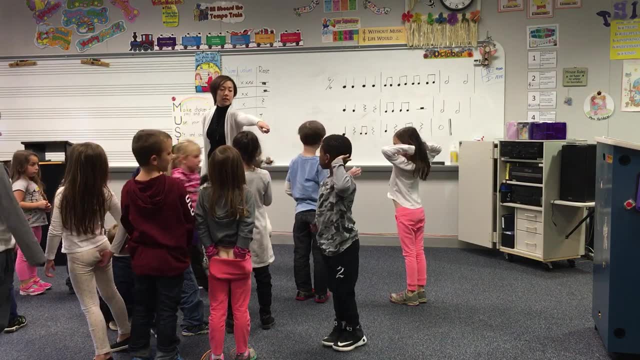 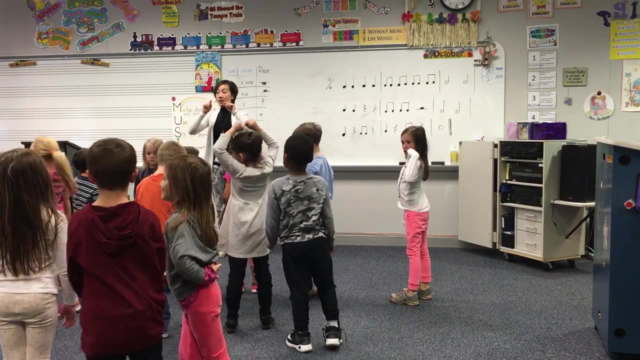 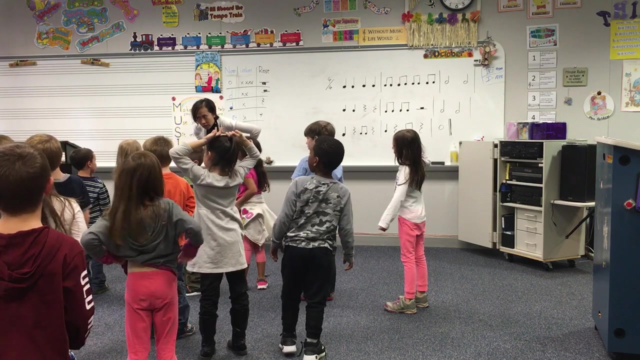 Logan, try one, I'm gonna go with you, Alright, Oh yeah, yeah, yeah, Maybe I'll try it over there. Third row: third row: one step back. Second row: one step back. Um, Seriously. 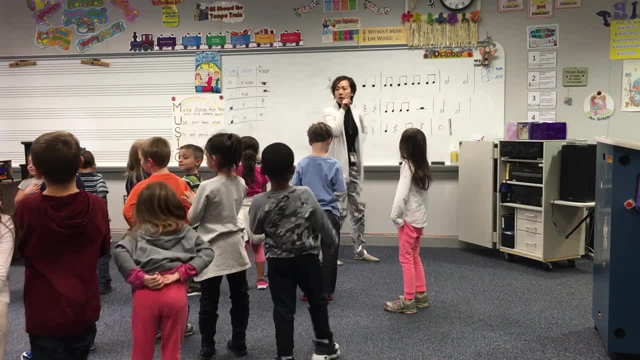 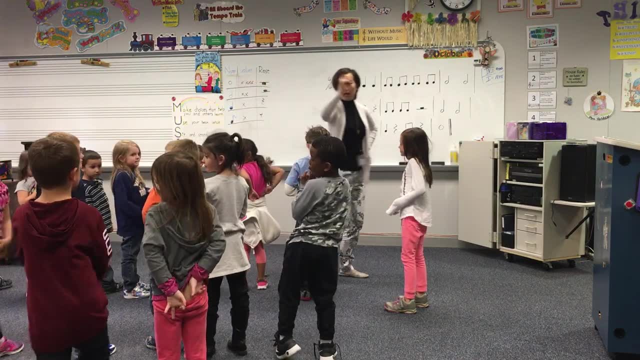 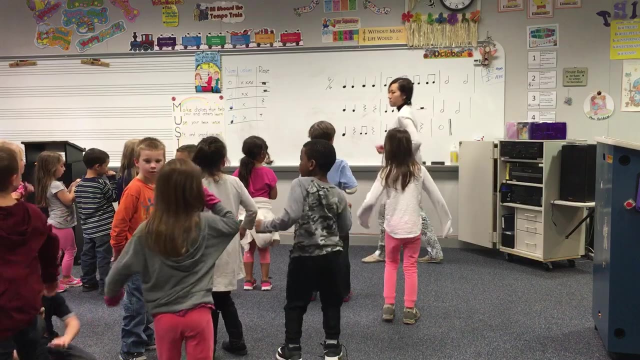 Shh, Last word now. Second row, second row, second row. where's my second row? Third row, where's third row? Ah, Third row. Okay, Oh, zombie style. Uh-oh, zombie style. I have a zombie walker job. 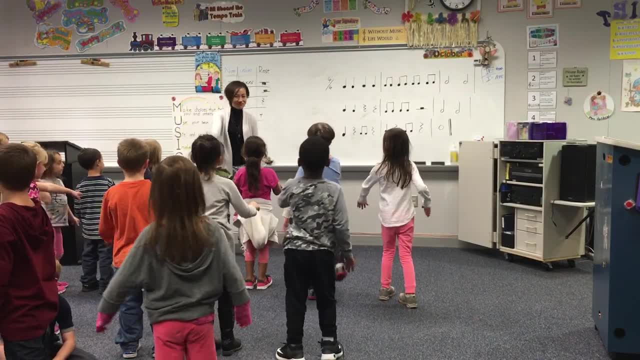 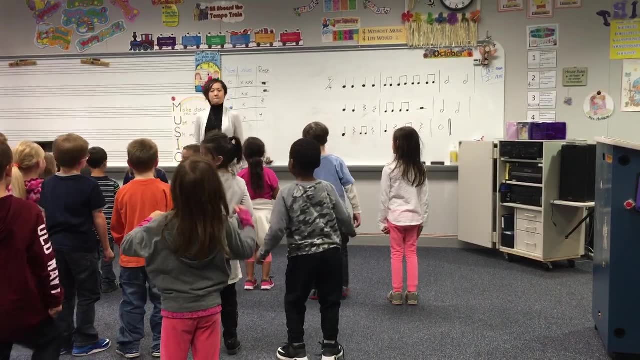 A zombie walker. A zombie walker Shh. Watch out for walkers coming at you down the street. They're moving slow because they're dragging all their meat. They're moving slow because they're dragging all their meat, But don't be fooled, they're really not that cool. 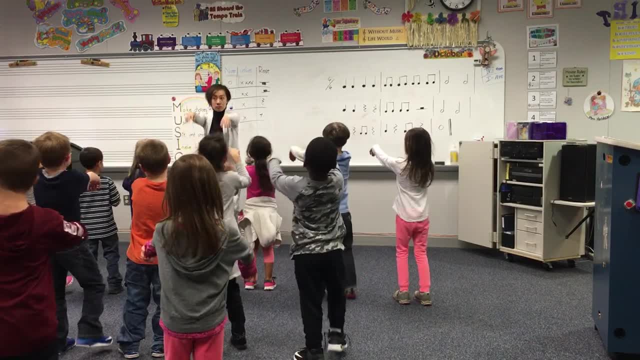 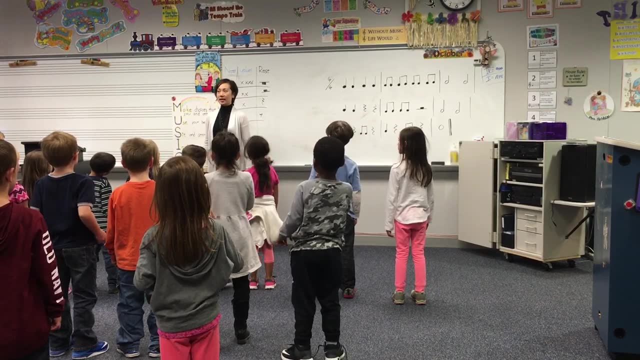 But don't be fooled, they're really not that cool. They only want to eat, eat, eat. They only want to eat, eat, eat. They want some brain snacks. They want some ooey dooey эти prossimo konny upgraded brain snacks. 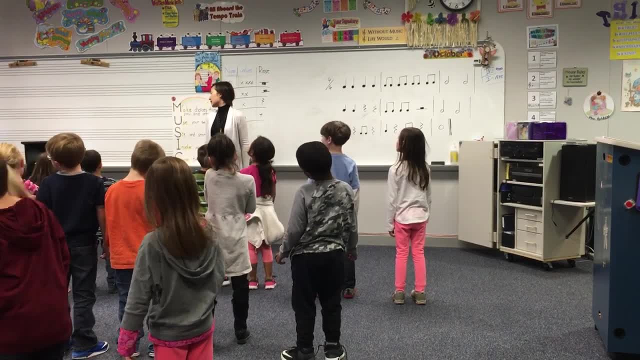 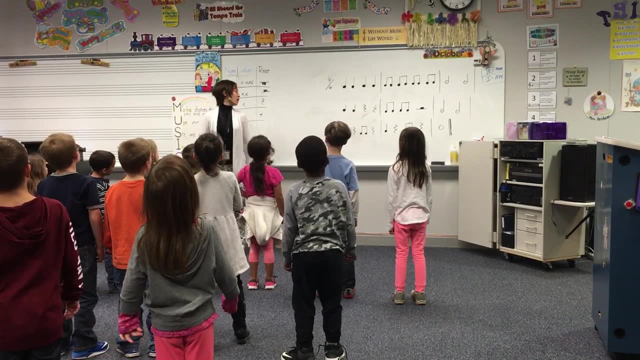 They want some inks, ink, quicky, squishy, wooshy, brainy snacks. They want some squishy, bushy, plaggy, very brainy snacks. They want brainy snacks. If they are wooing they might be drooling. 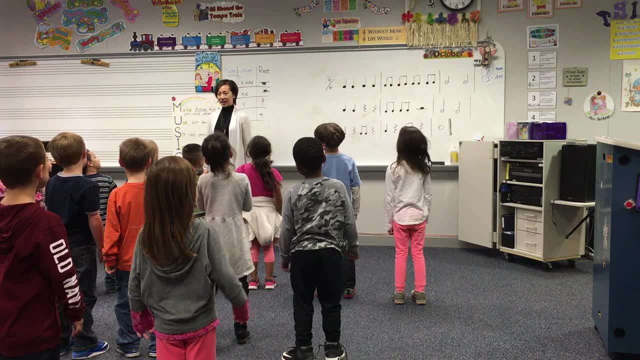 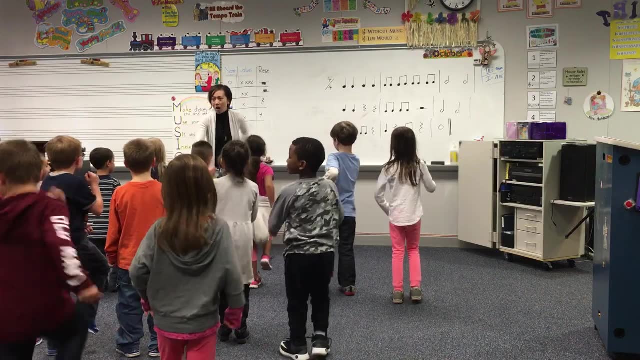 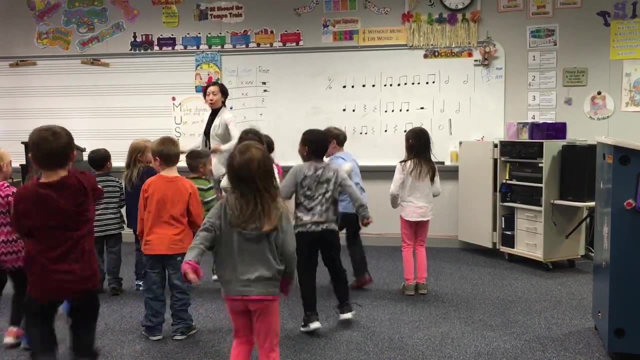 but they are zombies. They're really zombies. They might be dancing while they're advancing, but you must run, oh, you must run. Just run as fast as you can, Run as fast as you can, Run as fast as you can. Three, two, one. 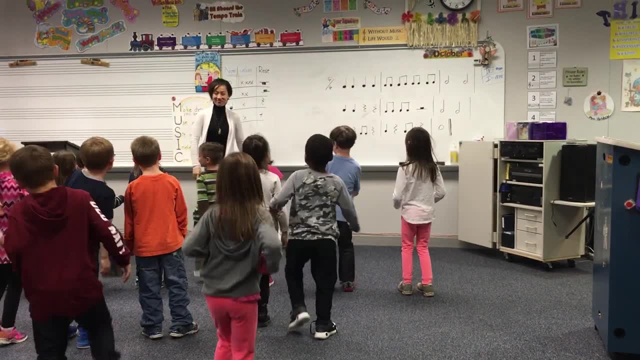 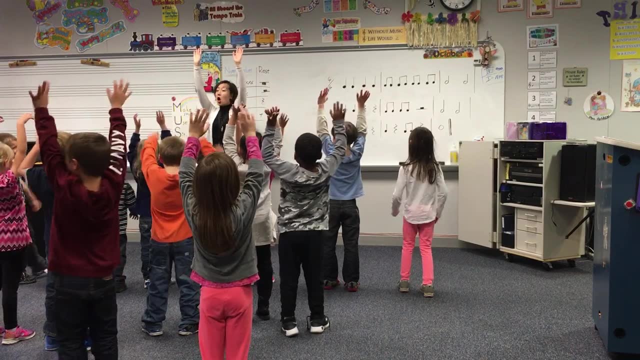 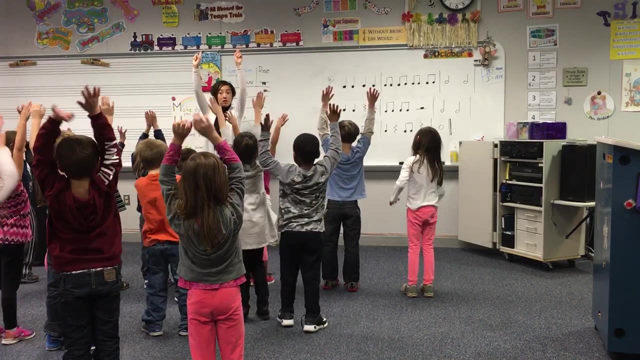 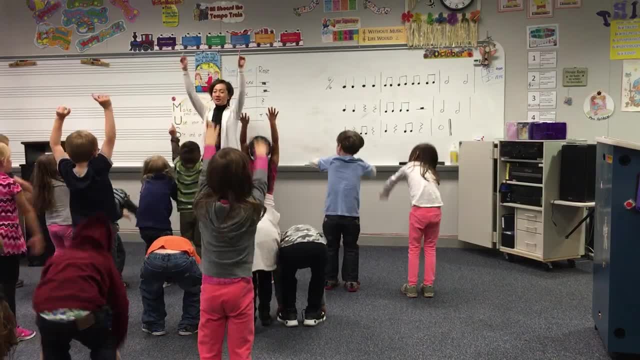 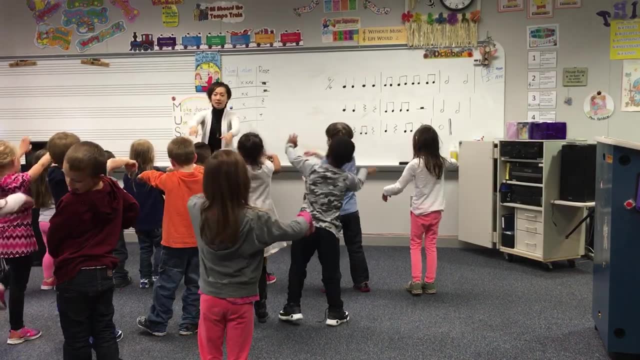 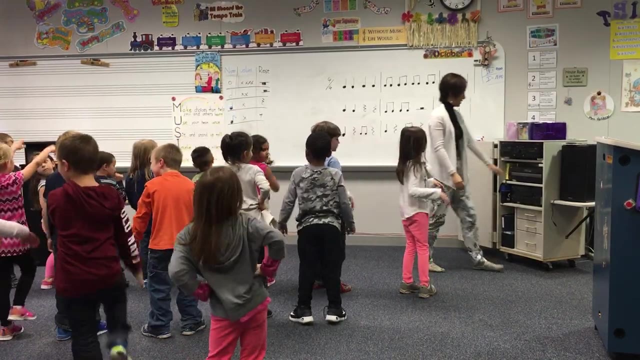 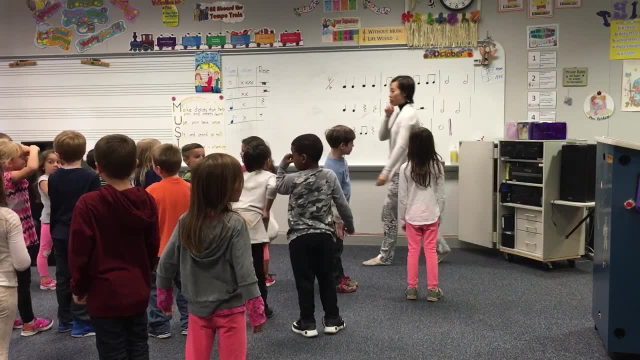 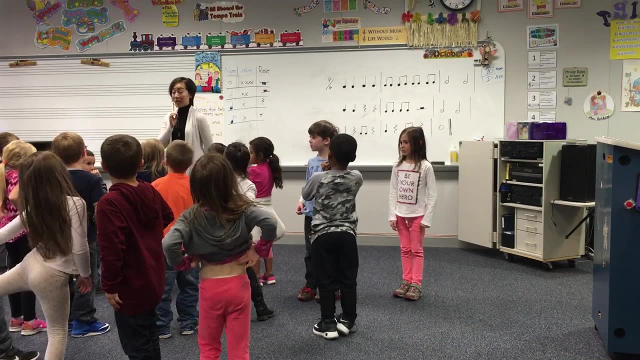 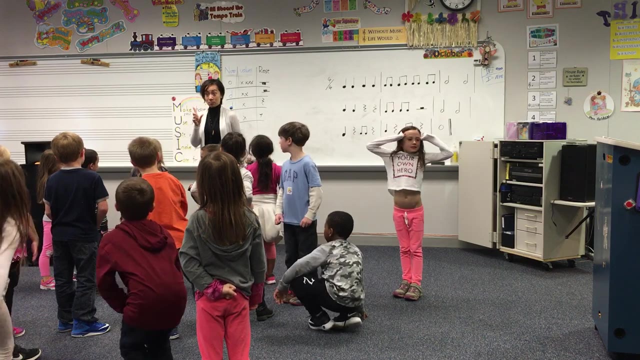 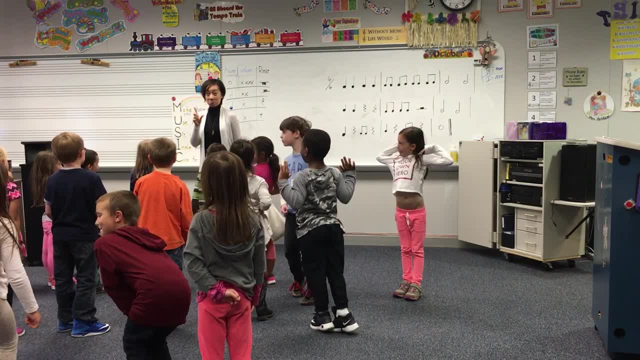 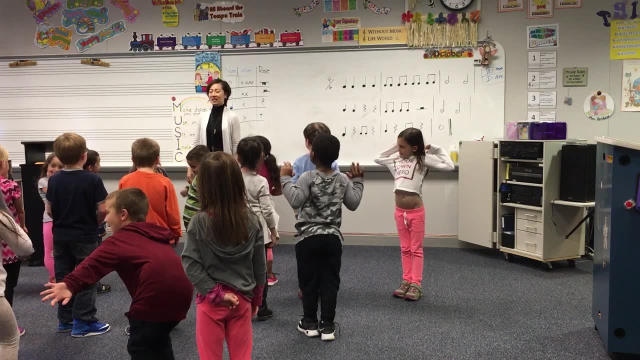 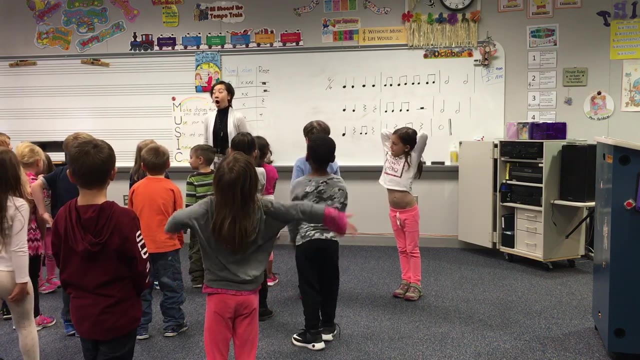 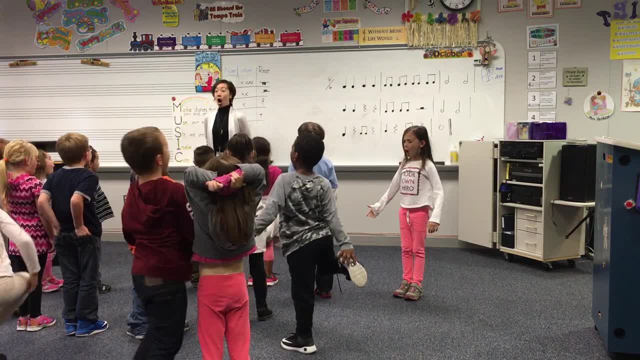 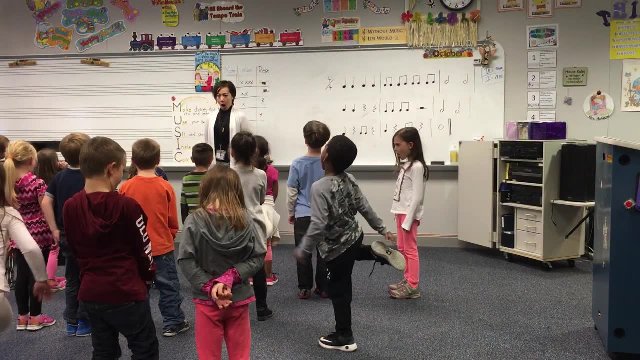 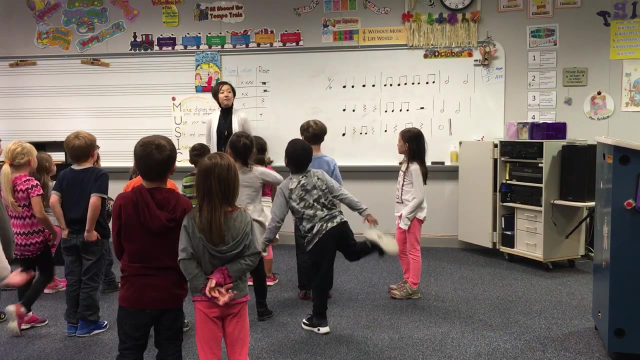 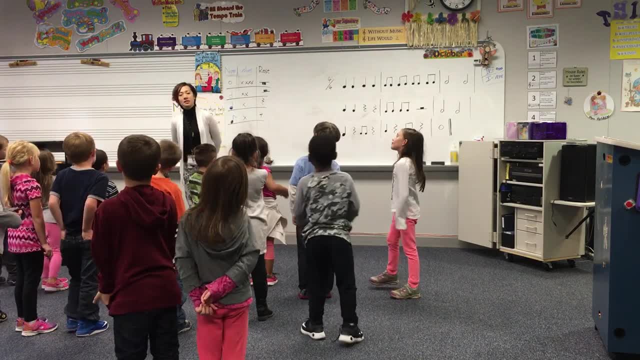 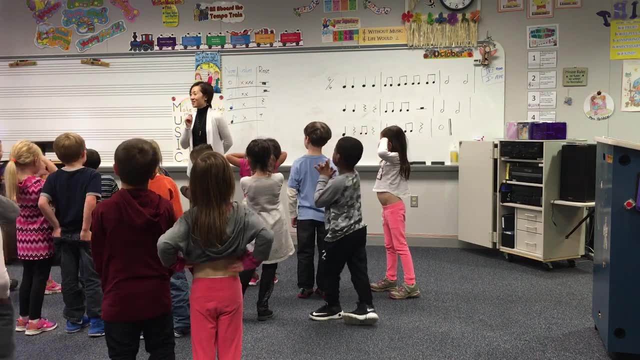 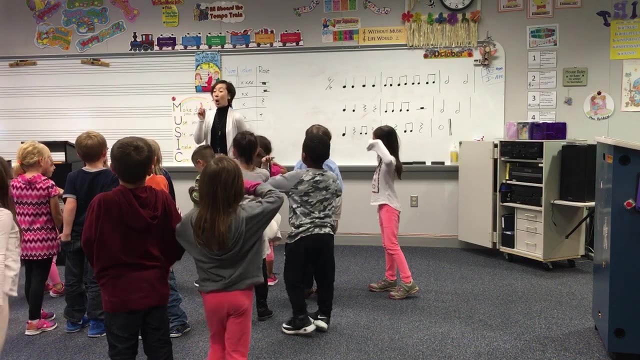 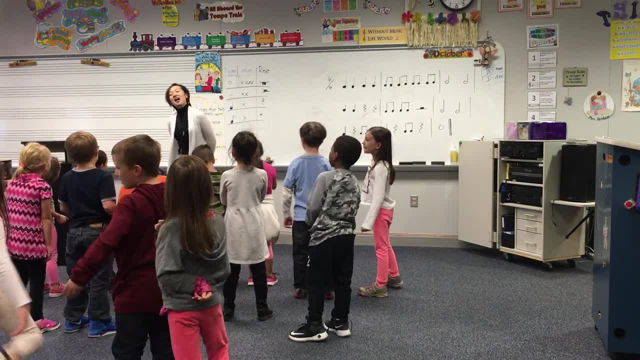 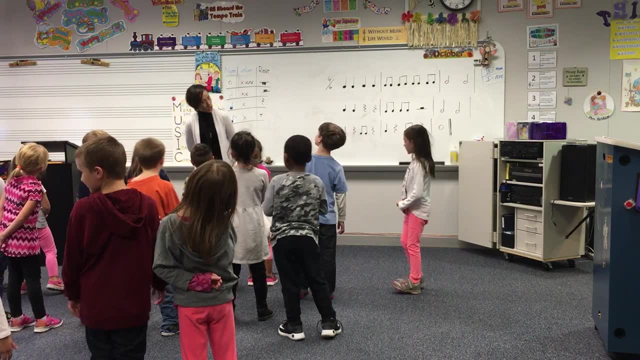 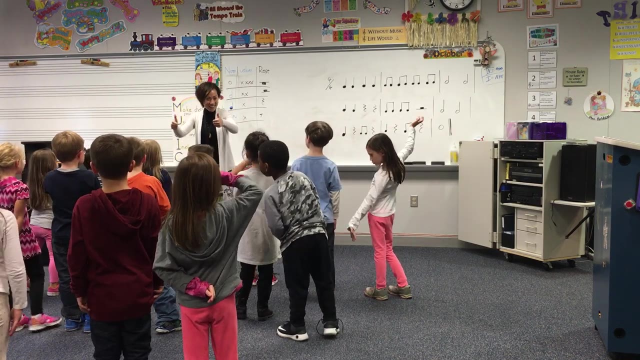 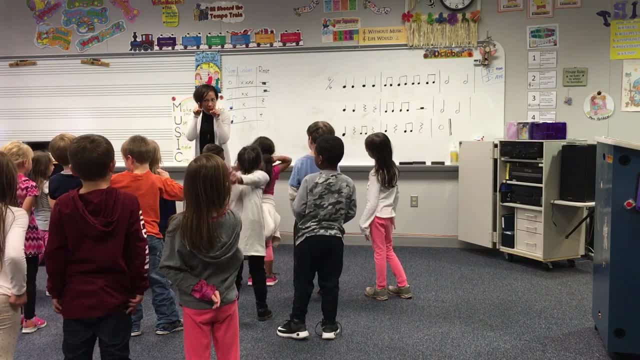 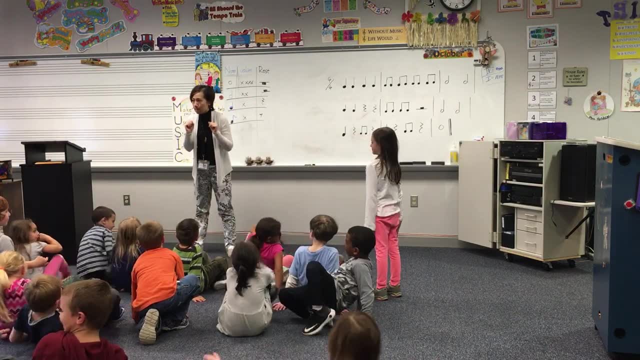 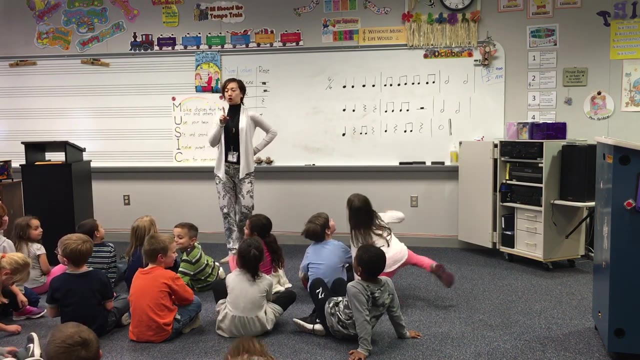 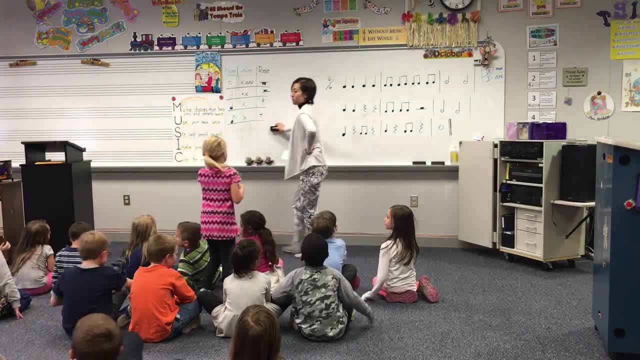 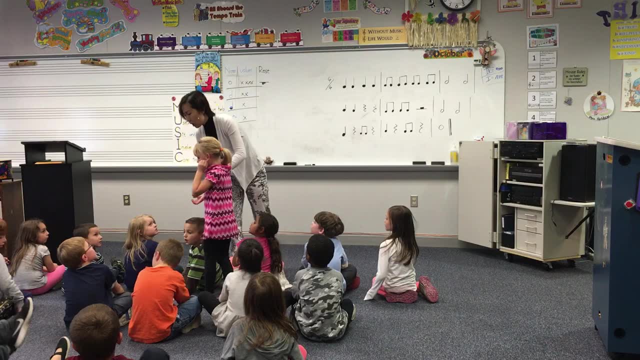 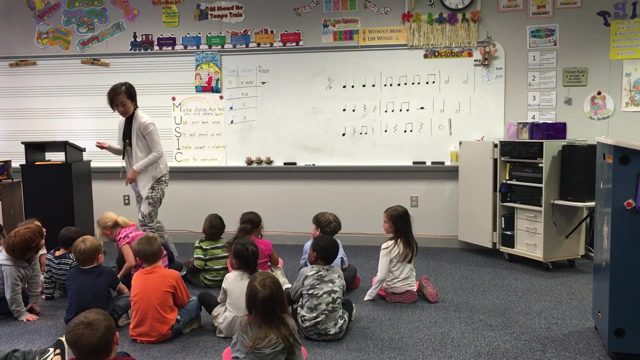 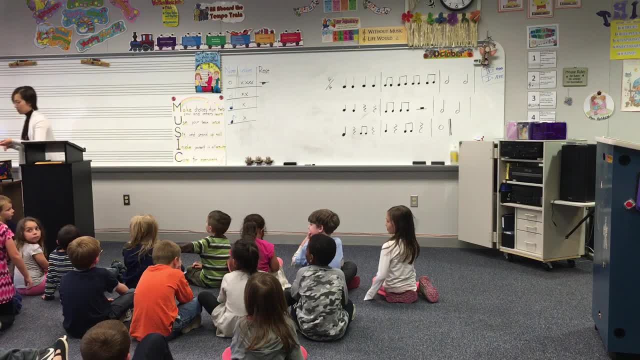 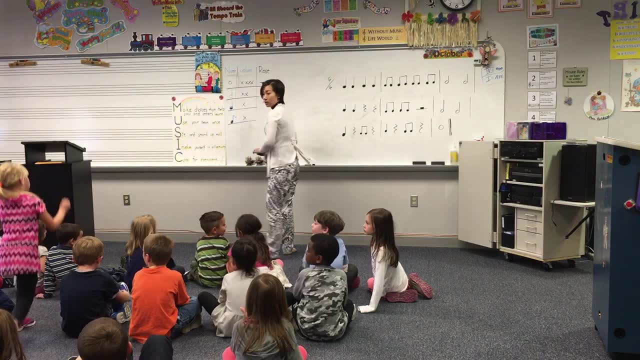 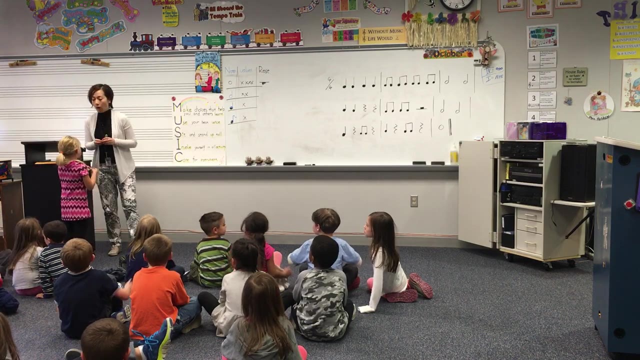 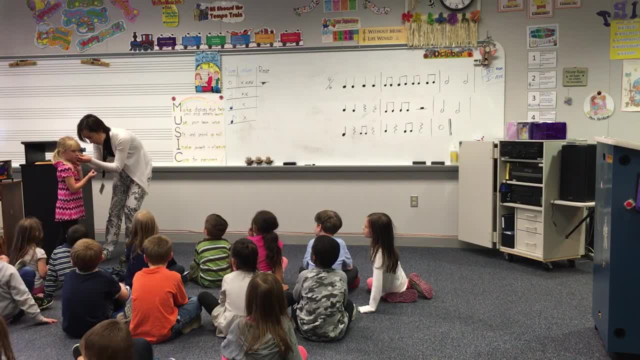 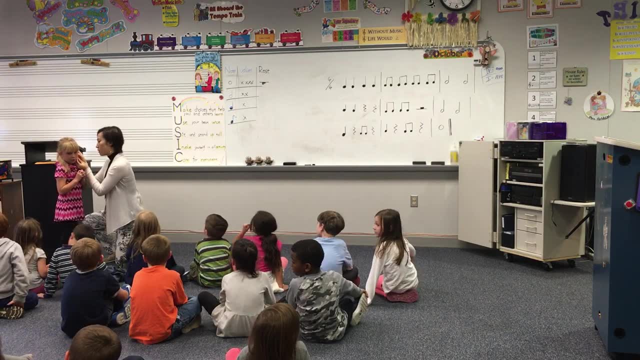 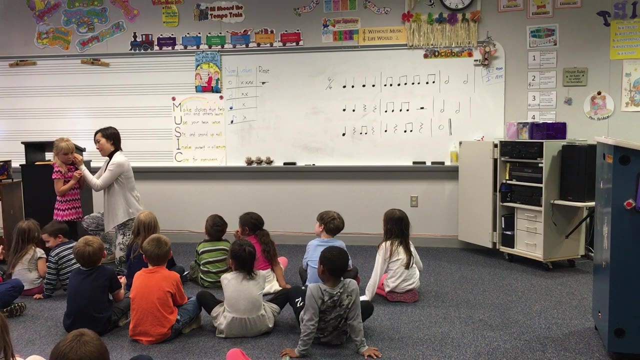 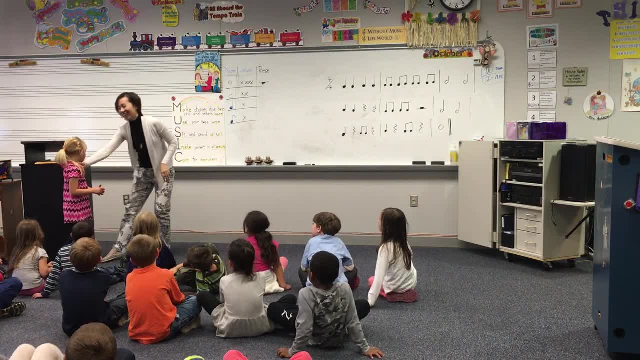 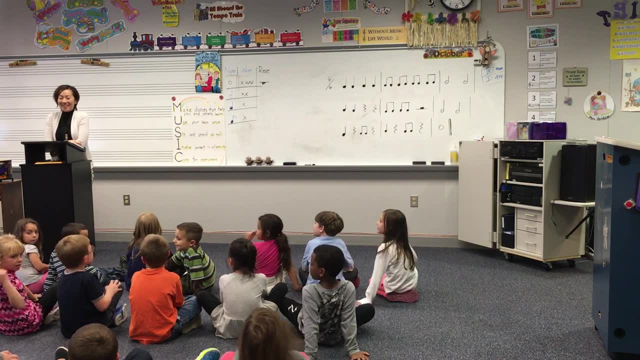 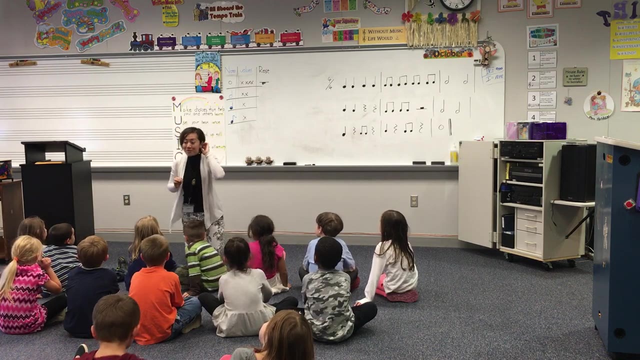 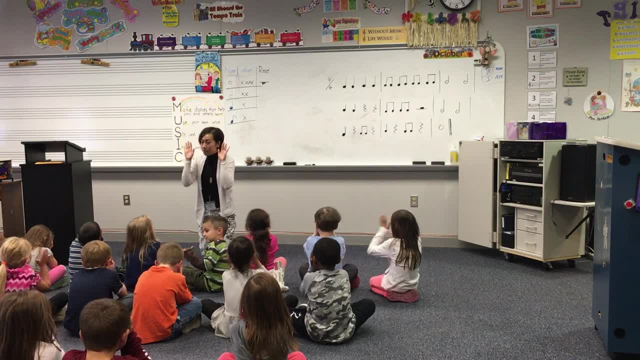 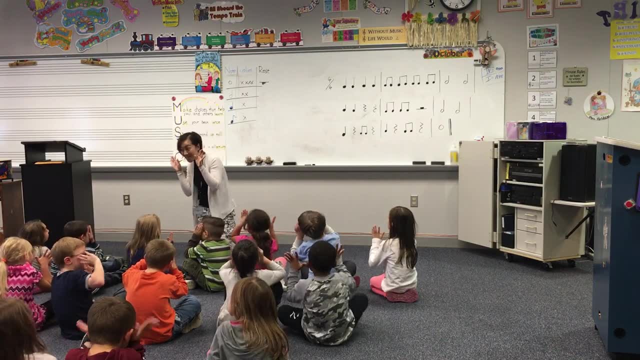 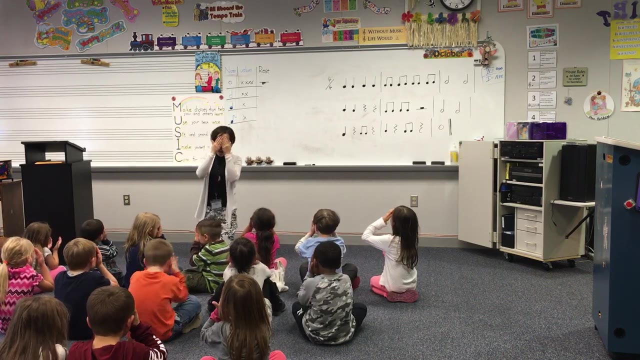 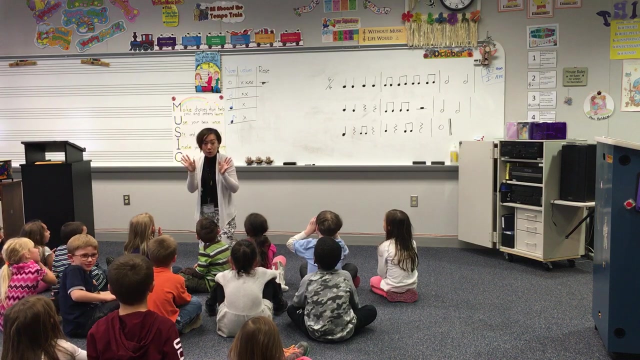 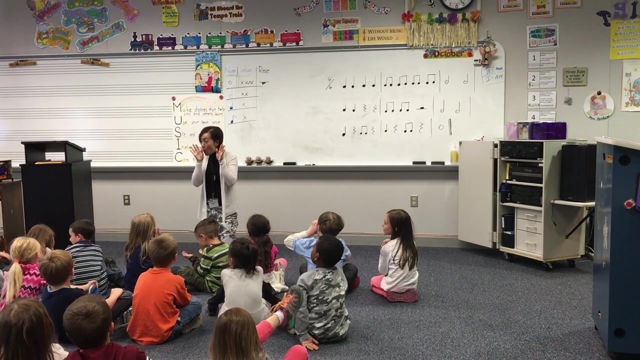 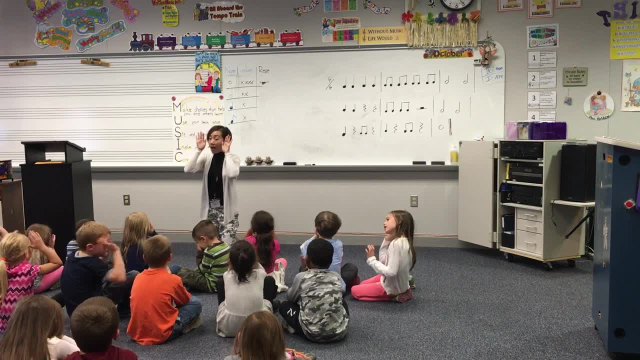 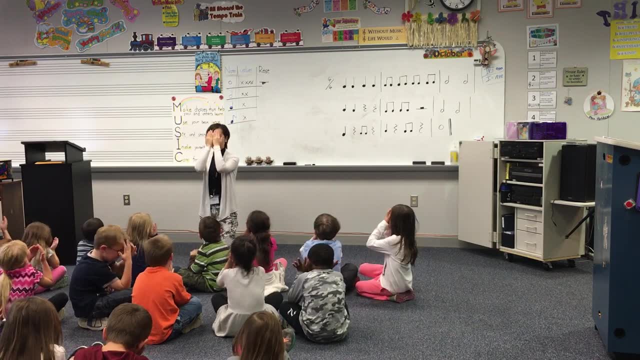 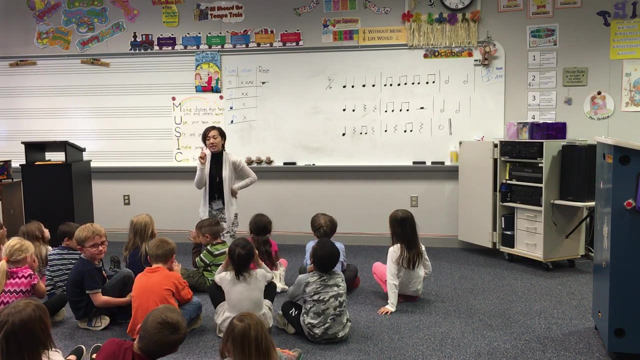 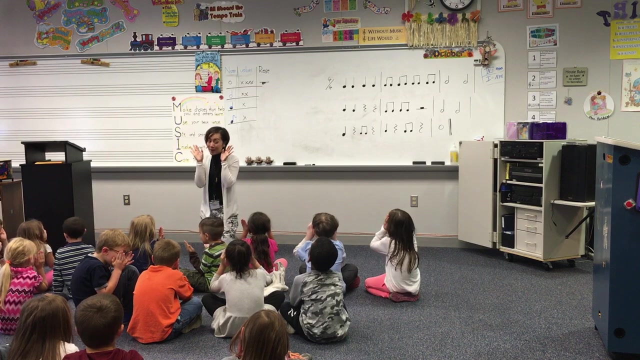 One, two ready, go, Boo, Now Jaden. One more time Jaden, One, two ready, go, Peek-a-boo. It's been Kaden. Shhh, Very soft, Lisa, Peek-a-boo, I see you, Peek-a-boo, I see you. 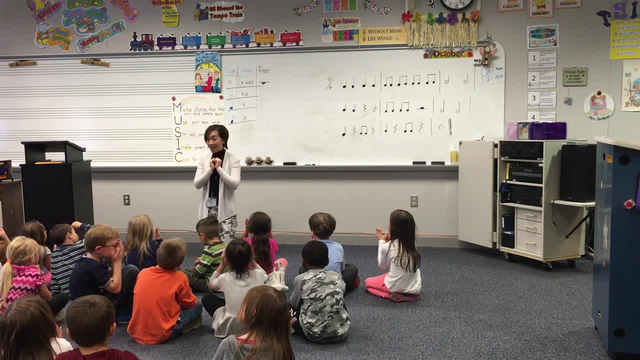 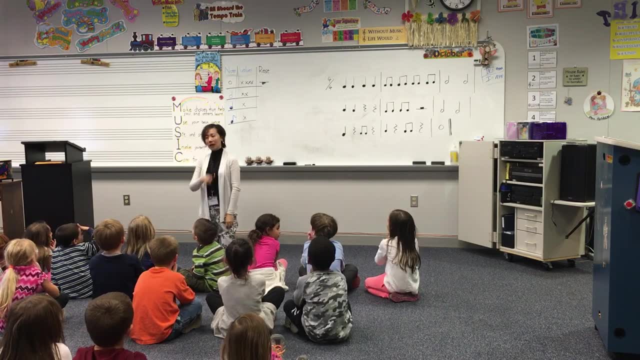 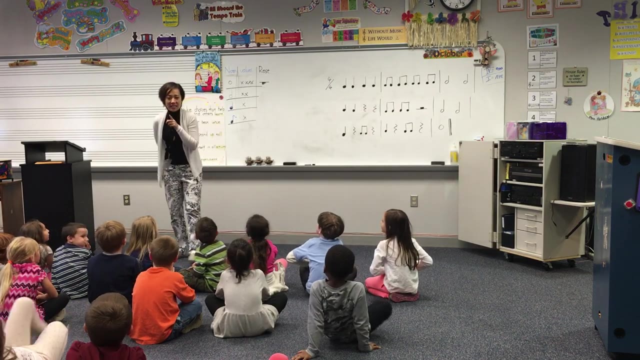 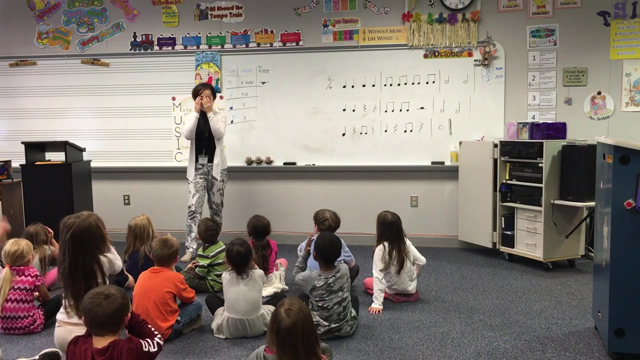 Peek-a-boo. I see you. Happy Halloween. I like this one Soft Boo Boo, Boo, Boo Boo. How about this? Let's all say a loud boo together: One Get ready. One, two ready boo. 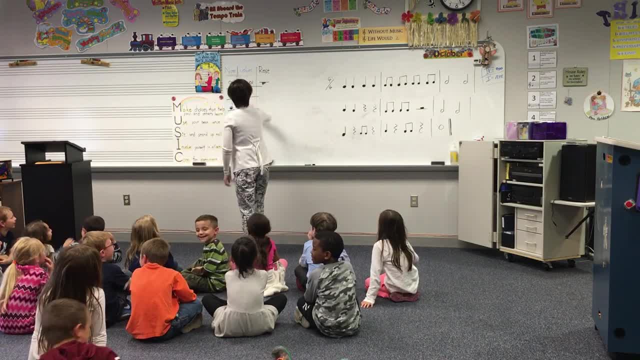 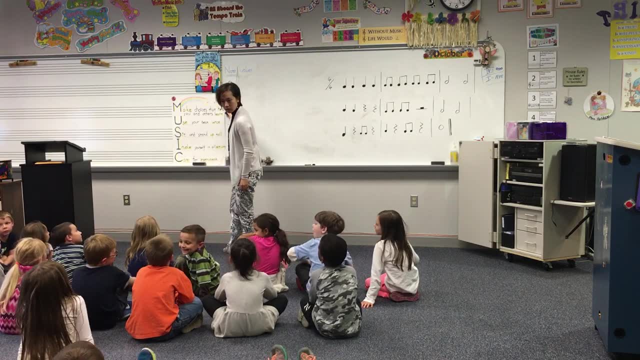 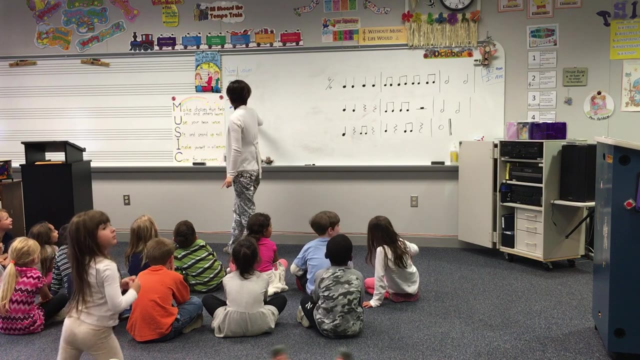 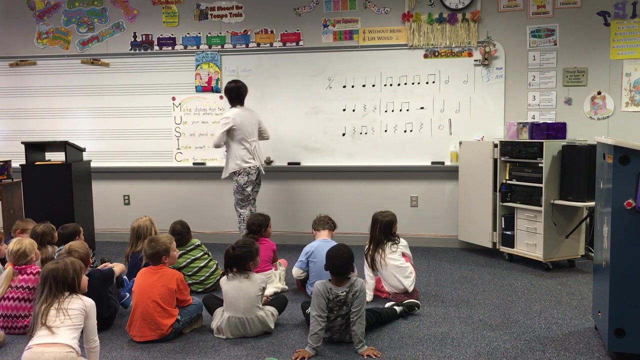 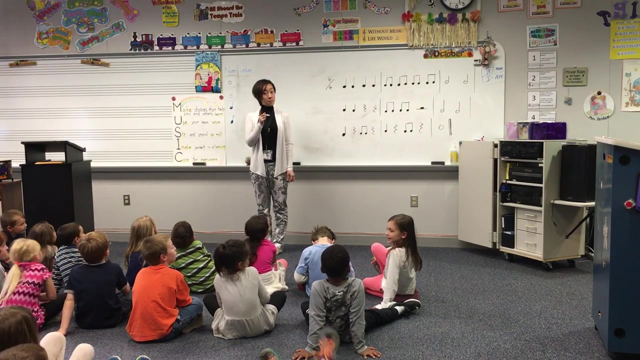 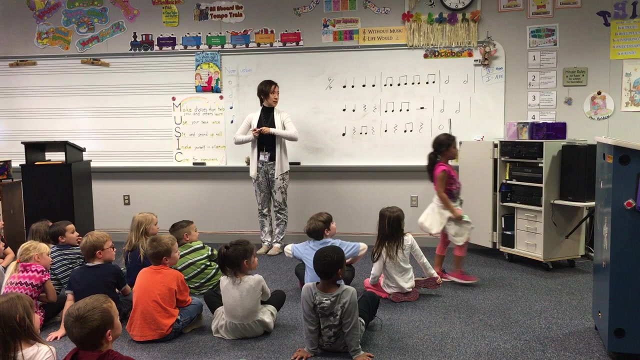 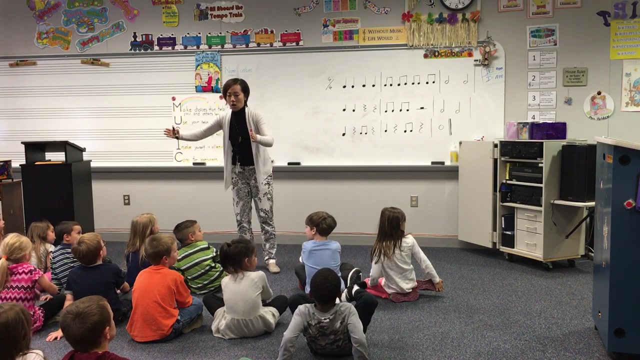 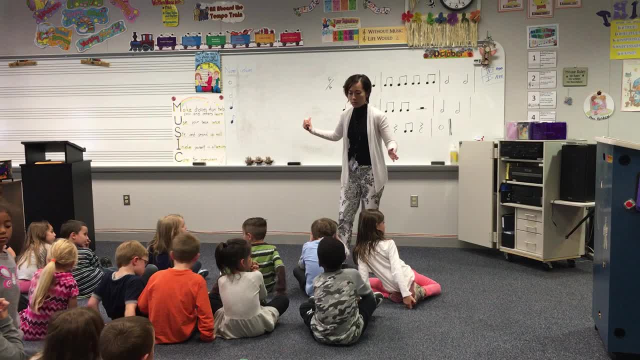 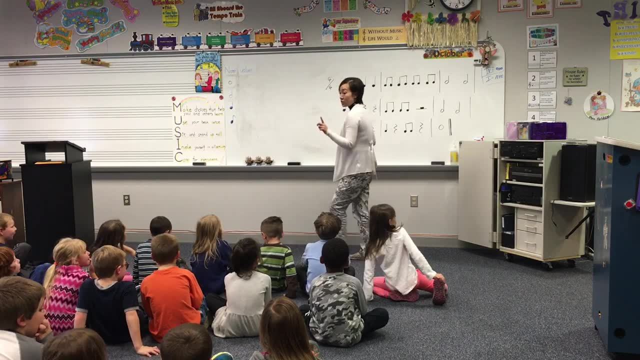 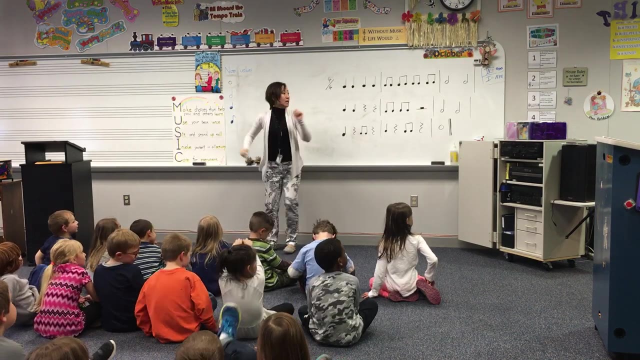 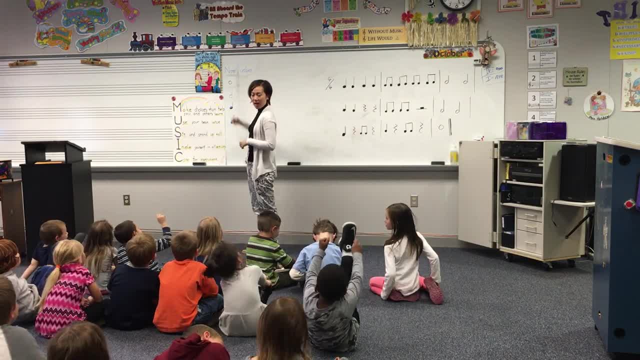 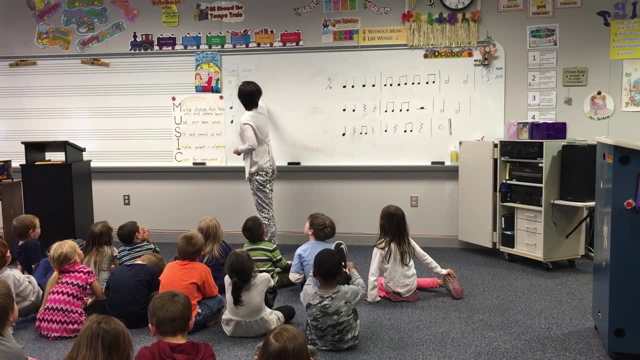 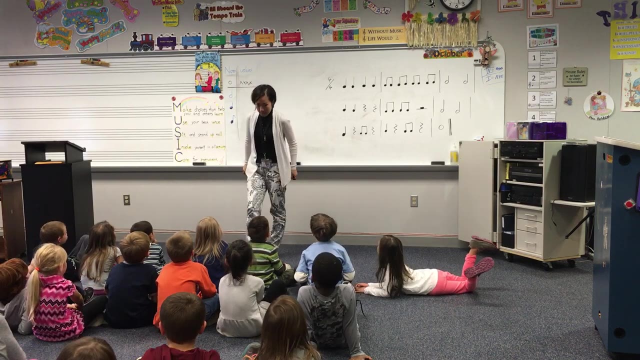 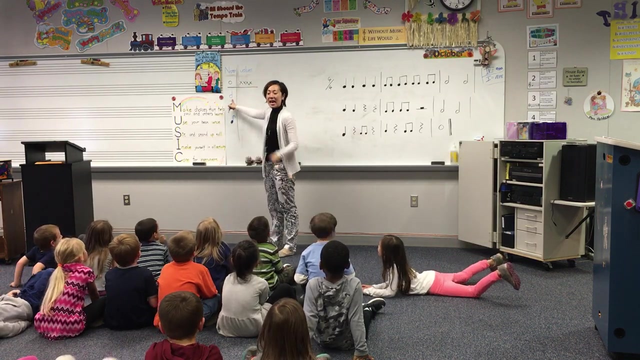 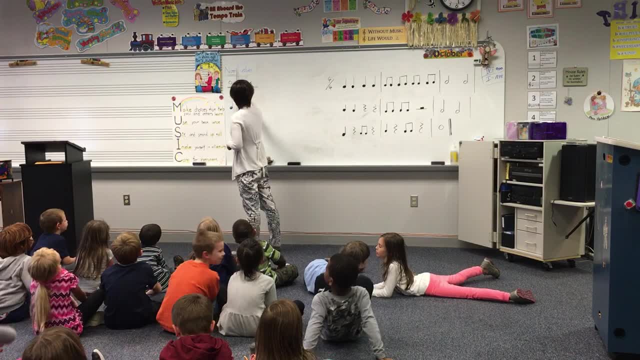 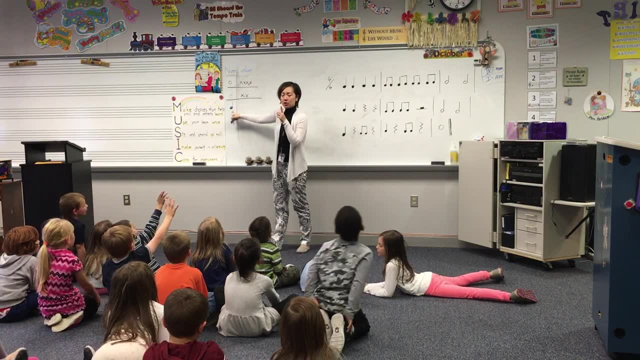 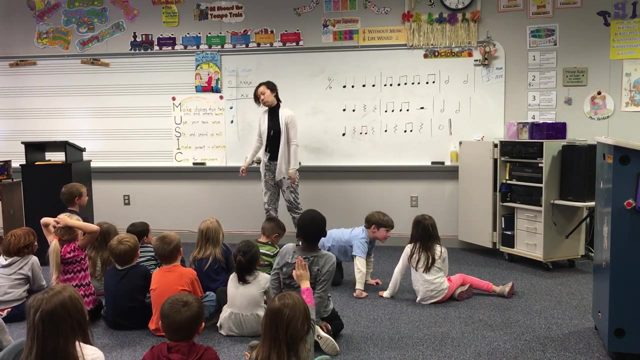 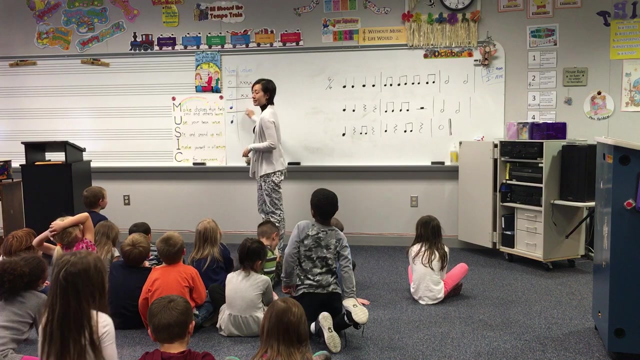 How many bees? Two. What's the name of this cup? Quarter cup. Listen, Listen, Listen. Just to see Quarter cup, Quarter cup. I tell you. Just to see Quarter cup, Quarter cup. How many bees? One. 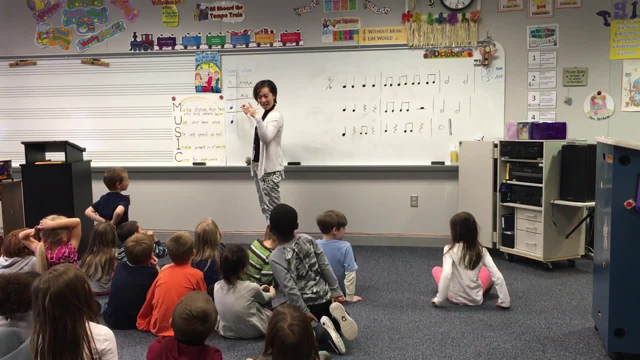 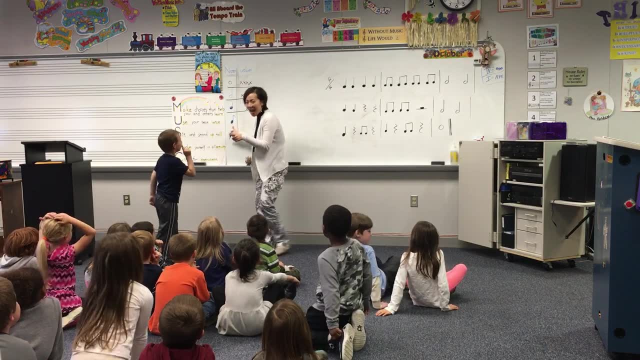 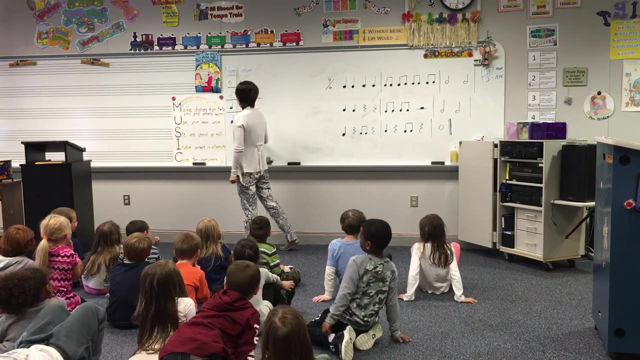 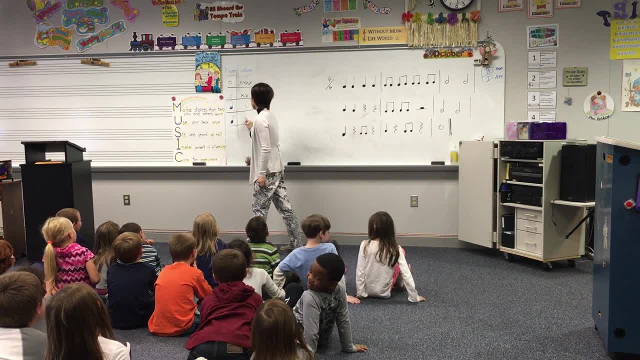 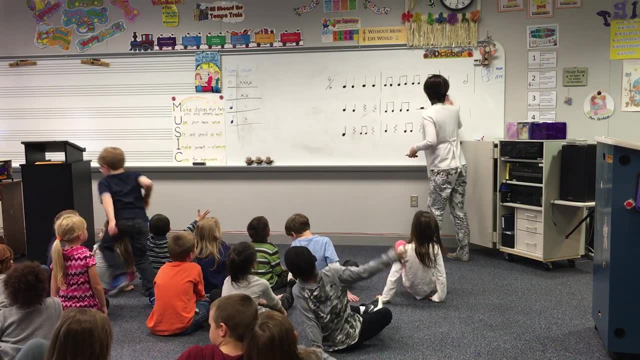 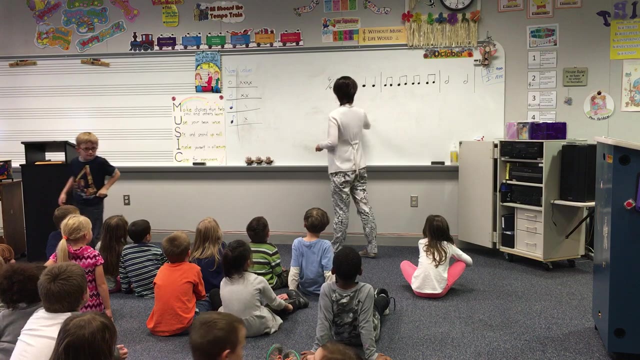 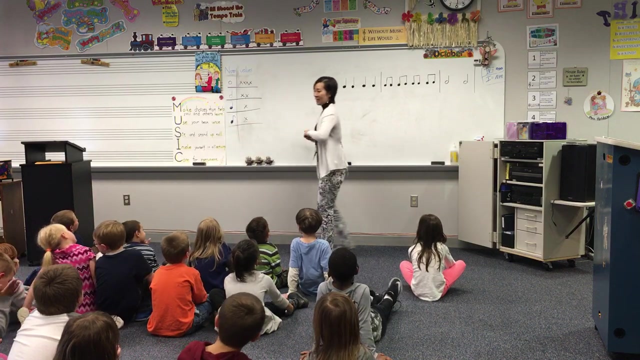 Half a bee, Half a bee, Half a bee. Listen, Listen, Uh-huh, Oh, thank you. Now I'm going to say that, Yeah, Yeah, I see, Thank you. Oh, blue, Blue, Blue. 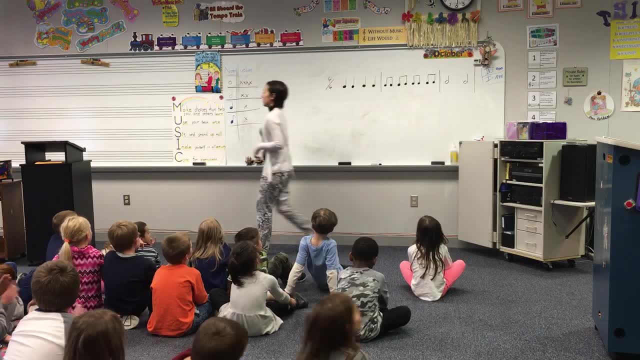 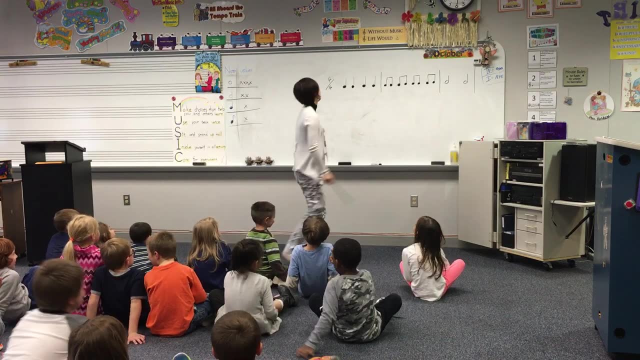 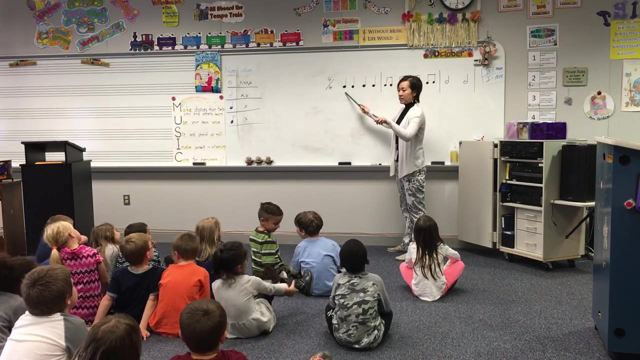 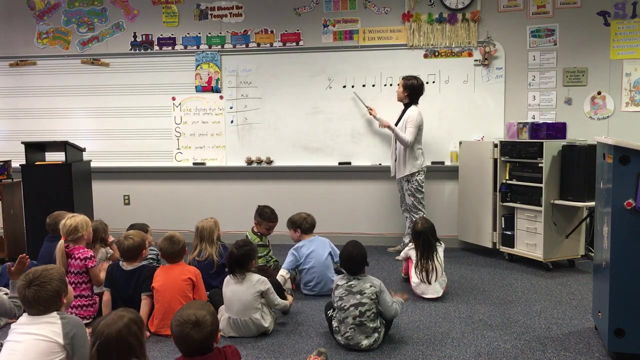 Blue, Two: Good Face my feet, This one. ladies and gentlemen, Sit up, sit up. This is a What note? Quarter, Quarter note. We say: tap, Tap, Tap, Tap, Tap, Tap, Tap away. 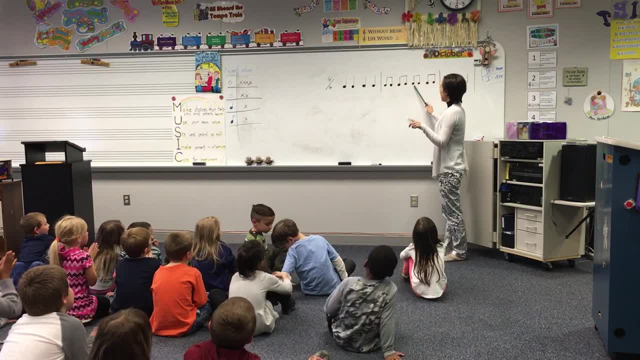 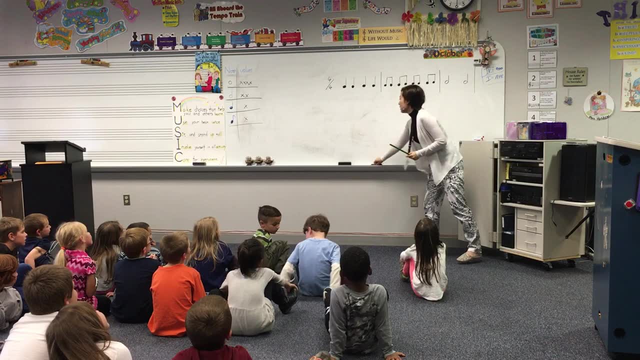 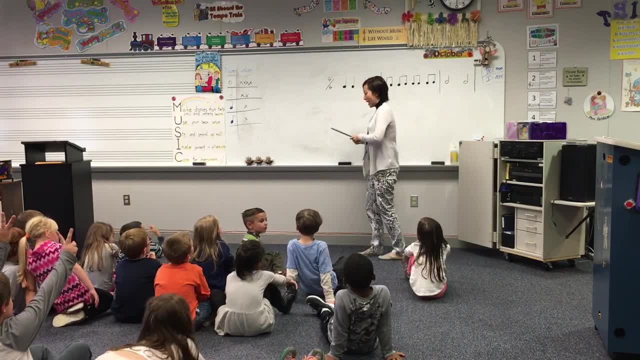 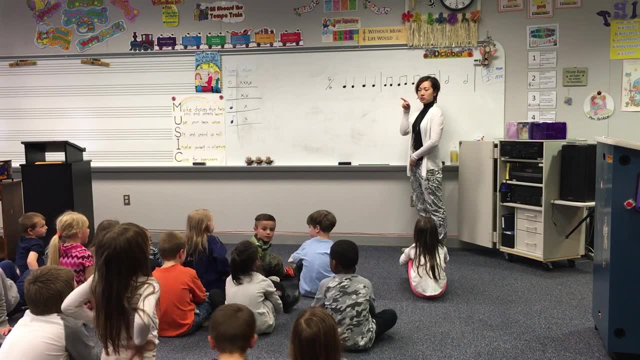 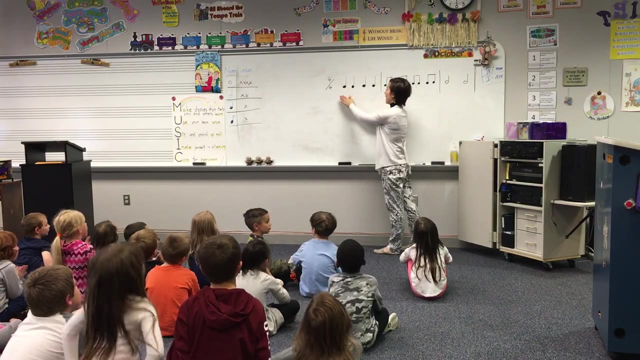 So how many bees fall in half-nose? Two, Two, right. So listen, Listen and watch. Sit on the bottom, sit up tall, Listen and watch. One, two, three, Ta-da, ta-da, ta-da, ta-da. 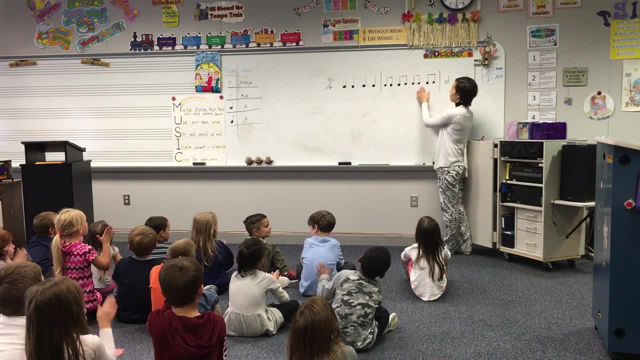 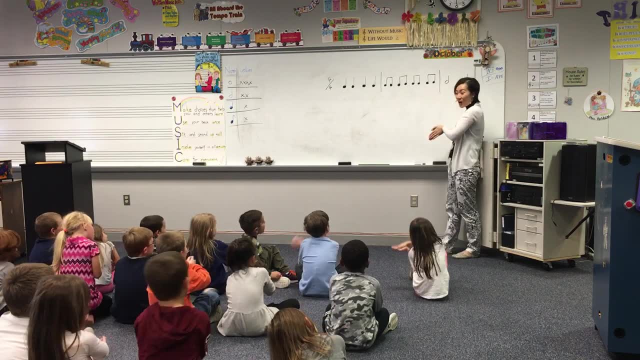 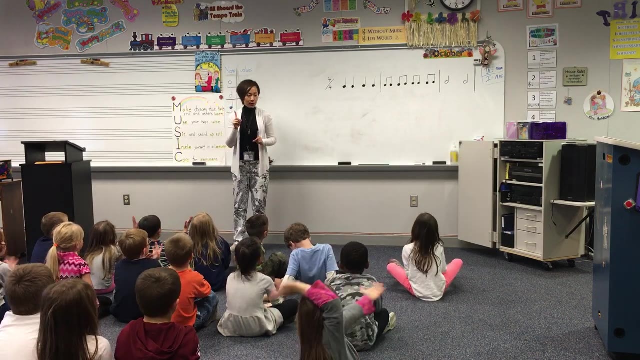 Ti-ti-ti-ti-ti-ti-ti-ti-ti-ti-ti-ti-ti, Play some Tu-wu tu-wu. Good job, Let's, clap tu-wu together. One, two ready go. 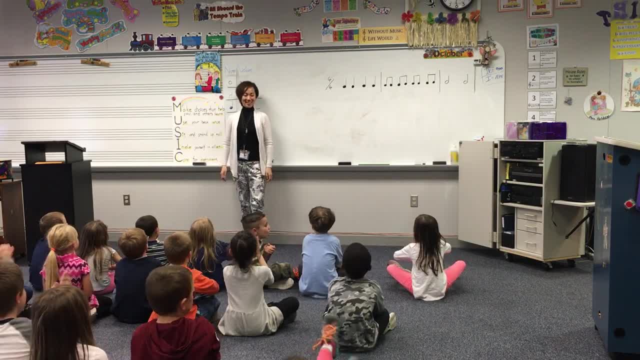 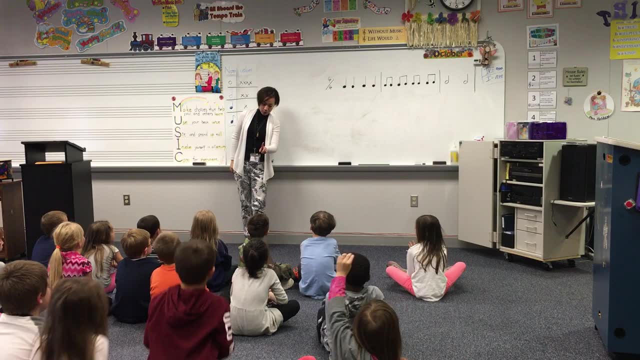 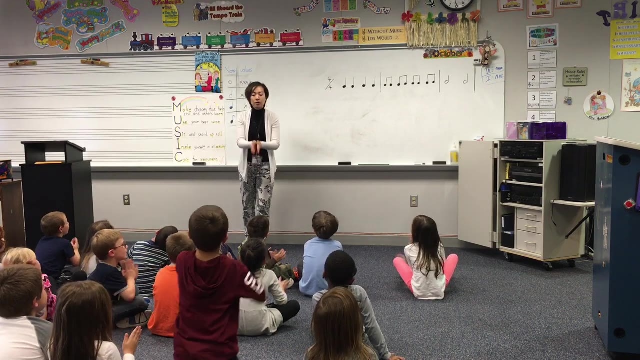 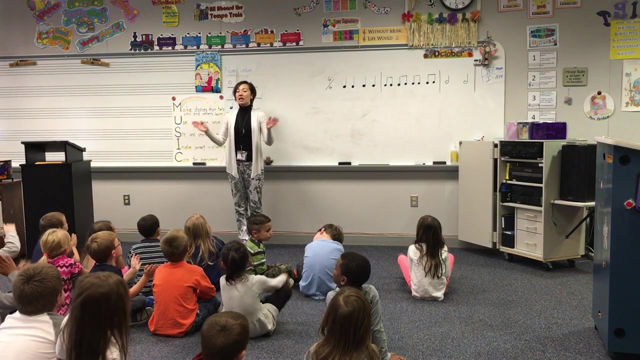 Two, two, two, two, two, two, two. How to clap? two, Two, two, two, two, two. How about ta One two ready go, Ta, ta, ta, ta ta. 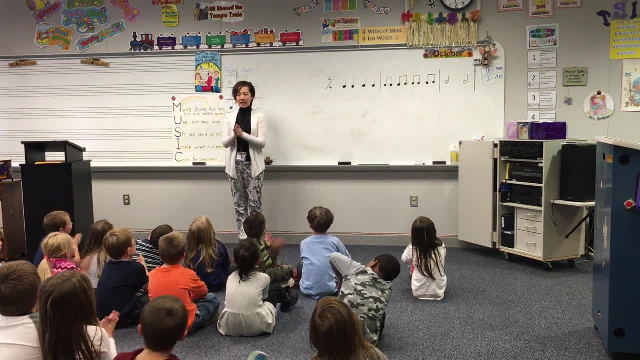 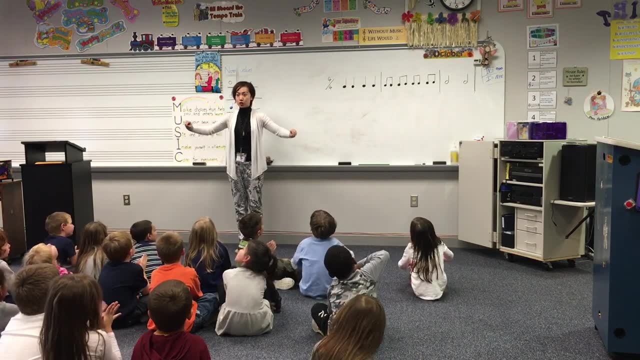 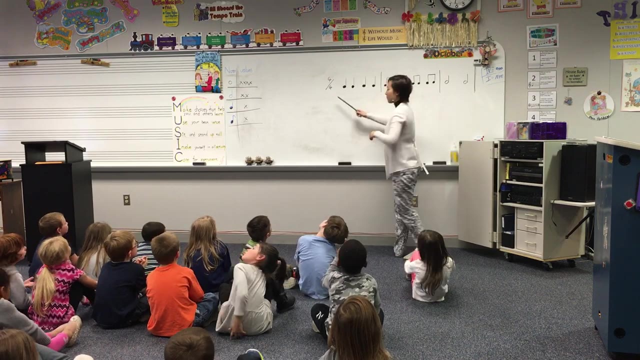 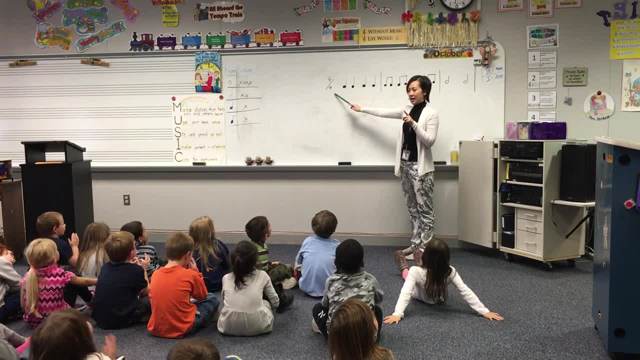 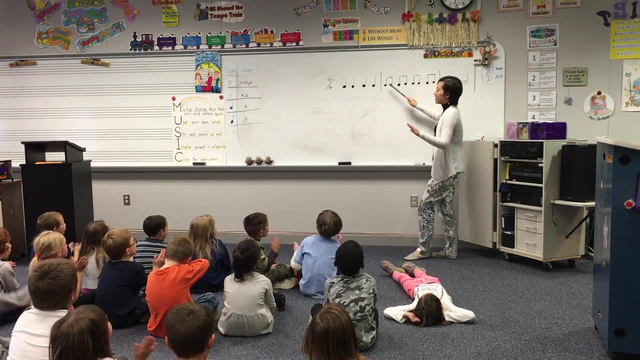 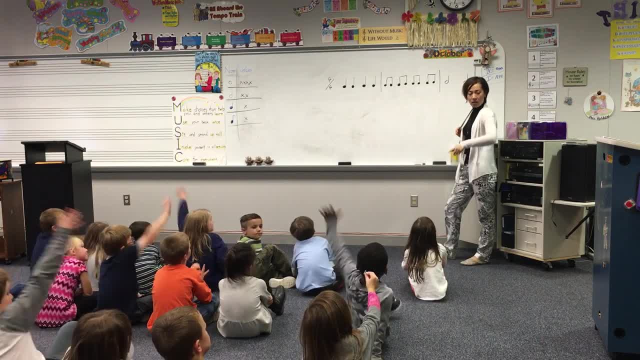 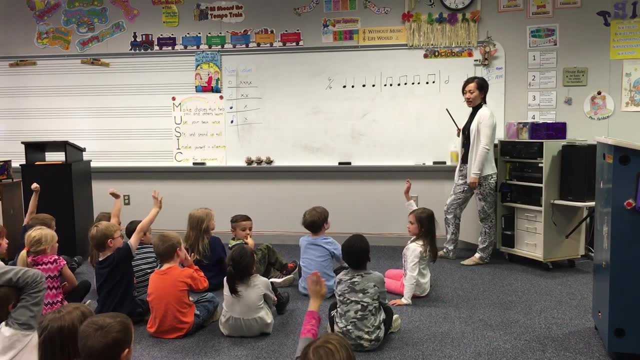 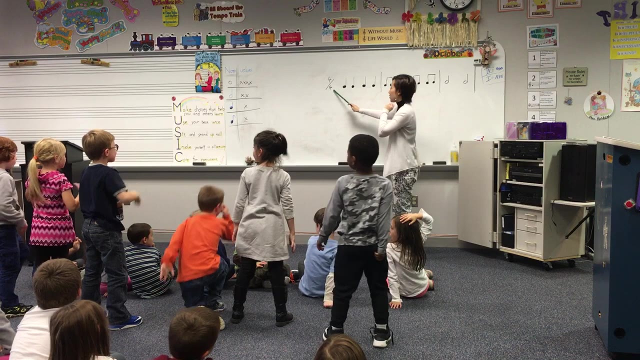 Nice, Which row wants to try? Me, me, me, me, me, me. Sit on top, sit on your bottom, I will see which row, Second row, stand up, Let's try. One, two ready go. 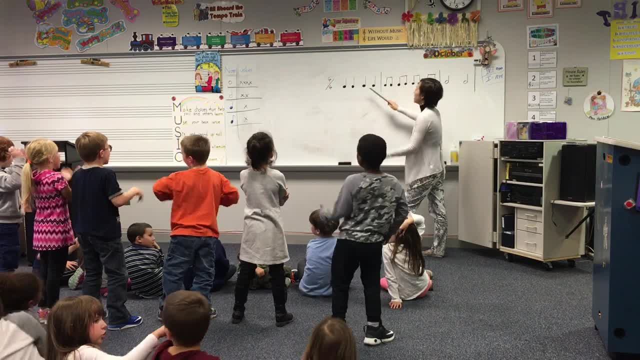 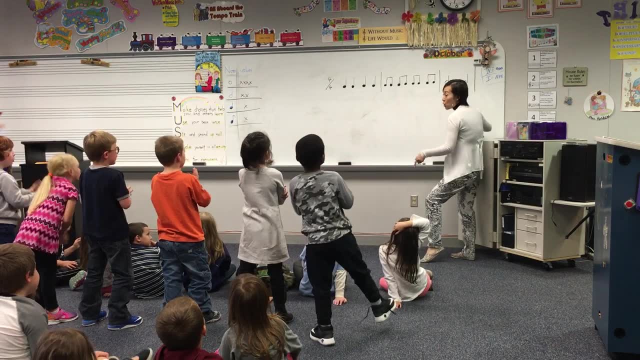 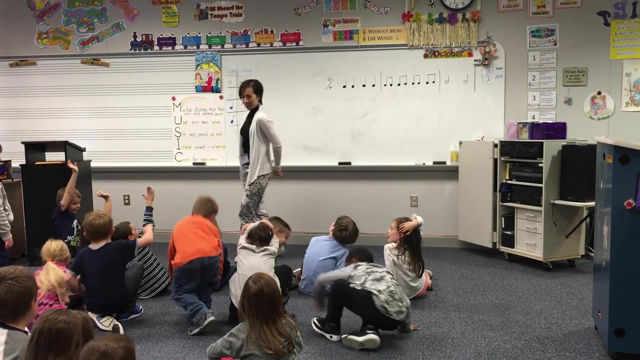 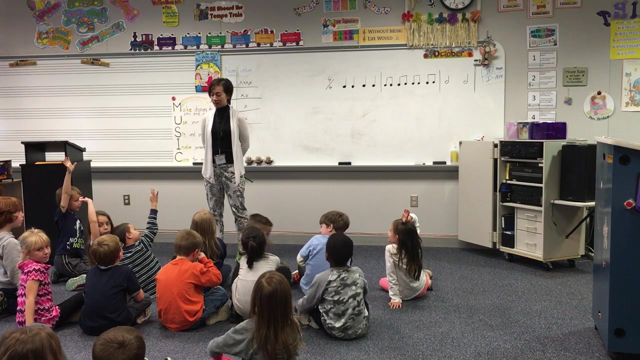 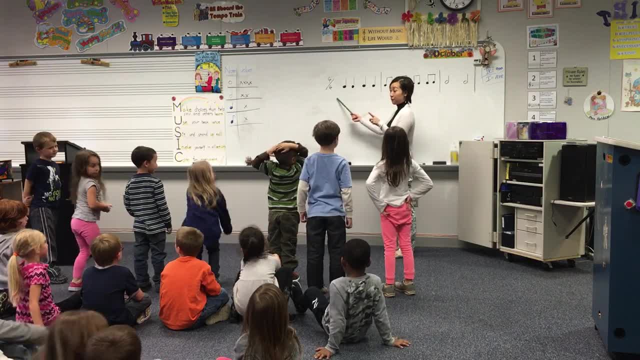 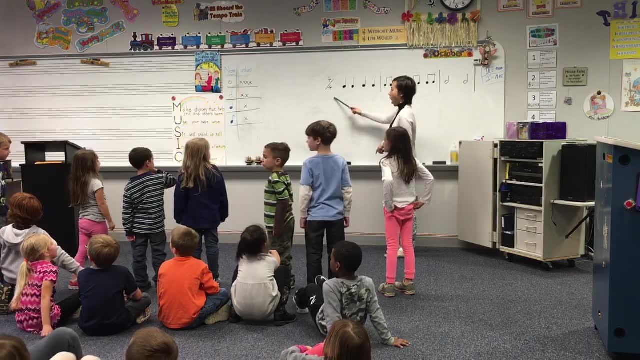 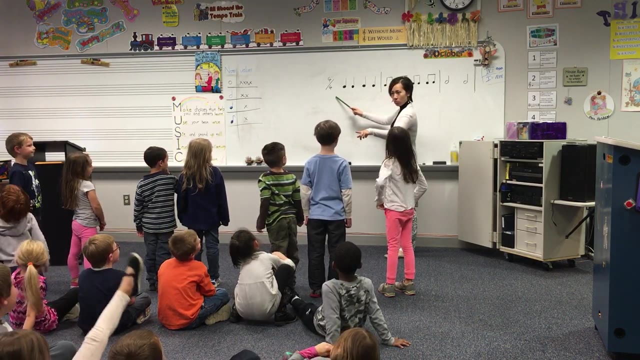 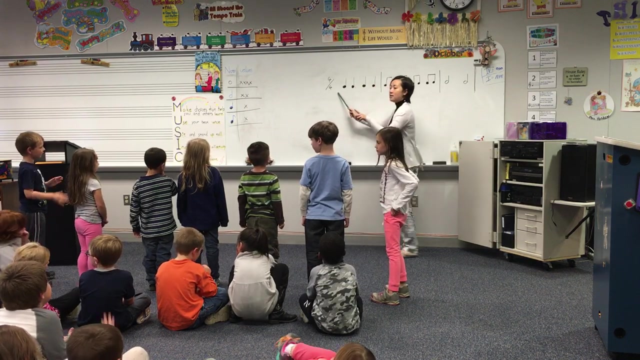 First row. One, two, three. First row. You want to play one more time? Go Good, Oh, wow, No, no, Sit down. Why are you yelling? Just talk One, two, Ready, go. 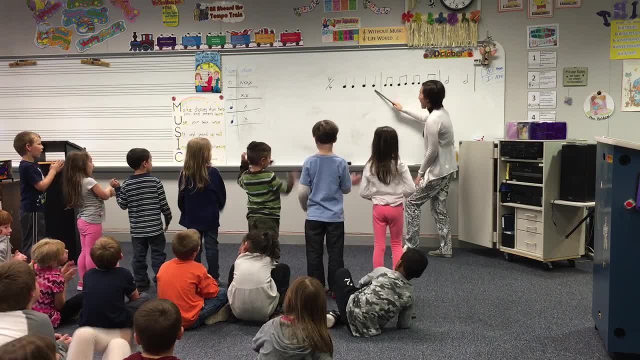 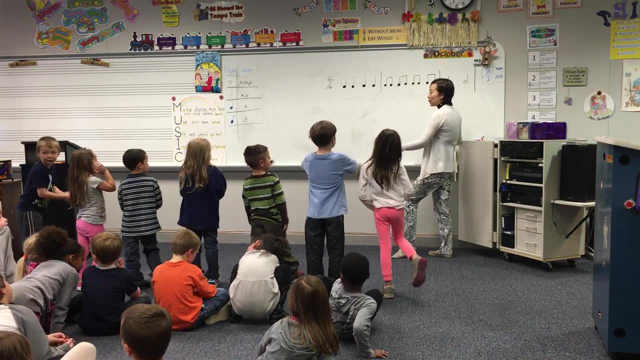 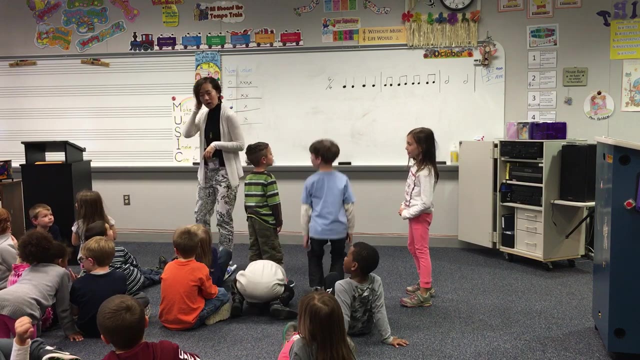 Ta, ta, ta, ta, Ti, ti, ti, ti, ti ti. Good job Tu tu. Very nice, Trevor, Sit down, Trevor go, Hurry, Hurry. Do you want to go or not? 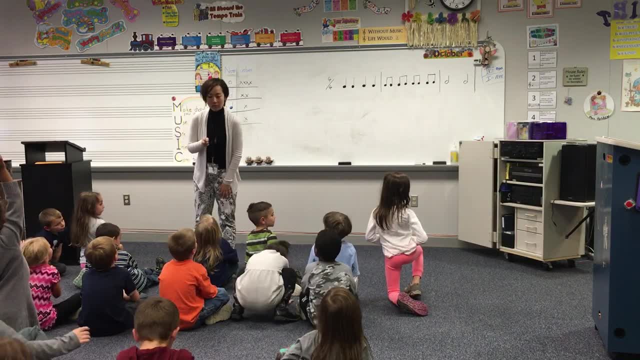 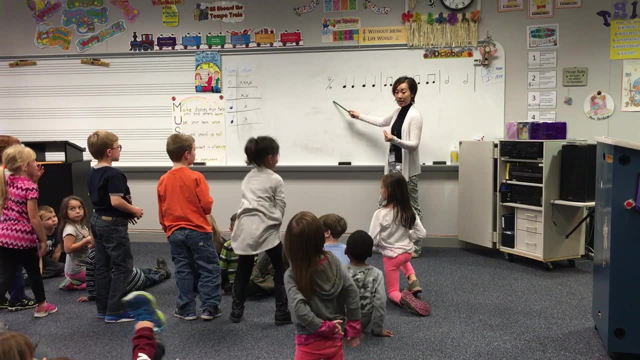 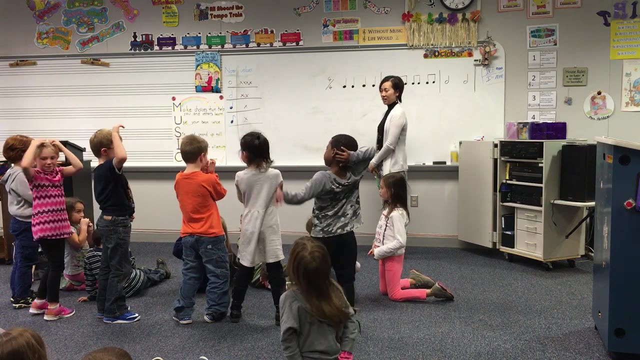 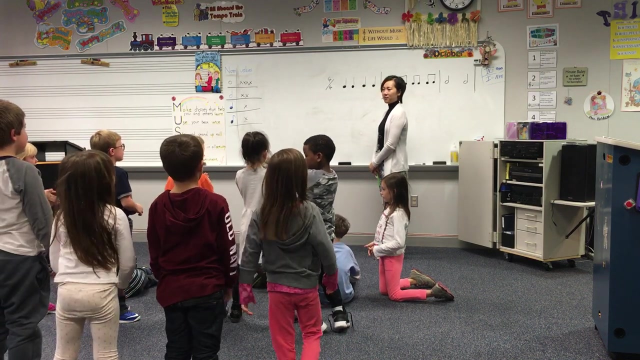 Hurry No more. Second row: stand up. Second row, Second row: come on, Hurry. stand up. Hurry One, two, Raise your hands. Third row: stand up, Clap your hands. second row. 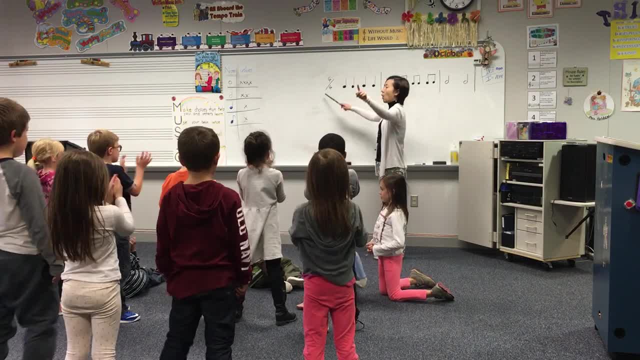 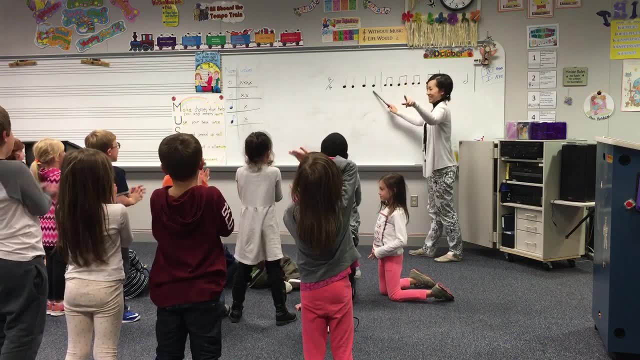 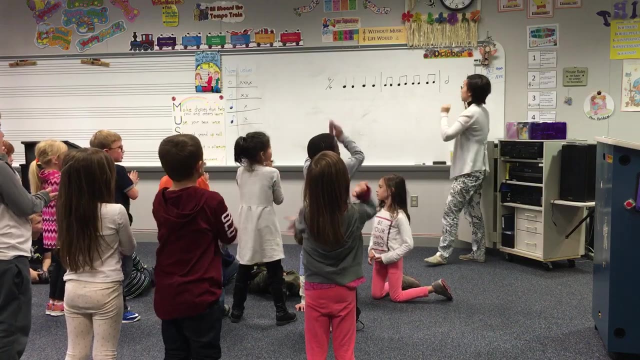 Very, very good model In front of you. One, two Ready go Ta ta, ta, ta, Ti, ti, ti, ti ti Tu tu. Good job. Sit down. Three Up. 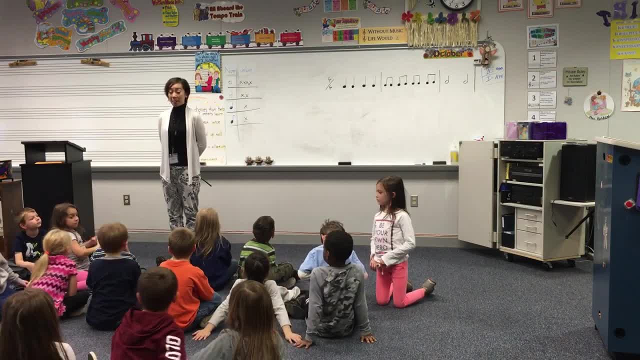 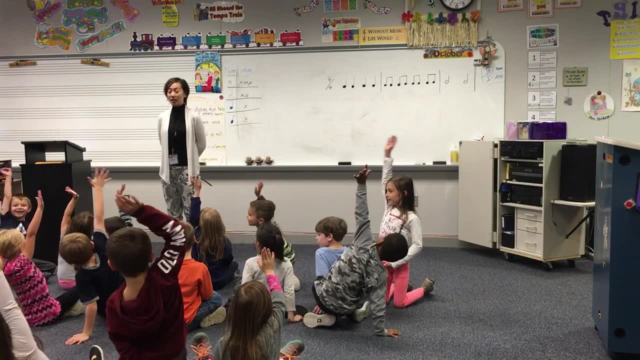 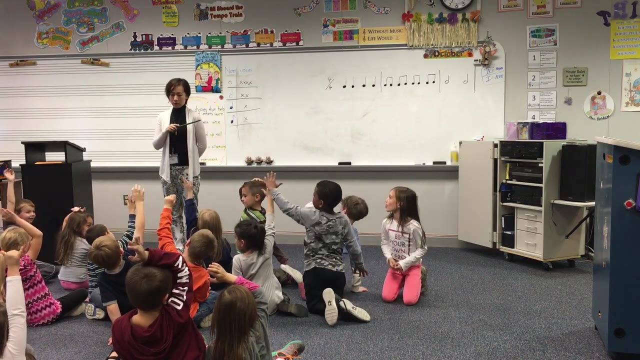 Oh, she's doing so good. Sit up tall and stay. Turn its arms, Move wise to the earth. Watch. Turn its arms, Vroom, Vroom, Vroom. Remember all the classroom rules, Because you built your background before. 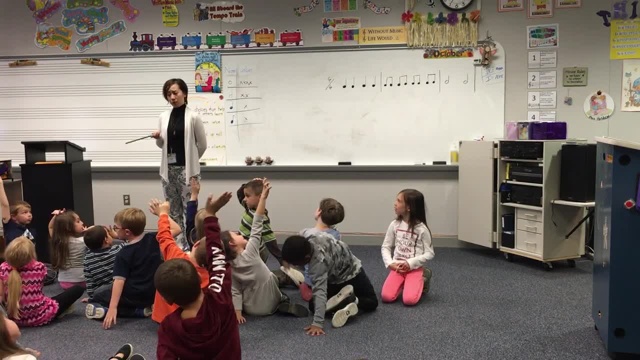 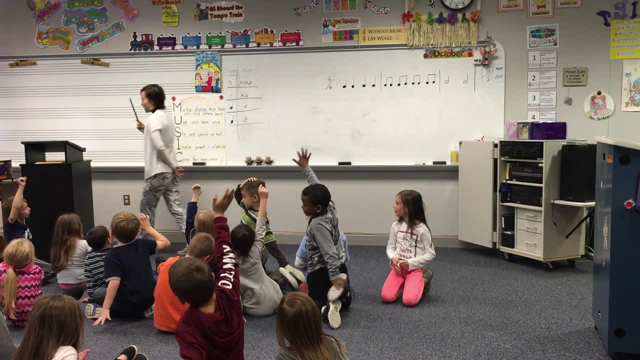 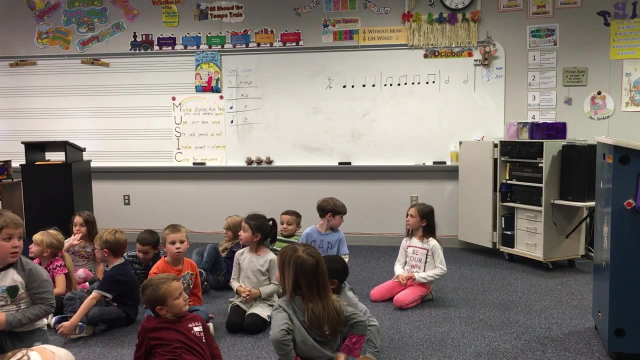 You come, Yeah. So if you built your background during that learning, you would be something. Oh, let's go to the dormitory, Turn around, Turn around, Let's get those moved over here. You want to do the weird select. 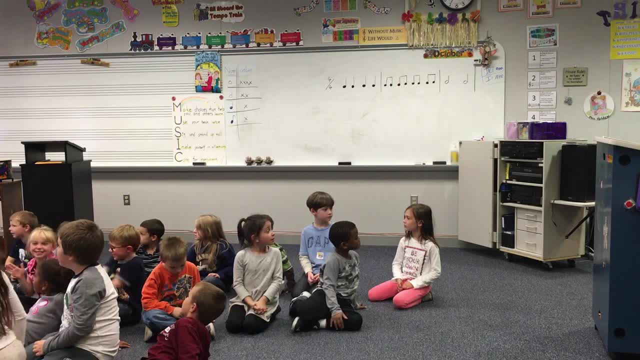 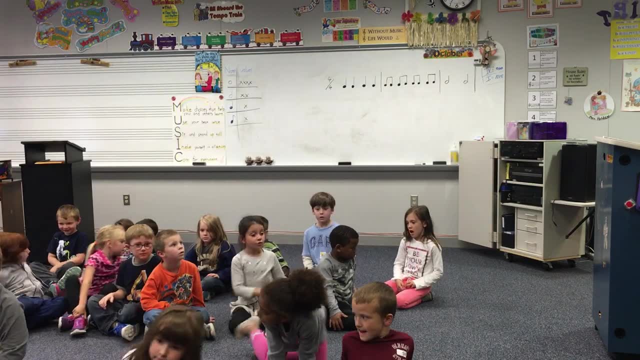 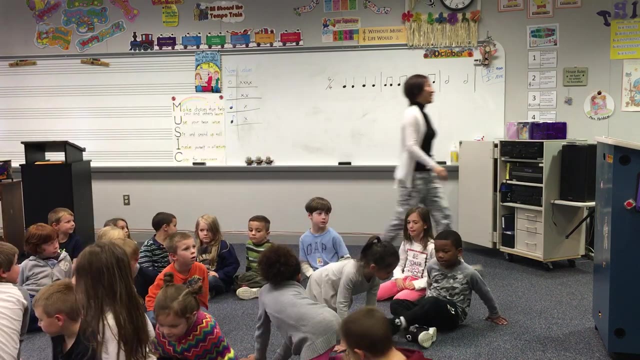 Can we do it like this, Of course, But let's move over here a little bit. Move to the left, Move to the left, Hurry, Hurry, Move, Move Up Over here. It's better that way. 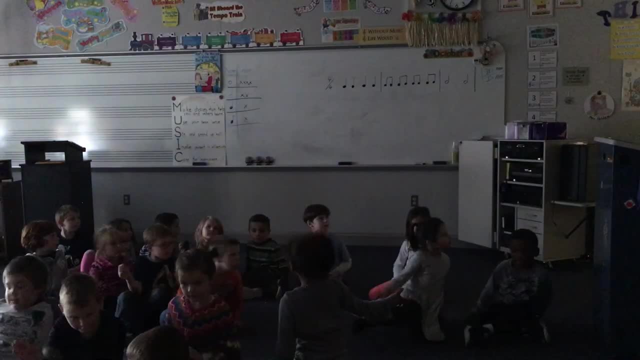 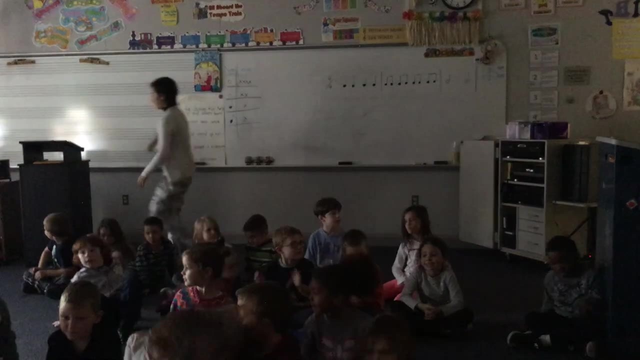 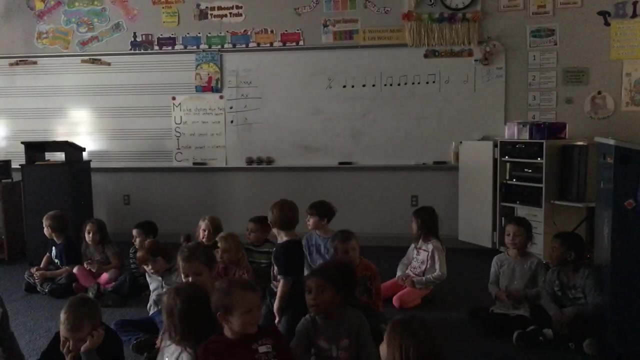 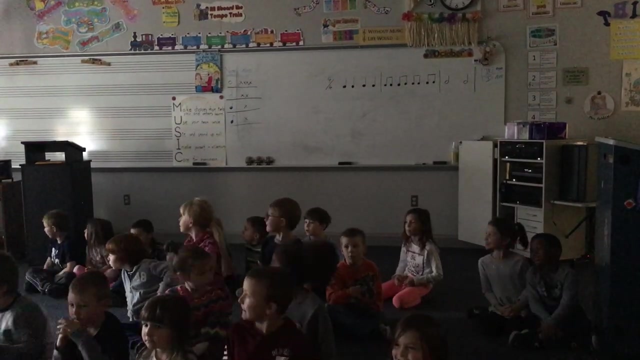 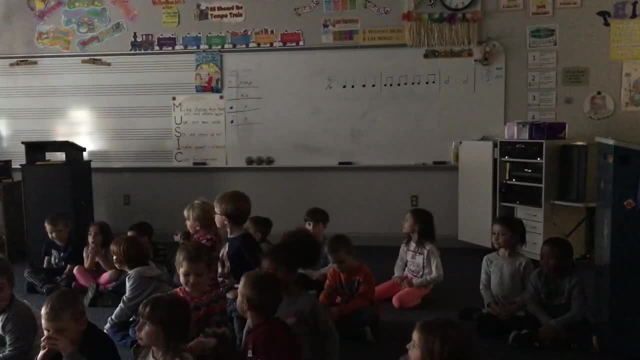 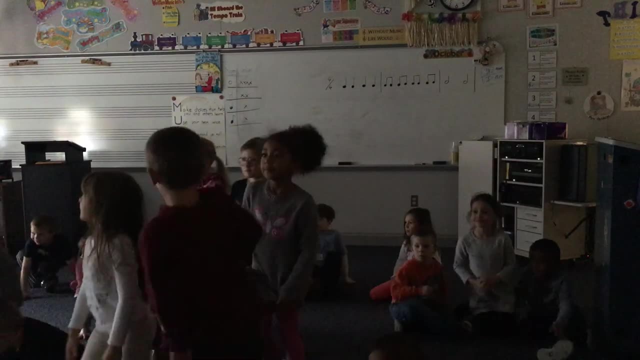 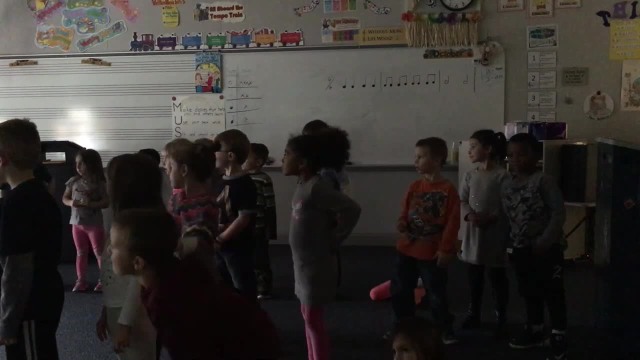 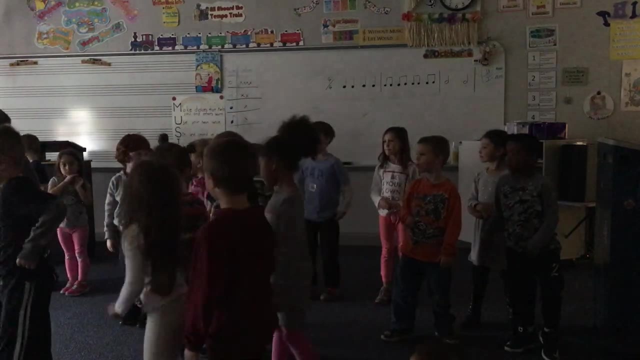 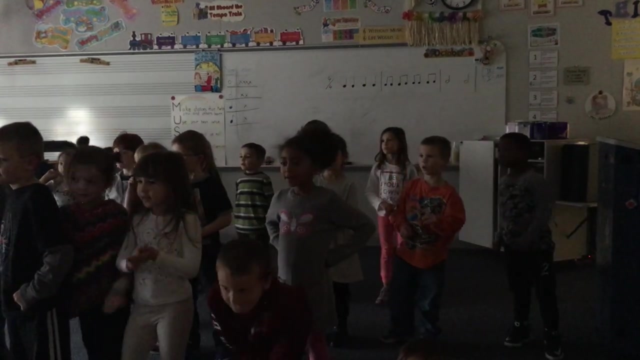 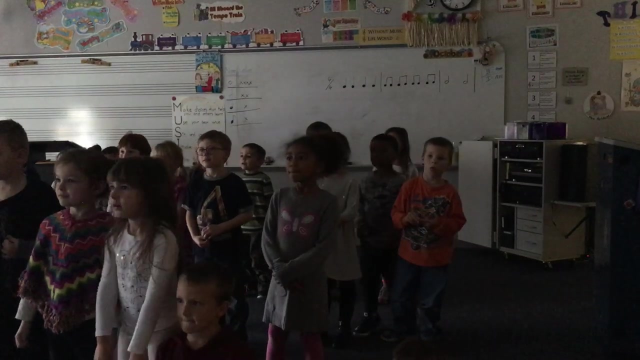 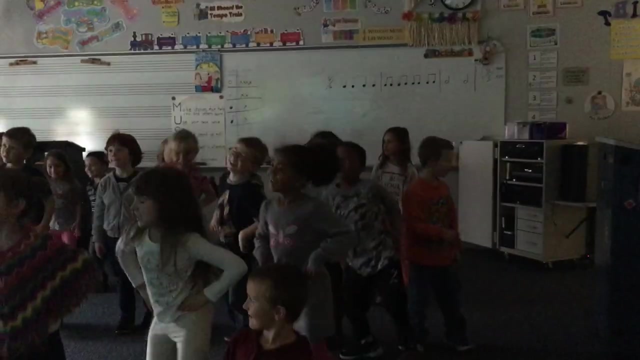 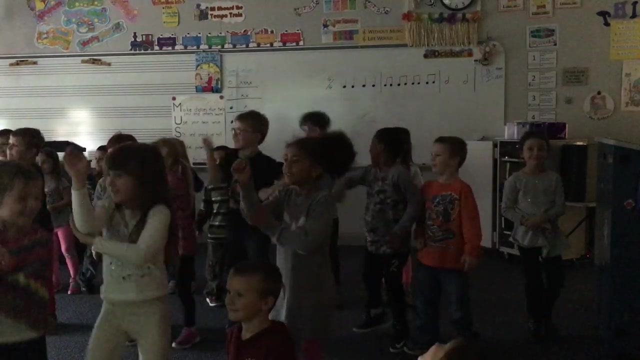 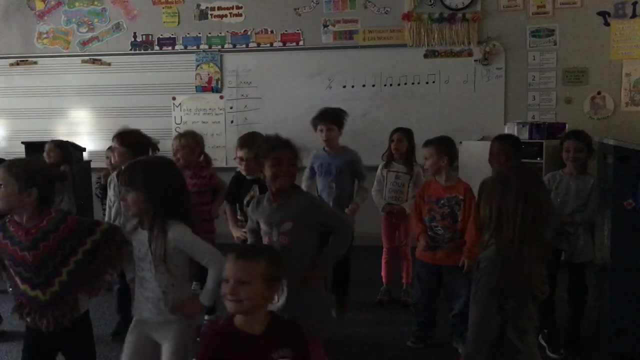 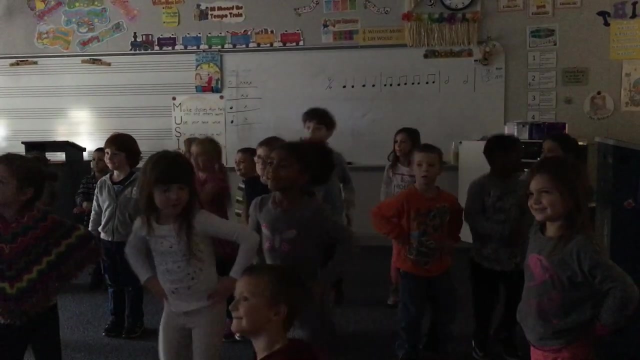 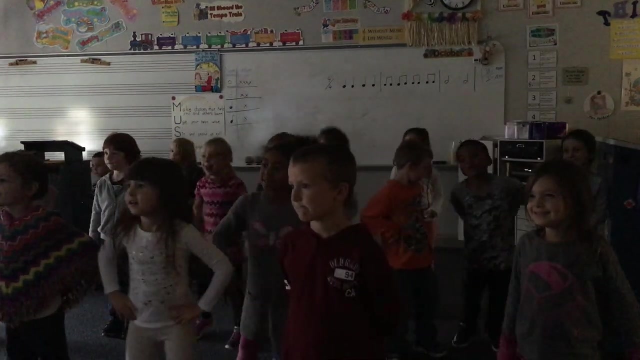 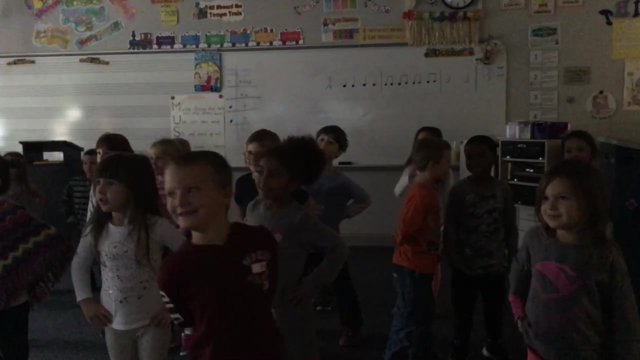 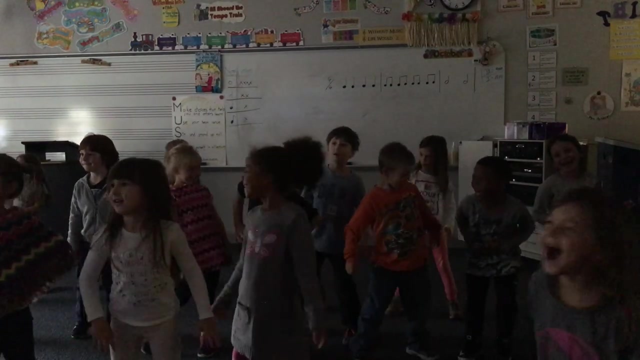 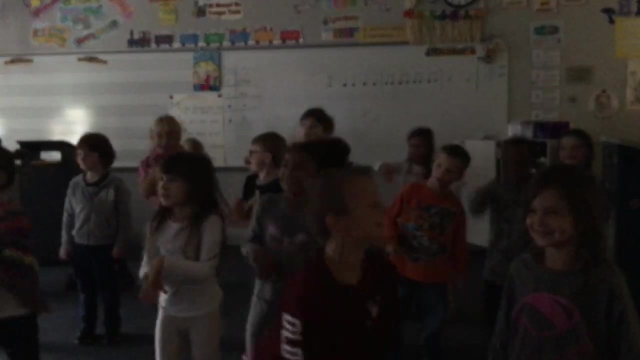 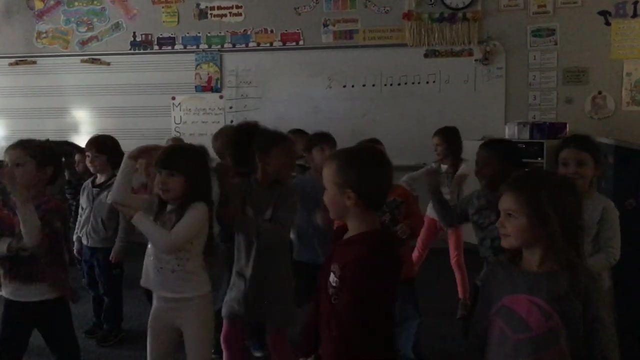 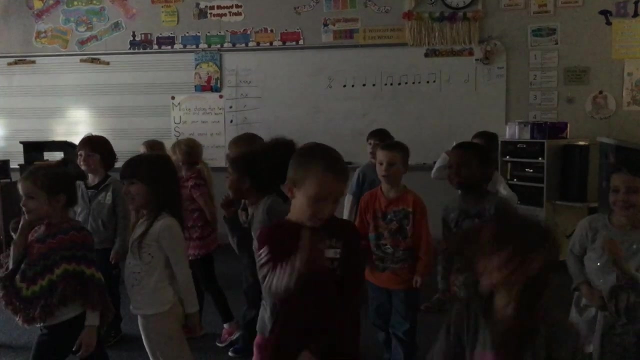 You dance to it, You guys Dance. You love dancing to it. It's going to go over there so we can watch it. It's going to go over there. What are you doing? We have to get down again. We have to get down again. 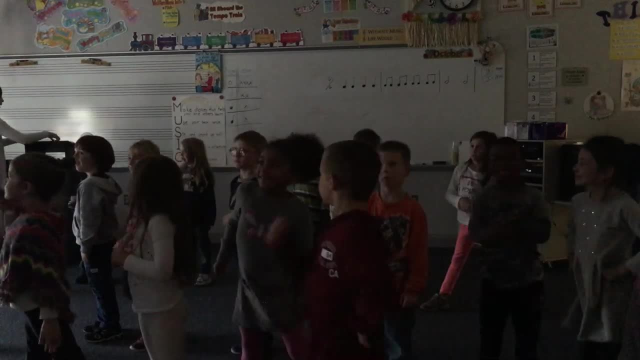 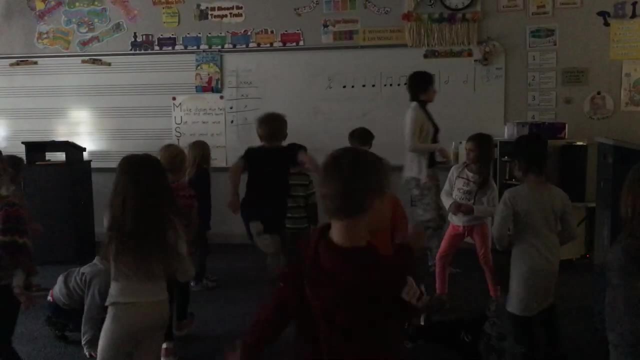 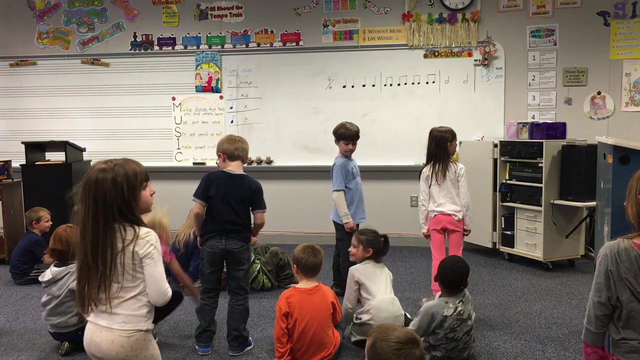 Shhh, Shhh. You've been having enough time to watch it again. Now back to your rows, Turn around. I'm dizzy, I'm dizzy. Shhh, I'm dizzy. I think we are standing up. I think we are standing up. 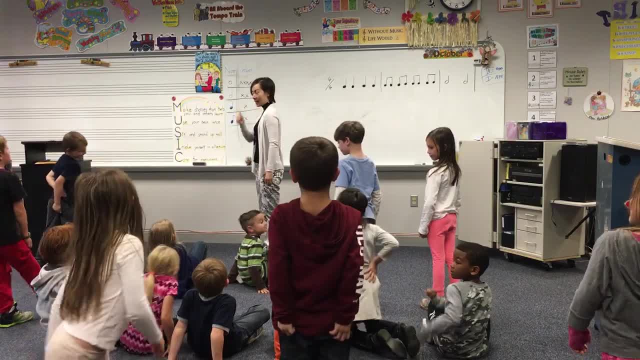 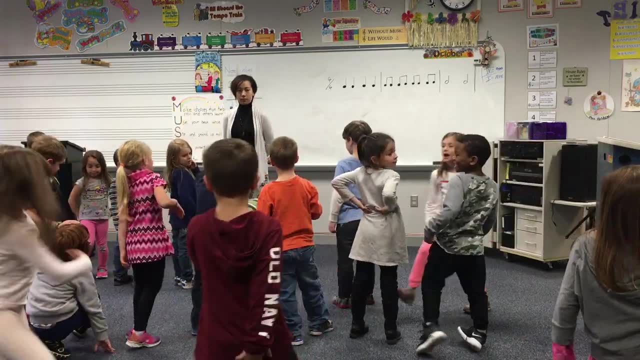 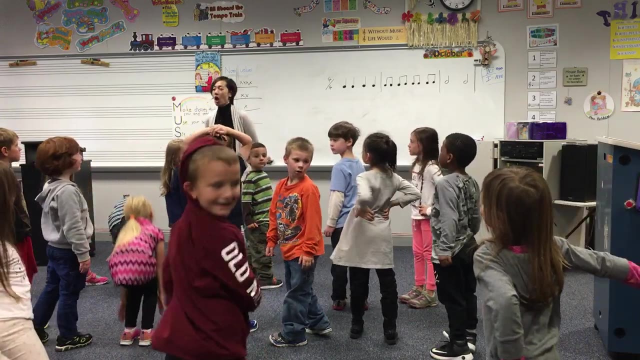 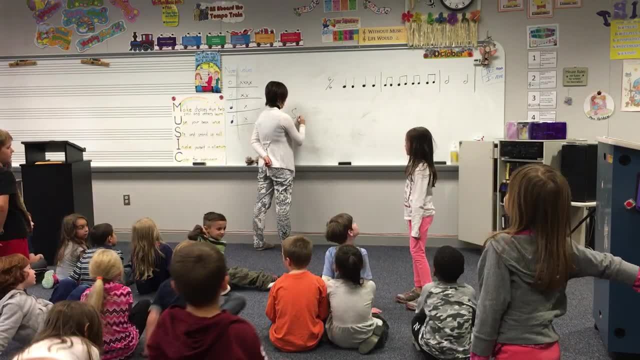 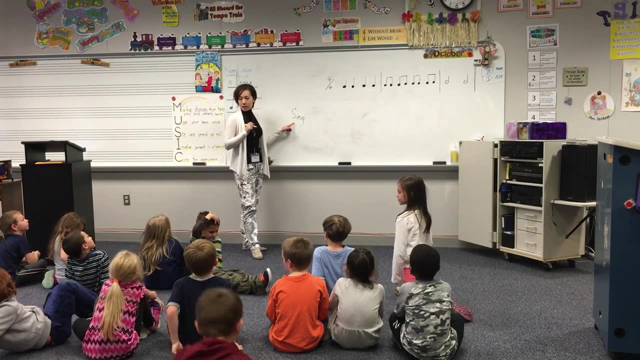 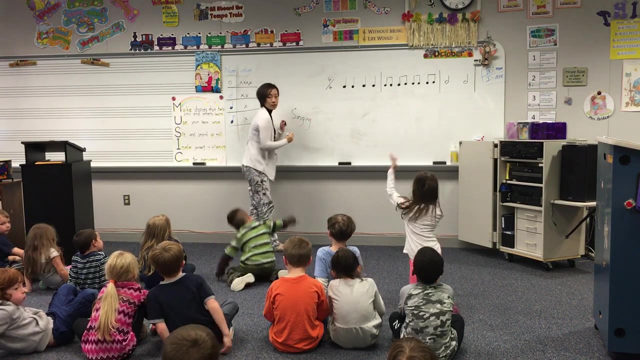 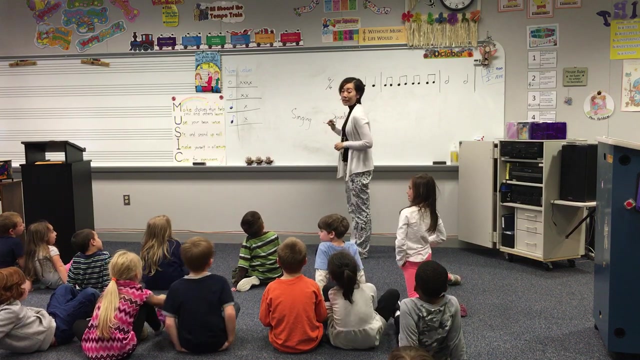 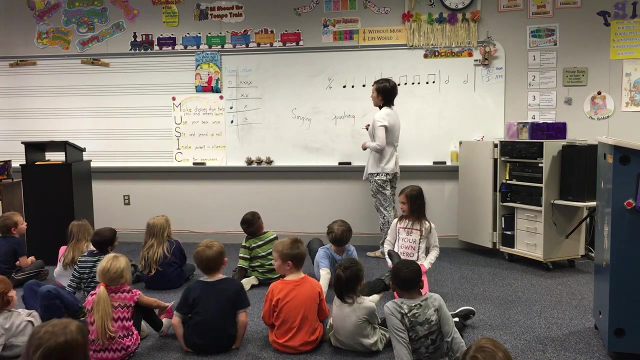 Shhh, Shhh, Shhh. Do you know the word? Do you know the word Sing? Do you know the word Sing, Singing, Singing? How about this? Speak, Speak, Speaking. How about this? 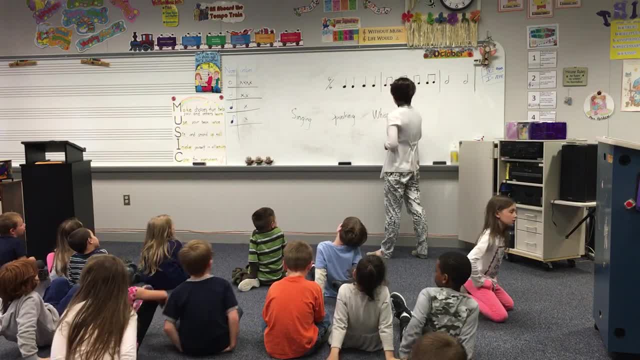 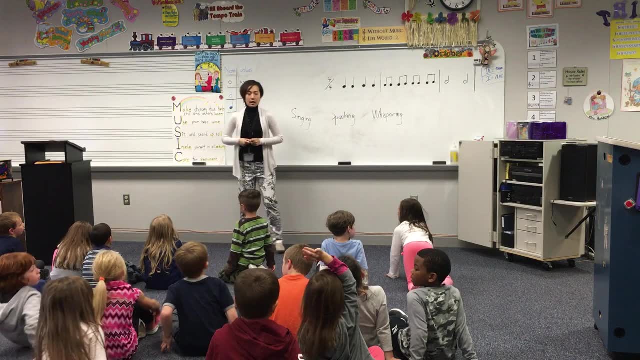 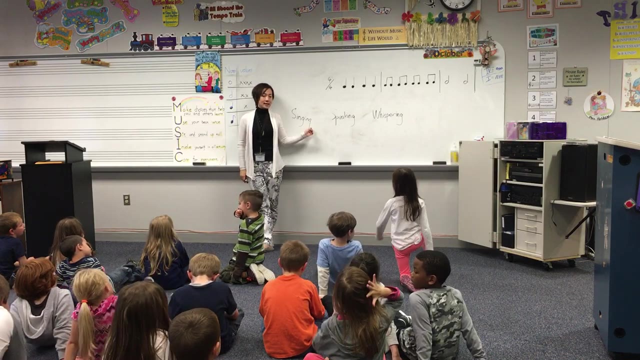 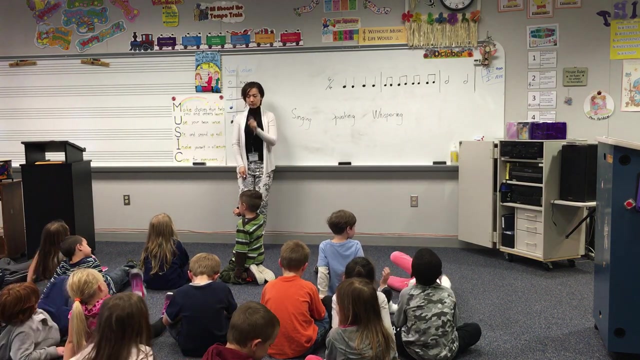 Whisper, Whisper, Whispering, Whispering. Now, we'll make some sounds. We'll make some sounds And tell me if I'm singing or speaking Whispering. Sit on the bottom, Listen and sound, Listen and sound, Listen and sound. 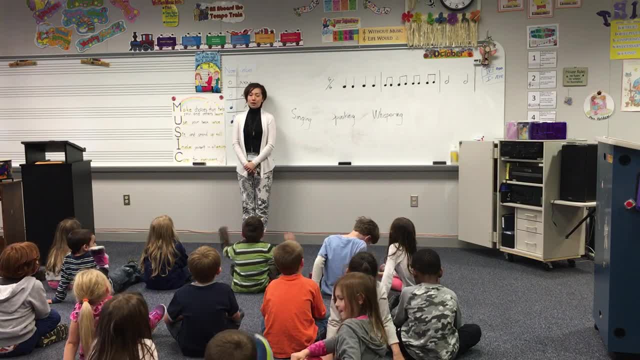 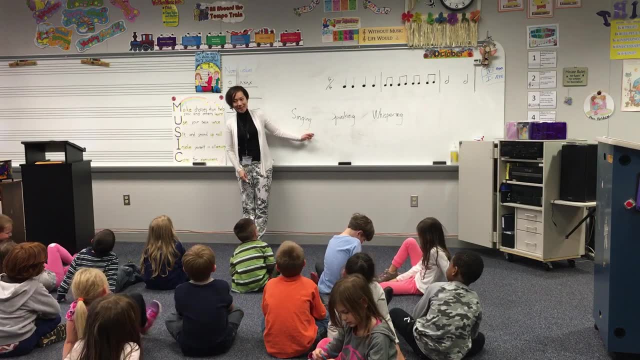 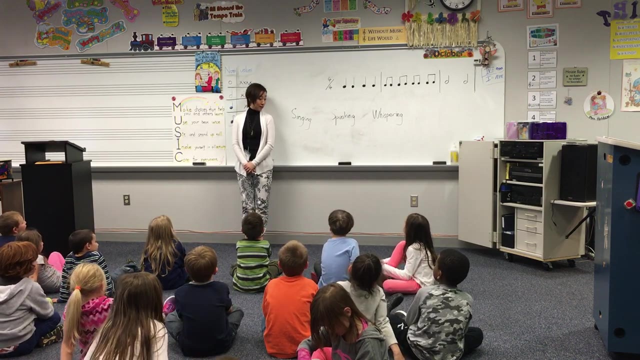 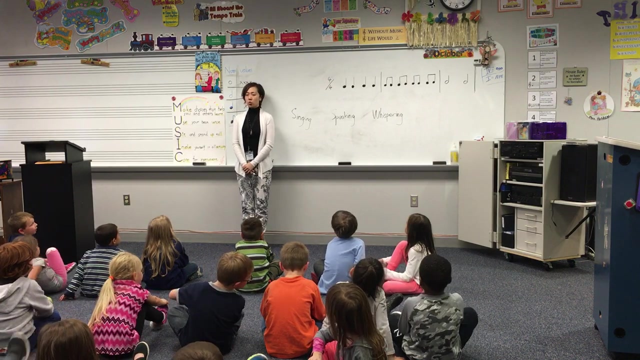 Whispering, Whispering, Whispering, Whispering, Whispering, Whispering, Whispering. Now tell me which one is. Do you have here or no? Are we good? Yes, Now tell me which one is: an opera singing, Oh. 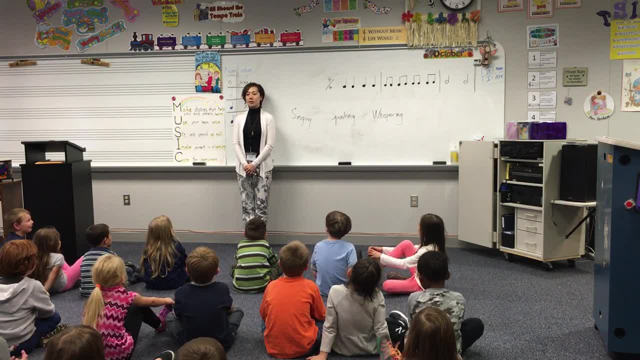 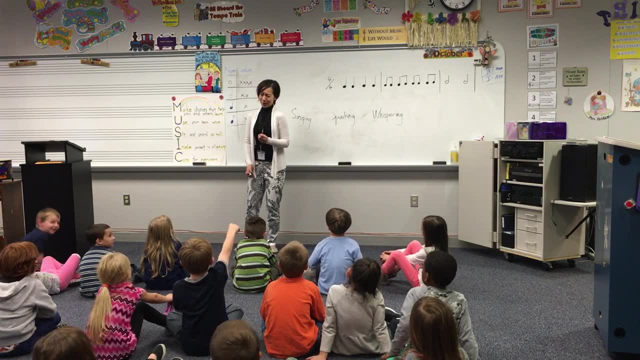 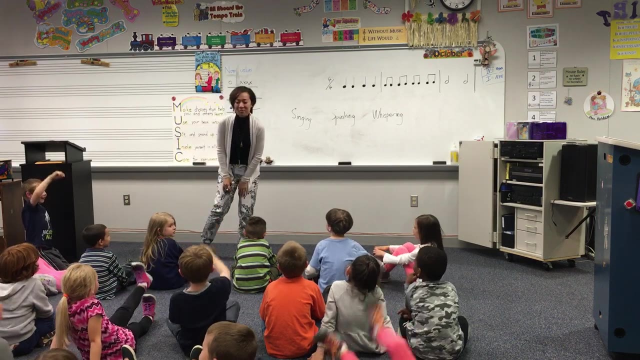 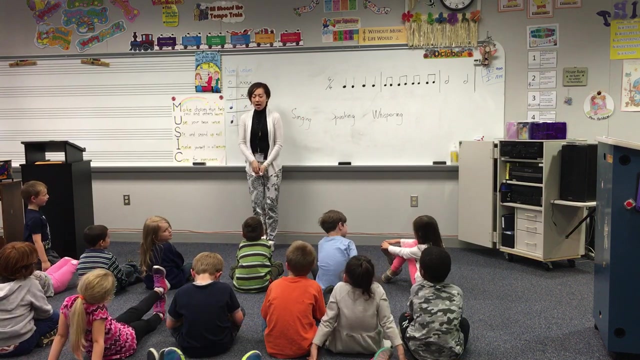 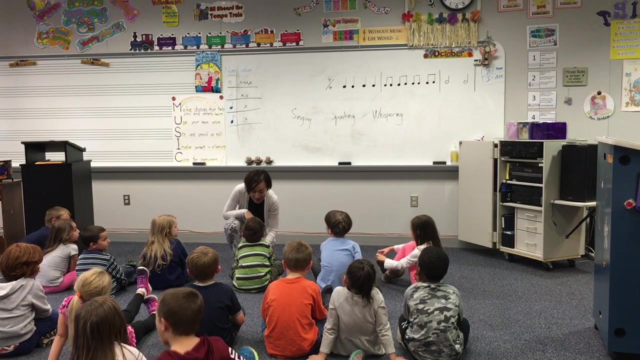 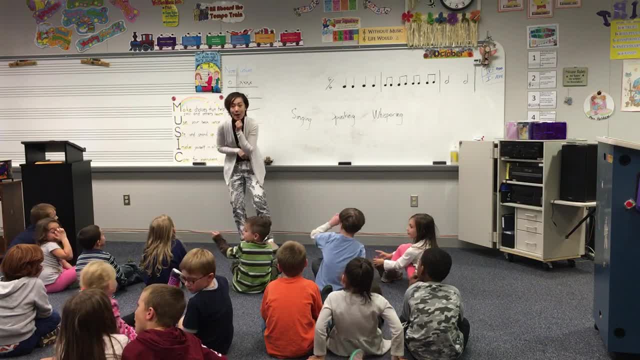 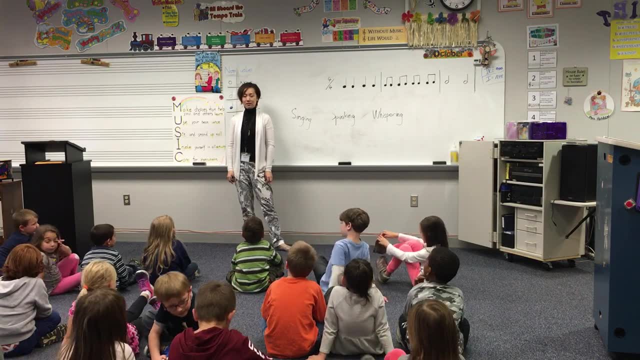 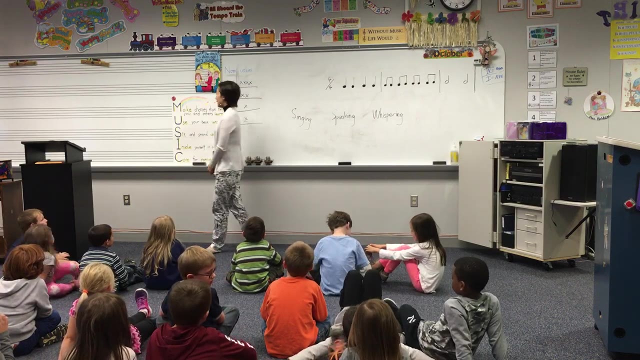 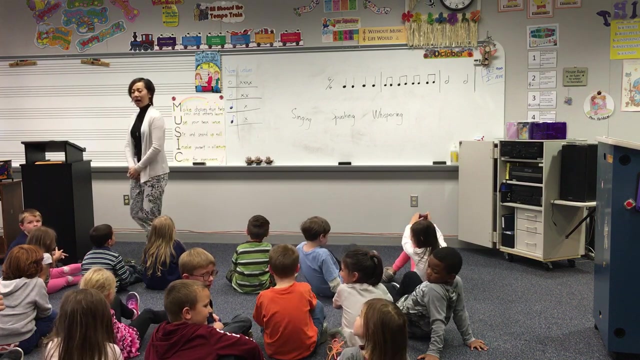 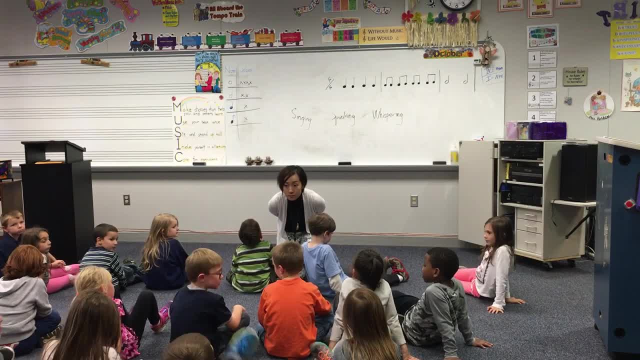 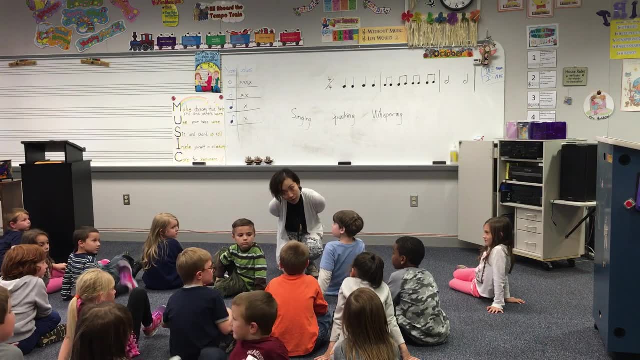 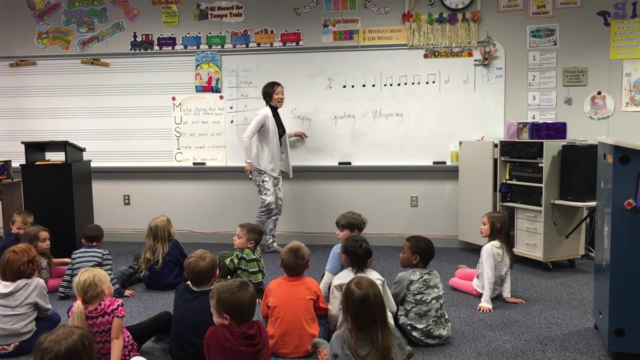 Spongebob in here. Spongebob in here. Two, three On your head. Oh my God, Oh my God, I'm traveling with you, Nice. Can you give me a hug? Can you give me a hug? Same voice. 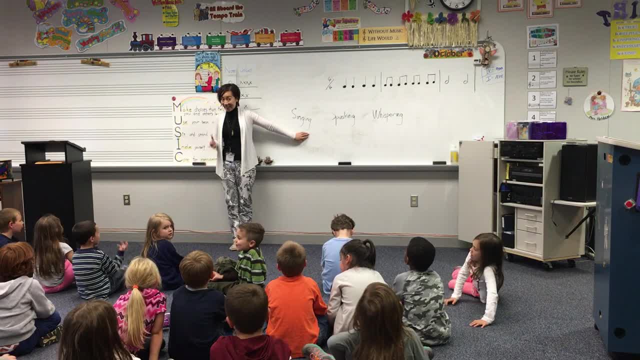 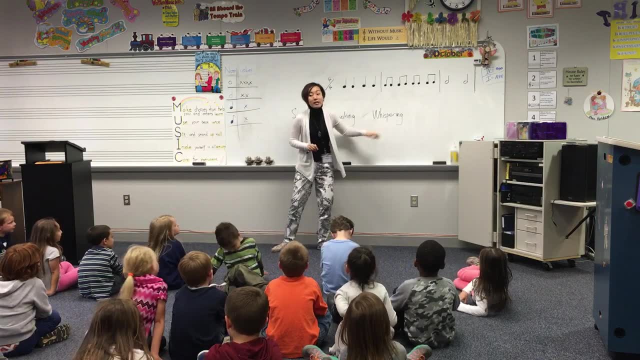 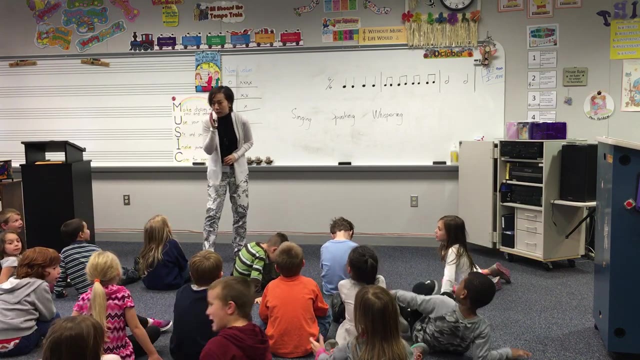 One, two, three, four sing. Oh my God, Very nice Shh. How about whispering? How about whispering? How about whispering? Who is great I like? Give me the whispering Good job. 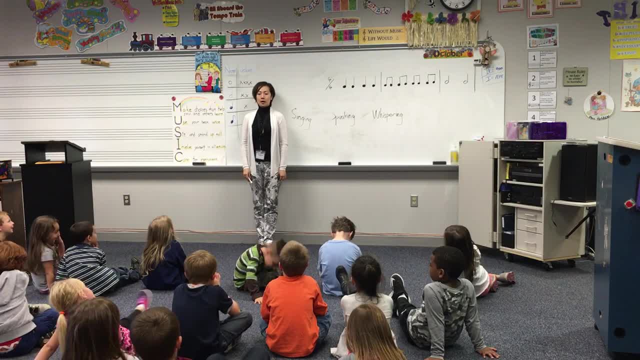 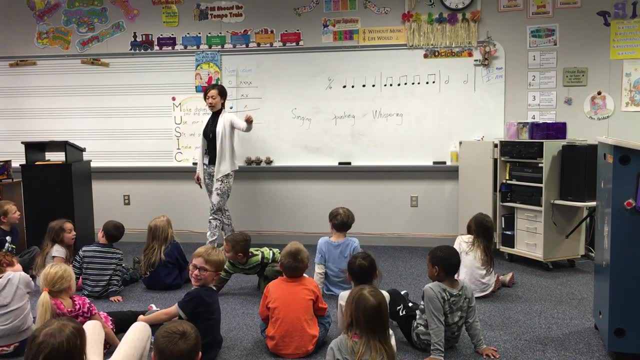 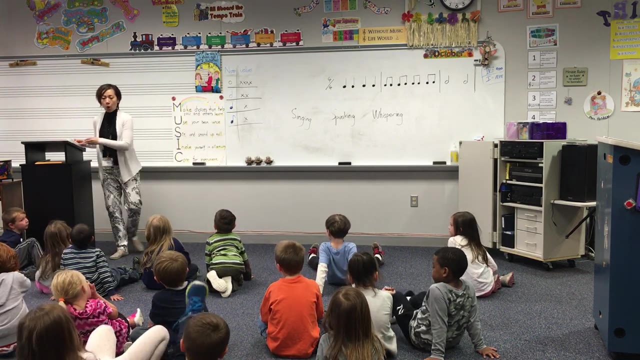 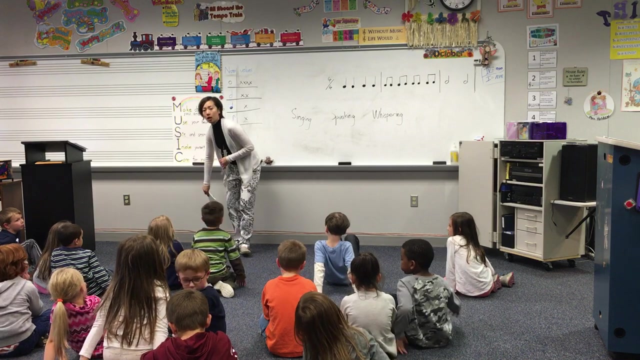 How about speaking Good job? Thank you, Shh. Good job, Good job, No, Okay Question: What is composure? What is composure? What is composure, Composure, What is composure? Where's my pen? 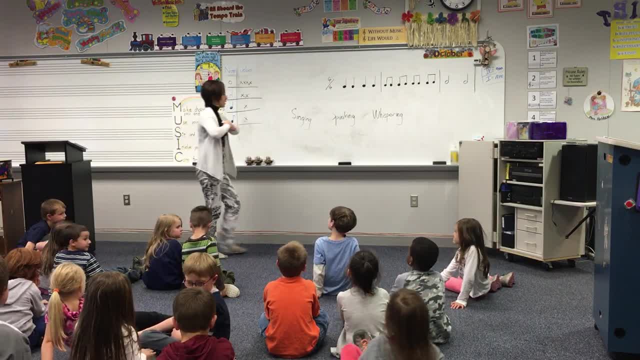 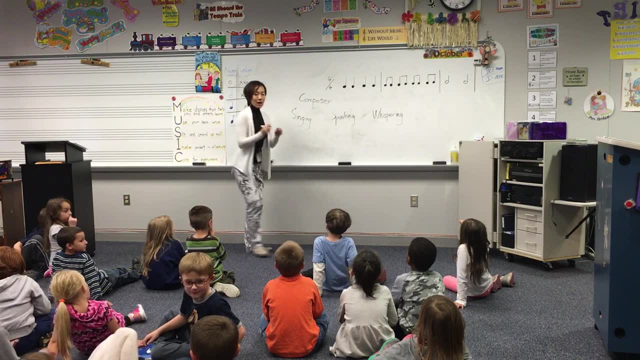 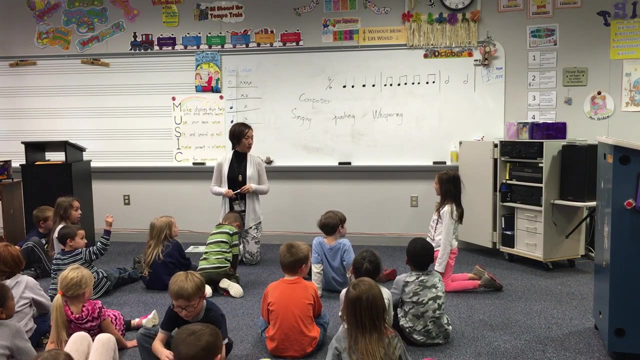 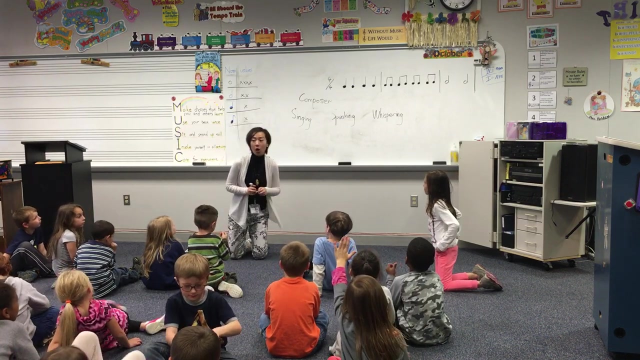 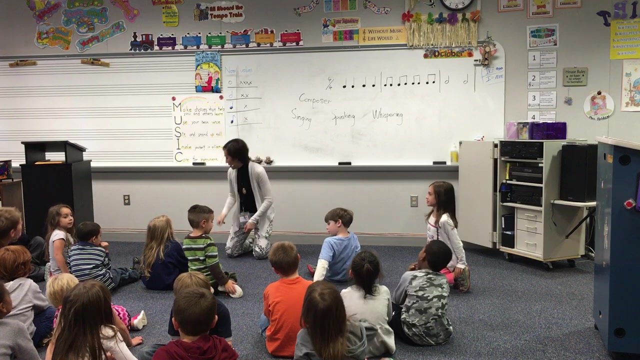 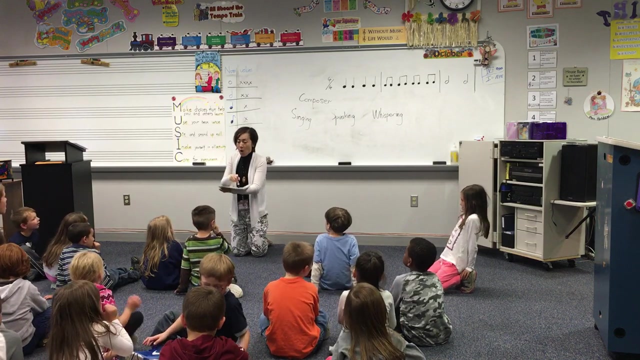 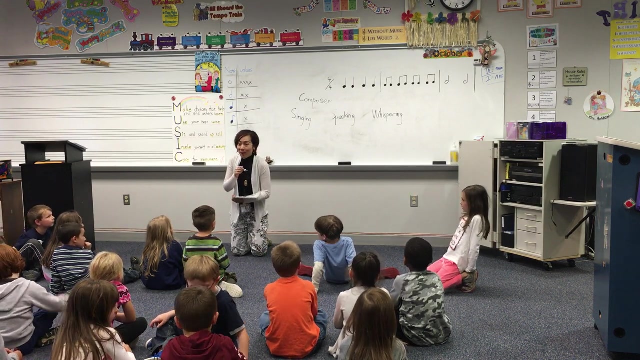 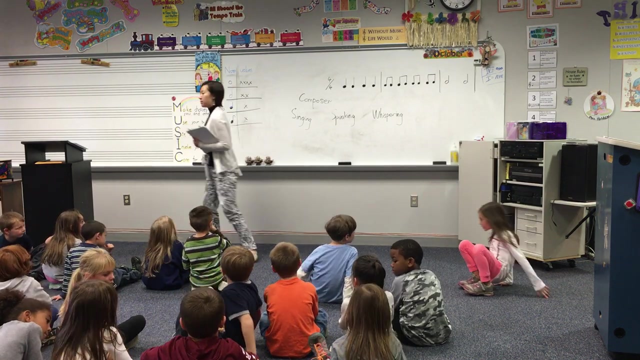 Compus, Compus, Compus, Compus, Compus. What is composure? Composer is the people. What am I doing Mixing? What am I doing Writing? Composer is the people who write the music. Composer is the people who. 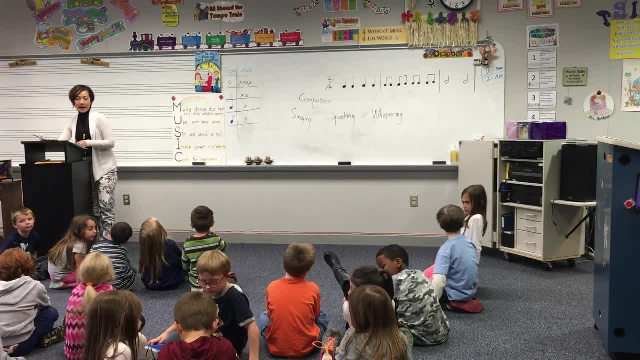 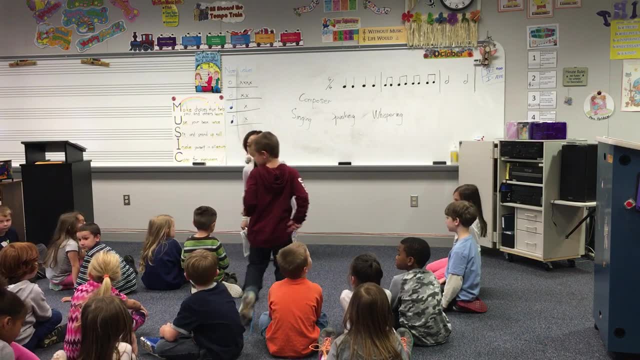 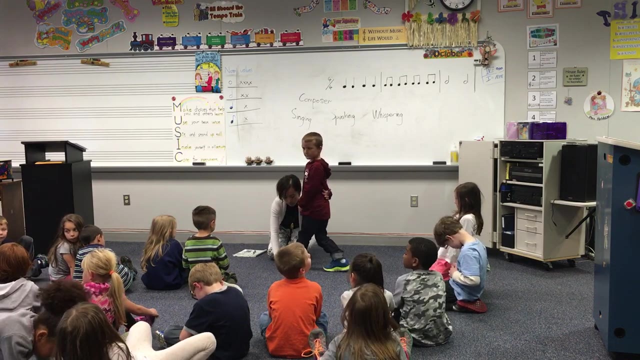 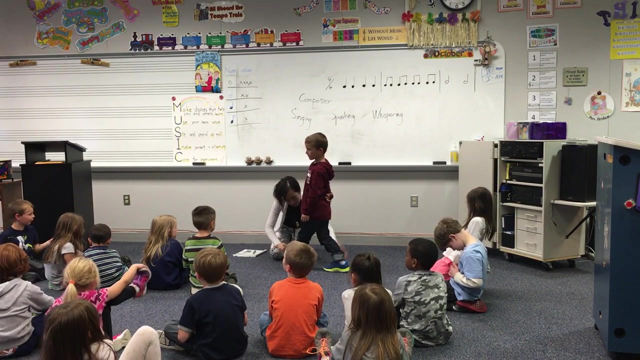 write the music: Hayden Hayden, come over here. What He said something? No, you don't say That he means it's a bad word. Oh no, They're called curse words. Oh, No, question, Logan, they call it curse words. 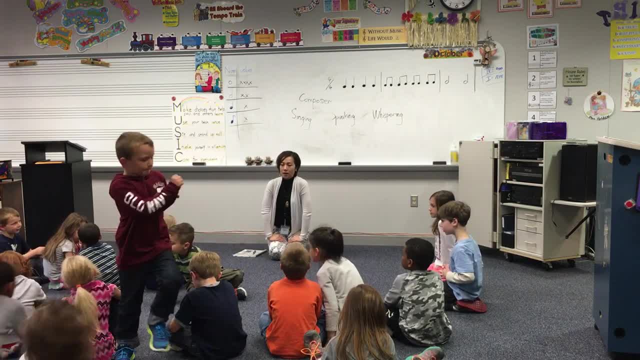 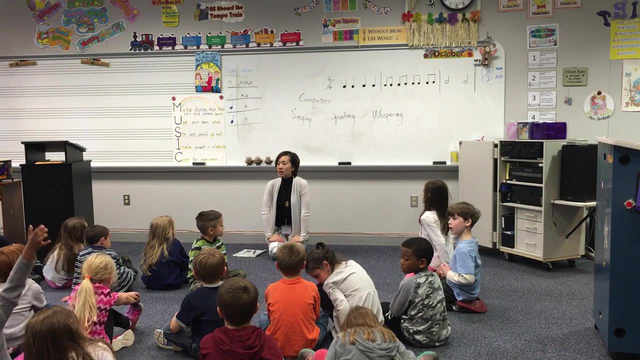 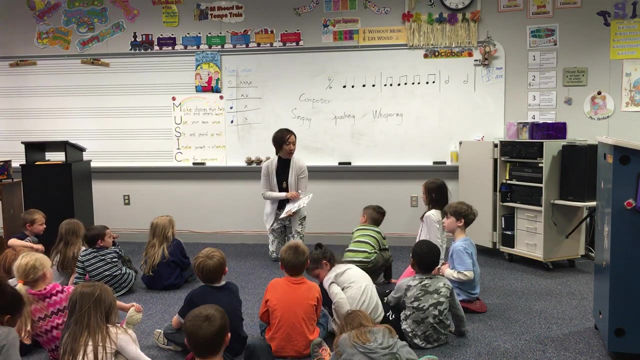 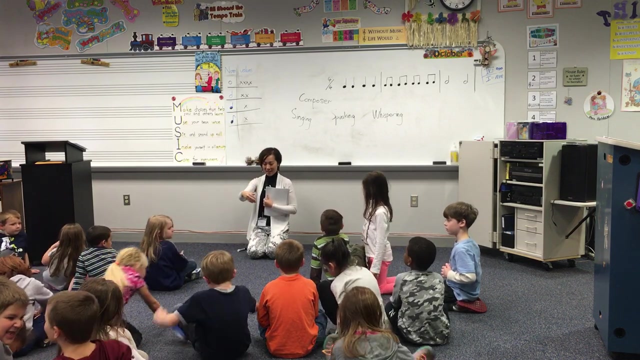 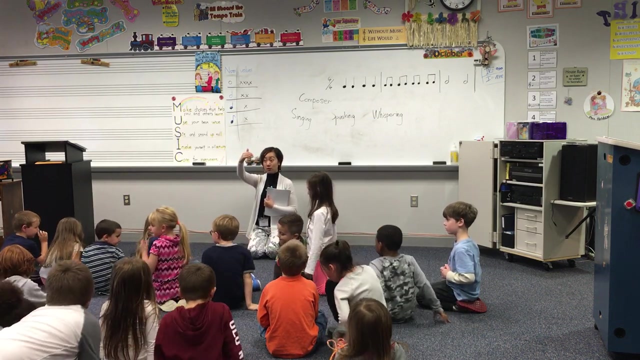 Good, okay, Question: What is a composure Turn around? What is a composure Music? Someone that writes music, Good job. Composer is the people who write music. First row here. Second row: move forward. Third row: move forward. 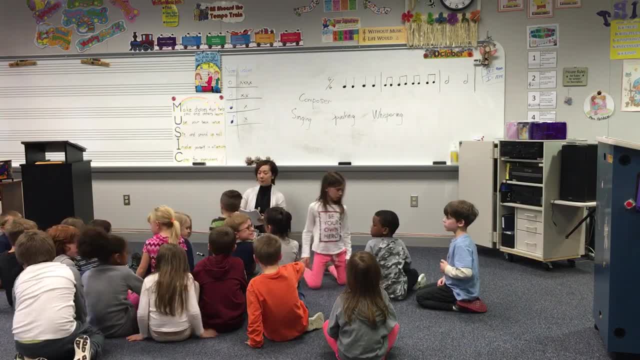 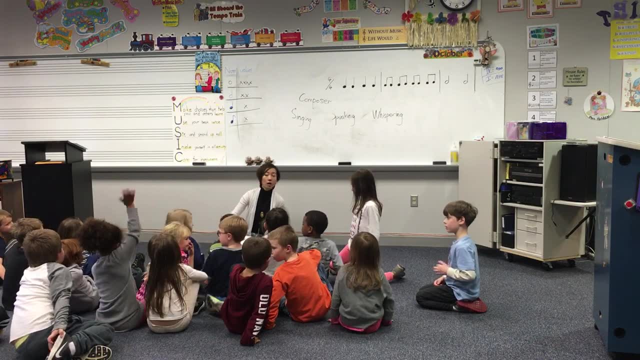 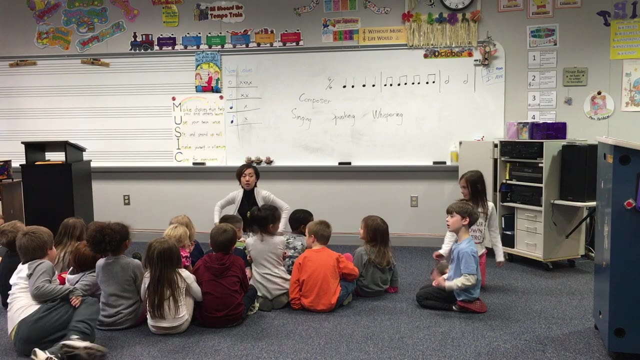 Sit on your bottom. Say it again: Sit on your bottom. Let's face that you can see me. Hey, Can you see me? Where are you? Where are you? Good, That's me Now sing, Sing after me. 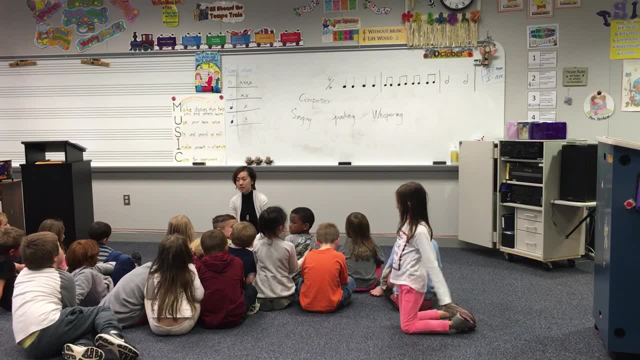 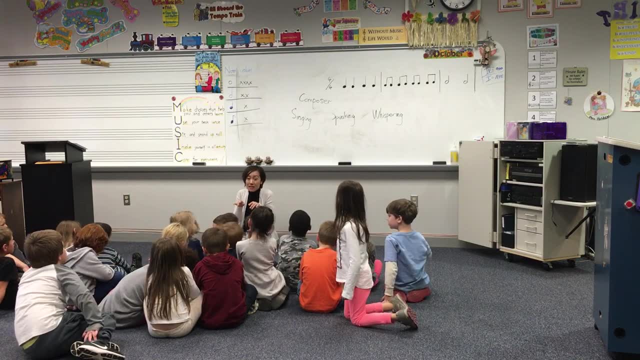 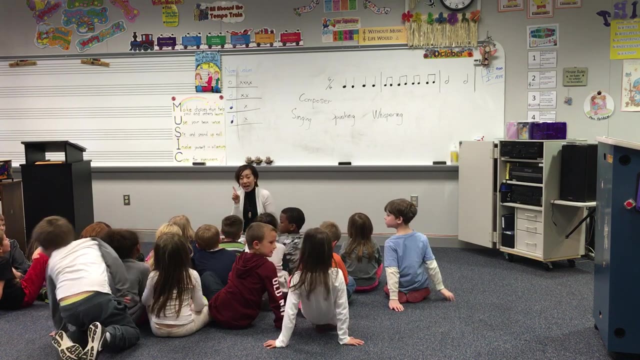 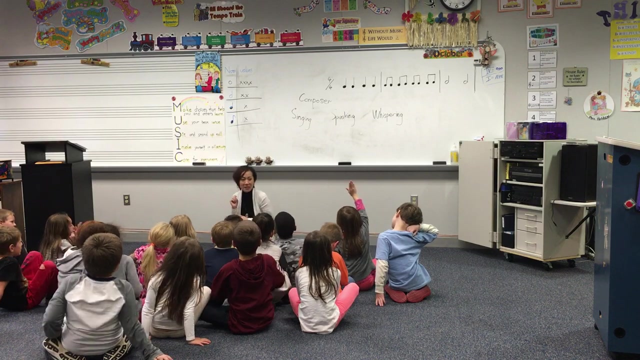 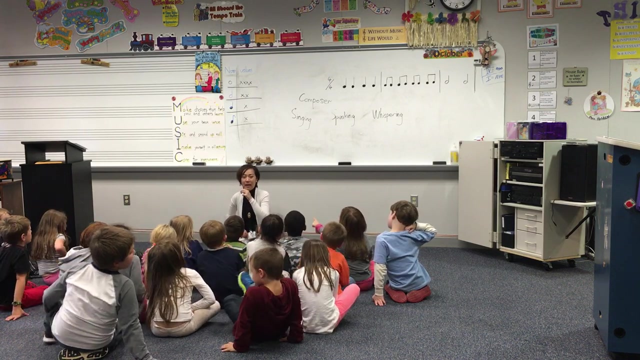 Sail, sail, sail free ships. Sail, sail, sail free ships. Slowly through the sea. Slowly through the sea. Three names: Ina, Penta, Santa Maria. Count them one, two, three. 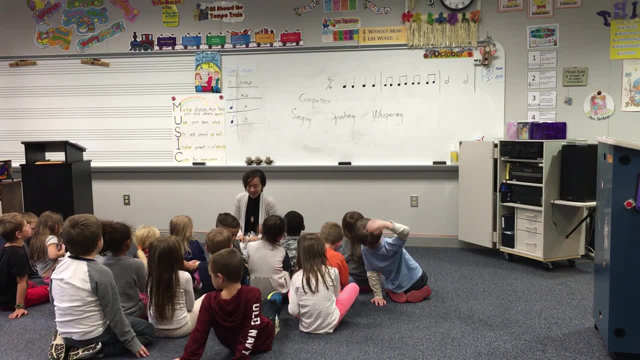 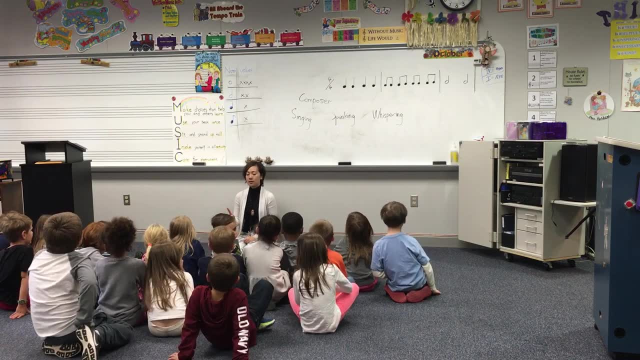 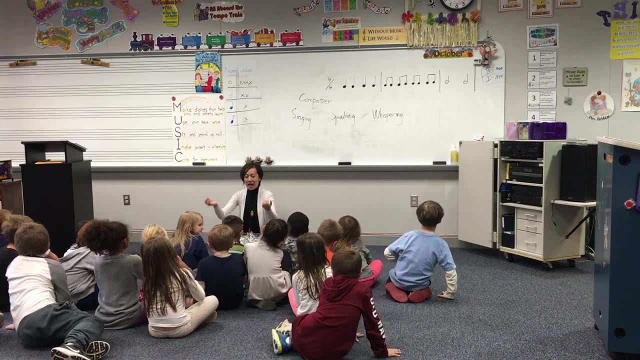 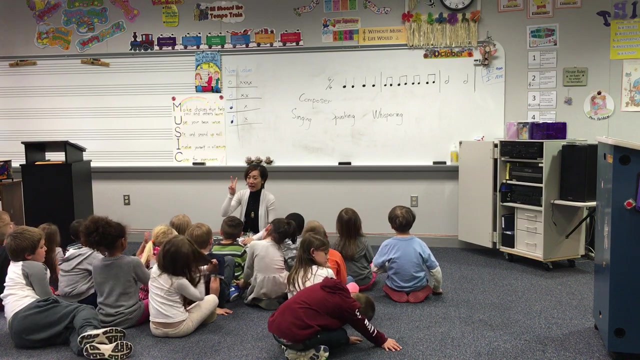 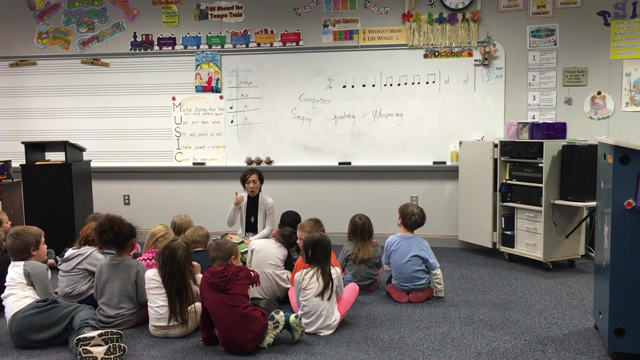 Count them one, two, three, Listen, Listen And one more time say it after me: Ssh, Sail, sail, sail three ships, sail, sail, sail three ships, slowly through the sea, slowly through the sea. Nina Penta, Santa Maria, Nina Penta, Santa Maria. count them one, two, three. count them one, two, three. 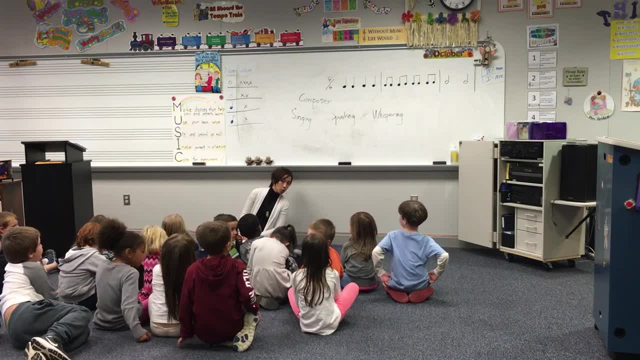 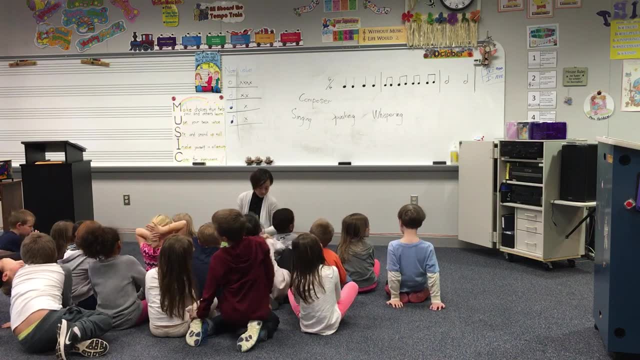 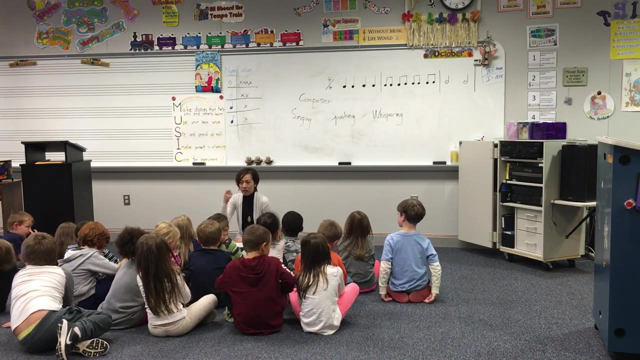 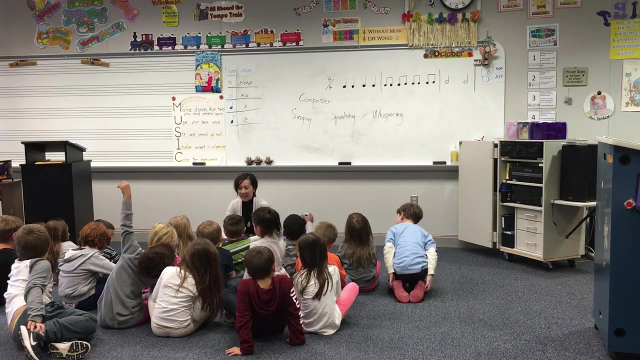 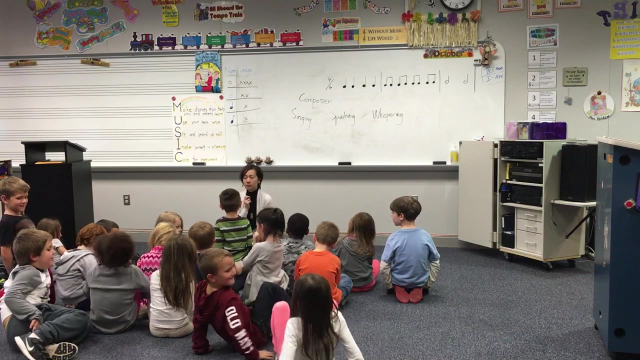 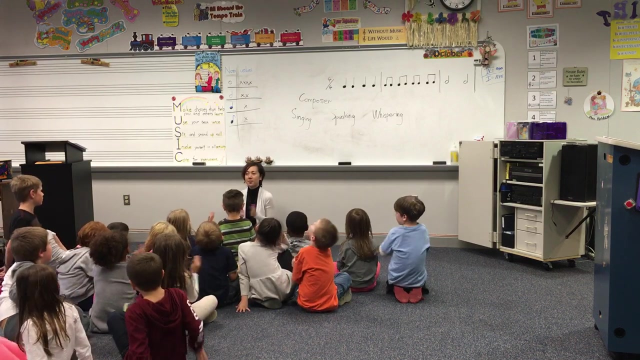 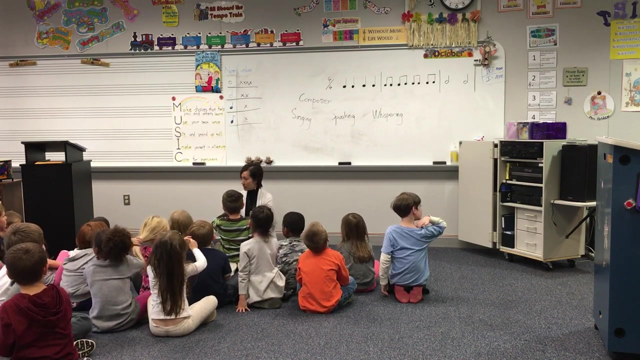 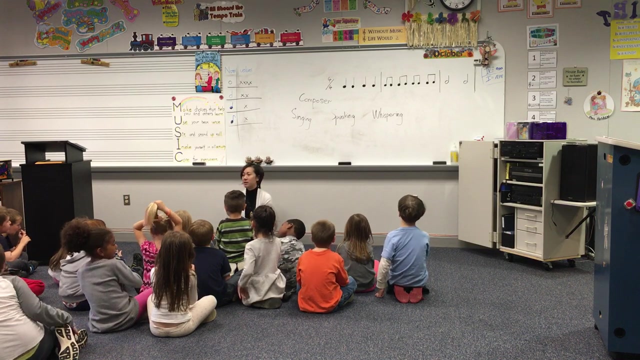 Let's sing some songs. Let's sing some Halloween songs On Halloween, you will laugh. Or let's sing Trick or Treat. Trick or Treat, Trick or Treat. It's all in the dick, It's all in the dick. One, two, three, four, Shh. Clap with me. No, What did you say? No, I said: clap with me. What did you say? Clap, Say nothing, Nothing. Clap with me, Right. Okay, Where is my third row? Where is my third row? 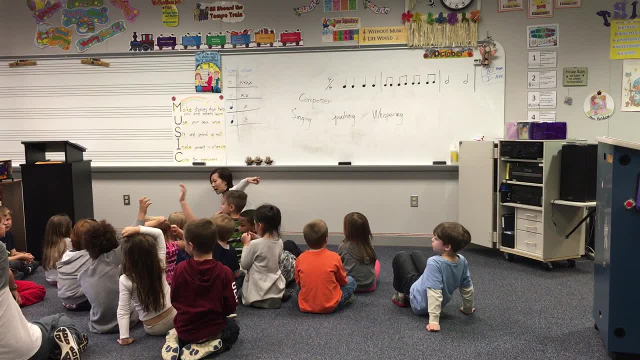 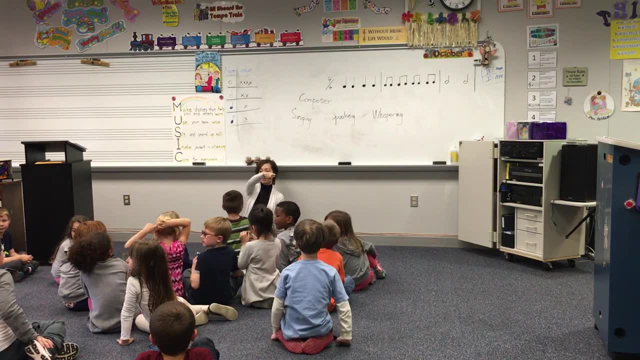 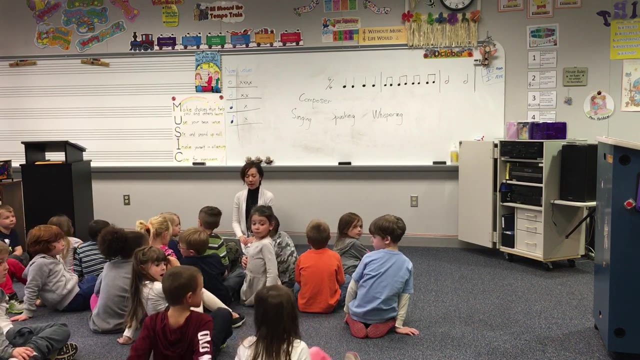 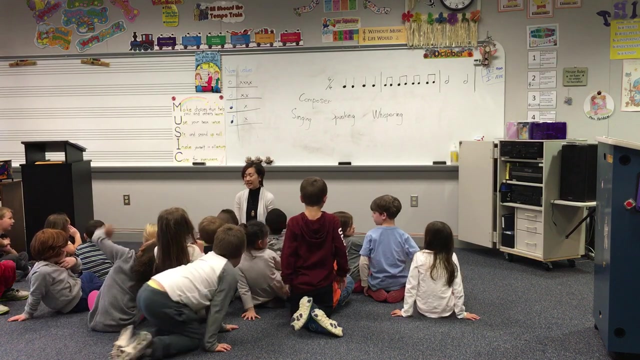 Someone Back to your spot. Bless you, Bless you. No, No, Only the girl Back to your spot. We are good. Now listen, Halloween is coming. I like it the most. Halloween is coming, I like it the most. I love me a company. 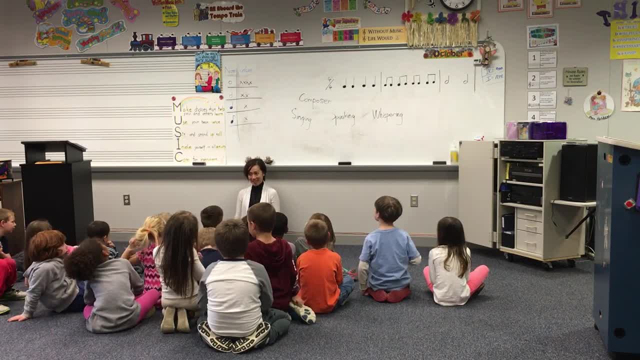 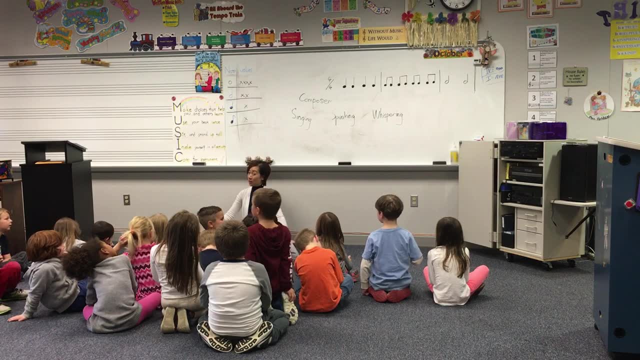 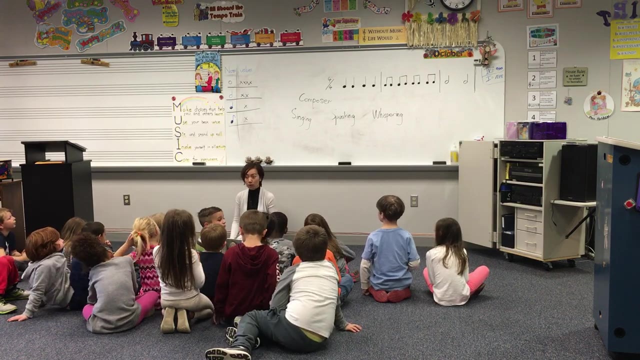 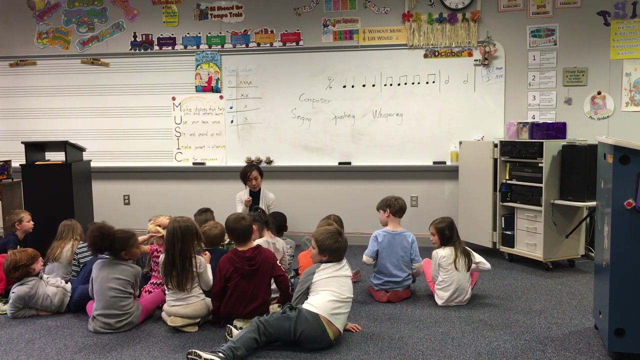 You can be a ghost. You can be a ghost. Okay, When we get undressed up, we will sing. When we get undressed up, we will sing Boom Boom Now, Anthony, Oh, oh oh. One, two, three. I say B, Turn your body. One, two, three Now. boom, boom, boom. Sing with me, Anthony. 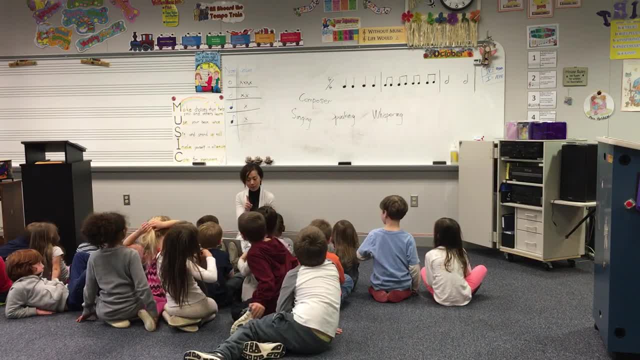 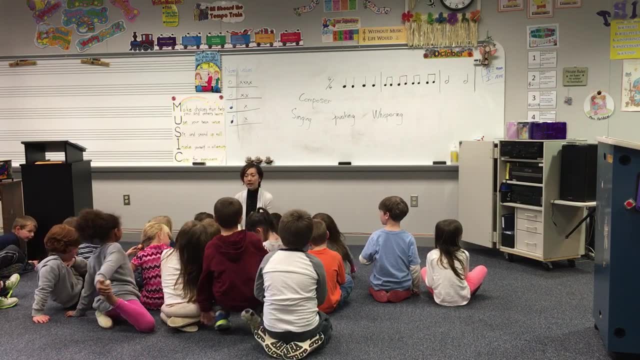 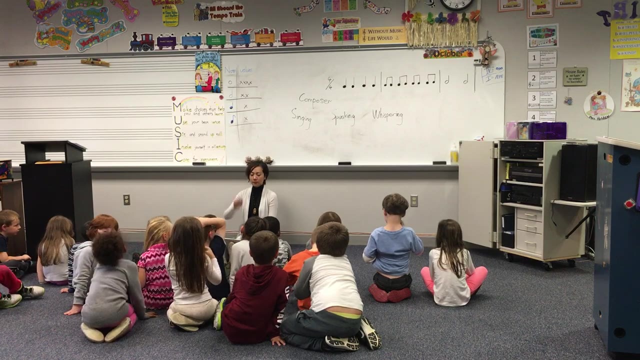 Bell. Thank you, I heard the bell. Let's finish this song. It's trick or treat today. It's trick or treat today One more time. Now listen to me When the wind is coming. I like it the most. 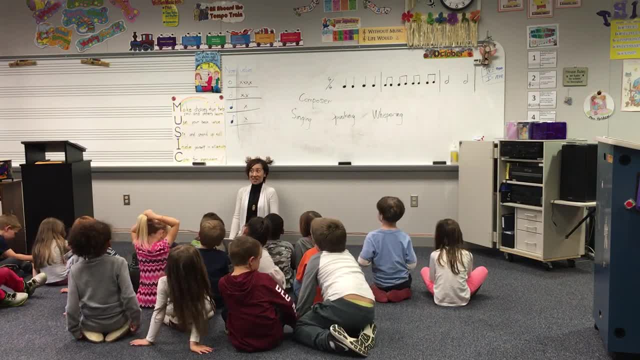 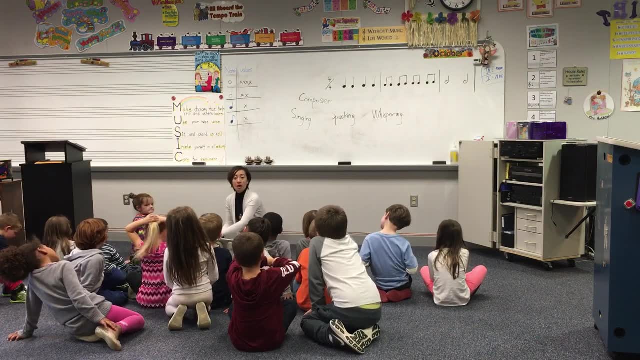 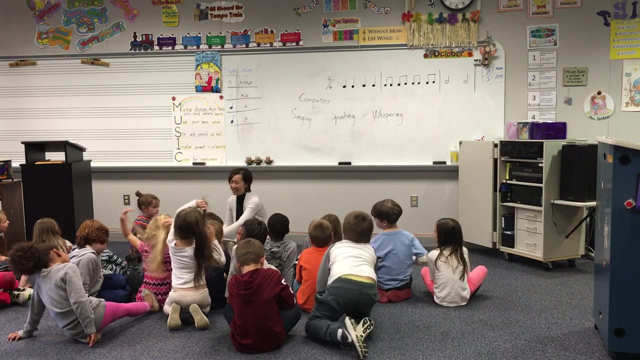 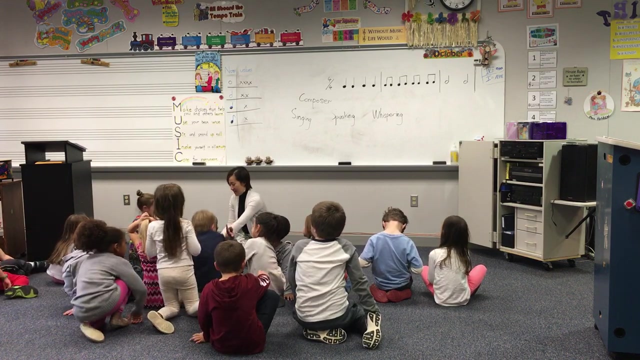 I'll be the dumpling. you can be the ghost. When we get dressed up, we will see. Woo Woo, It's trick or treat today. Boys over here, Face it, Face it. Take your book And don't forget the paper. 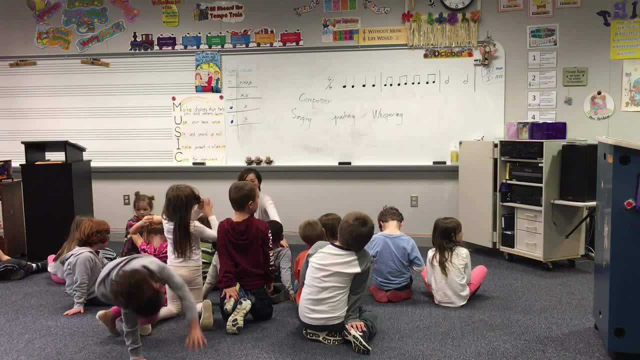 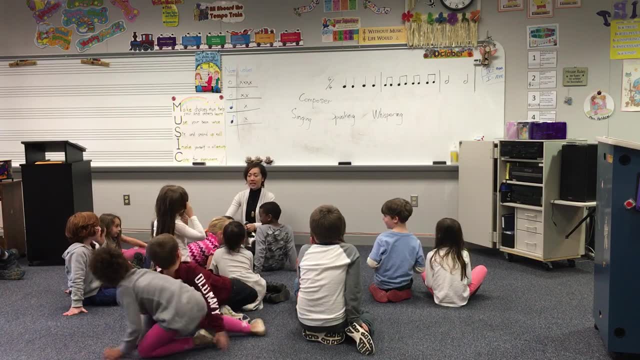 I can wear it. I can wear it. I can wear it. Come on, boy, I got sauce. Now let's see which row is sitting on top. Why not? Oh no, That's it. That's it, Yeah.